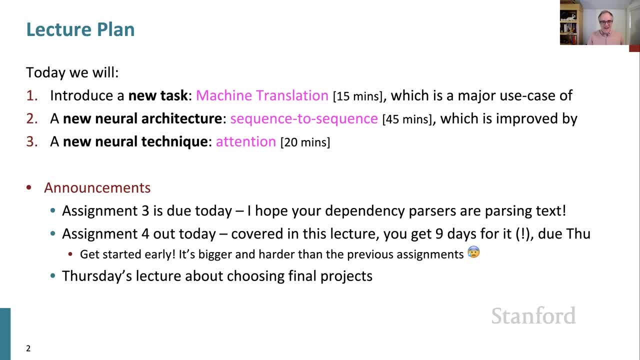 and so that's what I'll talk about in the final part of the class. Just checking everyone's keeping up with what's happening. So, first of all, assignment three is due today, so hopefully you've all gotten your assignments ready, So let's get started. 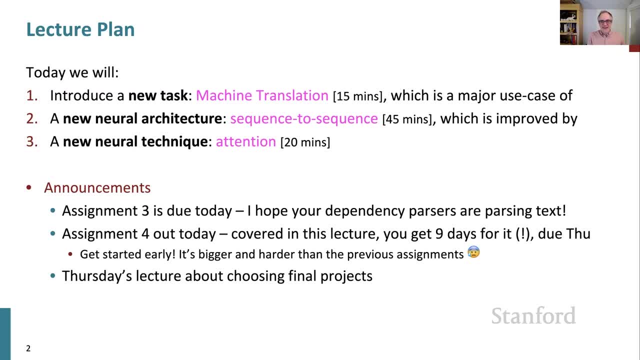 Assignment four is out today and really today's lecture is the primary content for what you'll be using for building your assignment four systems Switching it up for a little. for assignment four, we give you a mighty two extra days, so you get nine days for it and it's due on Thursday. On the other hand- do please be aware- 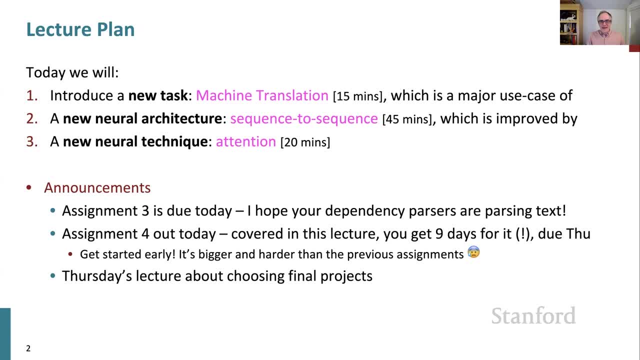 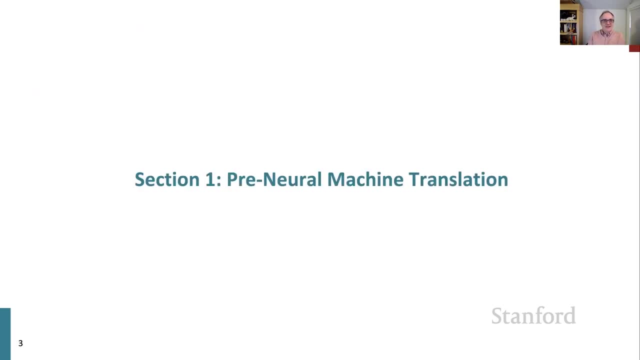 that assignment four is bigger and harder than the previous assignments, so do make sure you get started on it early. And then, as I mentioned, Thursday I'll turn to final projects. Okay, so let's get straight into this with machine translation. So, very quickly, I wanted to tell you 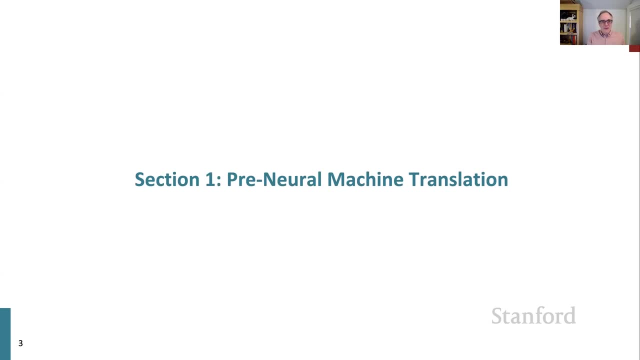 a little bit about. you know where we were and what we did Before we get to neural machine translation, and so let's do the pre-history of machine translation. So machine translation is the task of translating a sentence x from one language, which is called the. 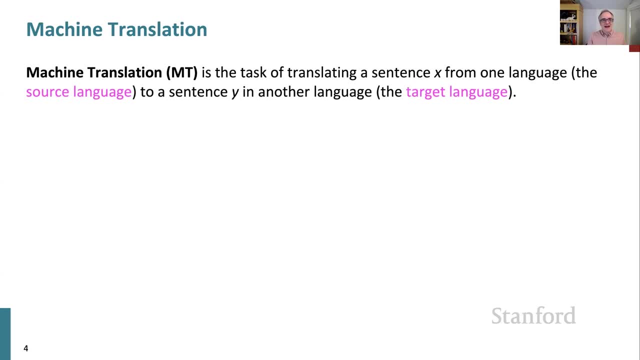 source language to another language, the target language- forming a sentence y. So we start off with a source language sentence x, and then we translate it and we get our kind of basic, basic generalization. So I'll show you here a little bit about the translation. 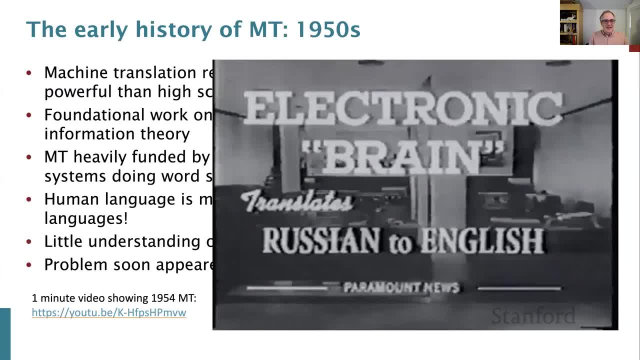 Man is born free, but everywhere he is in chains. Okay, so there's our machine translation. Okay, so in the early 1950s there started to be work on machine translation, And so it's actually a thing about computer science. If you find things that have machine and the name, most of them are old. 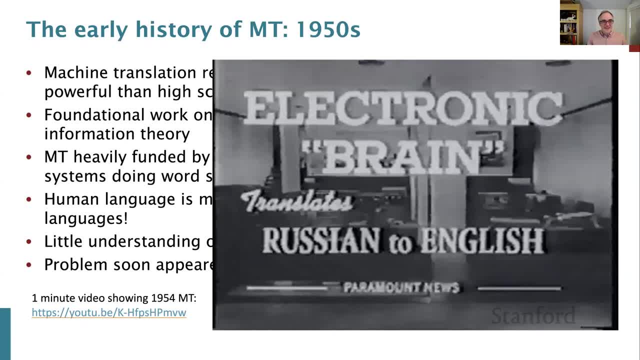 things So, and this really kind of came about in the US context, in the context of the cold war. So there was this desire to keep tabs on what the Russians were doing And people had the idea that because some of the earliest computers had been so successful at doing code breaking during the Second World War, 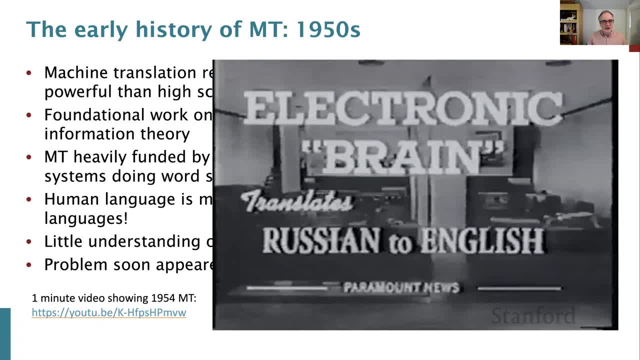 that maybe we could set early computers to work during the Cold War to do translation, And hopefully this will play and you'll be able to hear it. Here's a little video clip showing some of the earliest work in machine translation from 1954.. 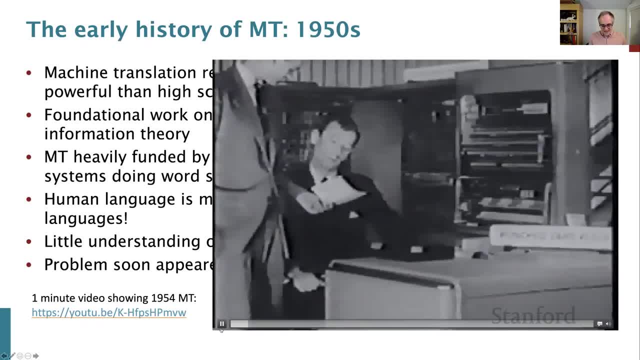 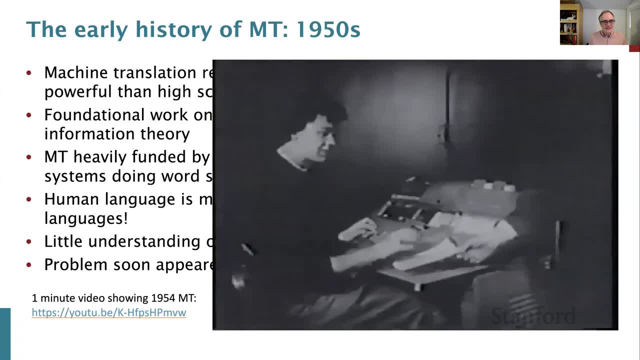 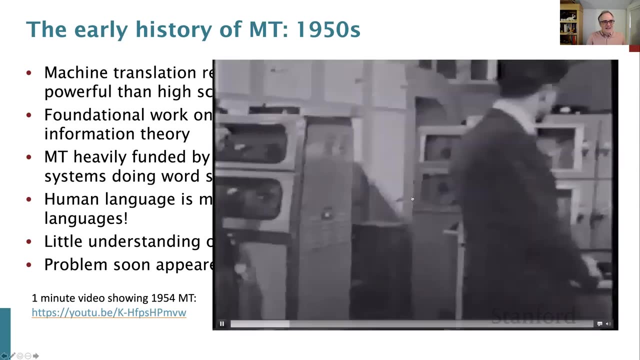 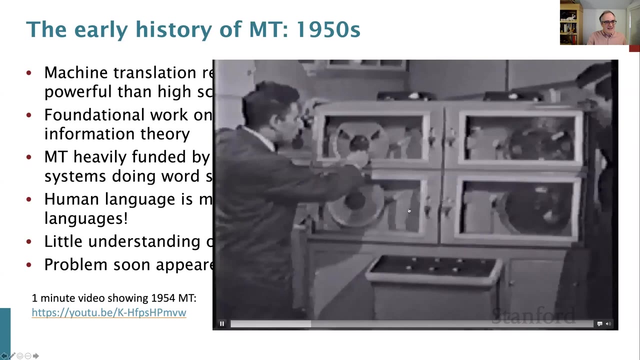 They hadn't reckoned with ambiguity when they set out to use computers to translate languages. A $500,000 super calculator, most versatile electronic brain known, translates Russian into English Instead of mathematics, One of the first non-numerical applications of computers. it was hyped as the solution to the Cold War obsession of keeping tabs on what the Russians were doing. 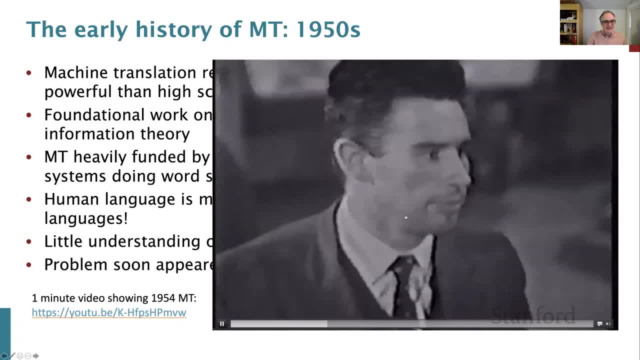 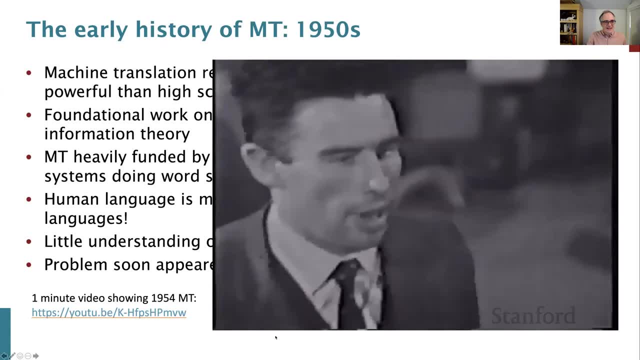 Claims were made that the computer would replace most human translators. At present, of course, you're just in the experimental stage. When you go in for full-scale production, what will the capacity be? We should be able to do with a modern commercial computer, about one to two million words an hour. 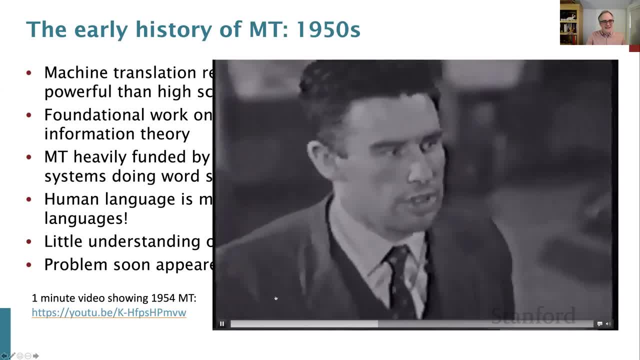 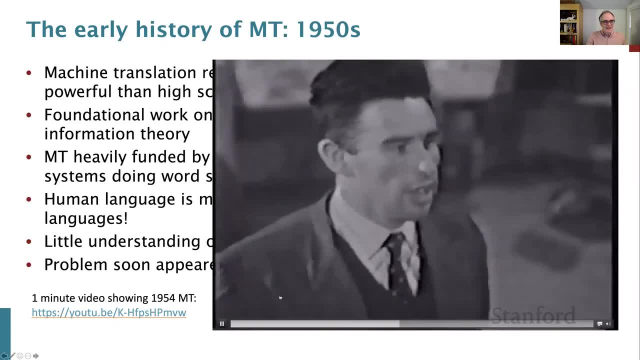 And this will be quite, quite an adequate speed to cope with the whole output of the Soviet Union in just a few hours computer time a week. When do you hope to be able to achieve this speed? If our experiments go well, then perhaps within five years or so. 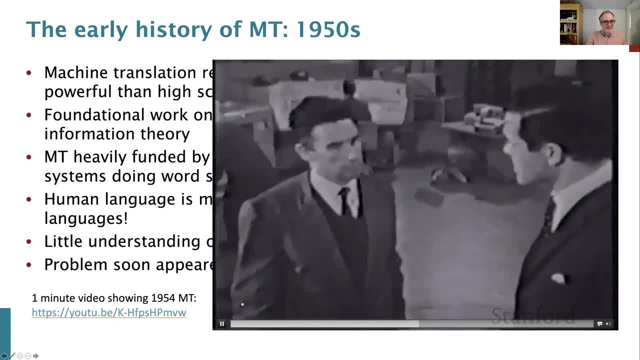 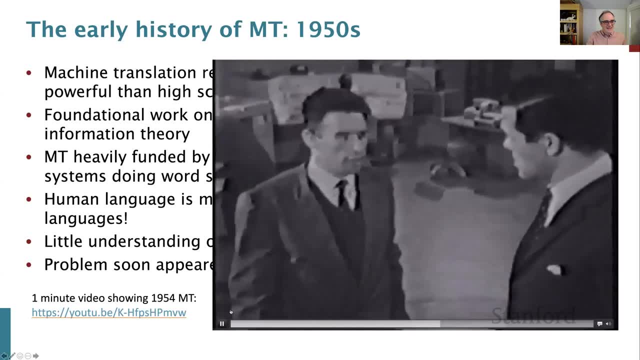 And finally, Mr McDaniel, does this mean the end of human translators? I'd say yes for translators of scientific and technical material, but as regards poetry and novels, no, I don't think we'll ever replace the translators of that type of material. 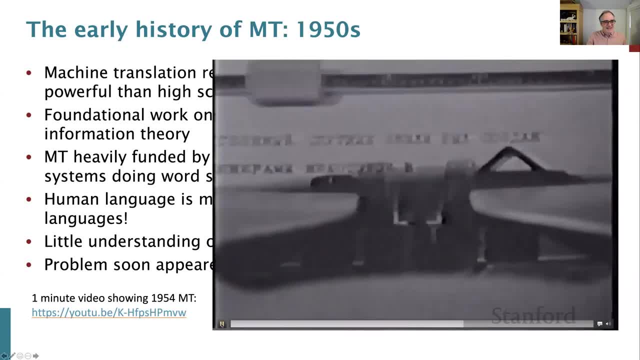 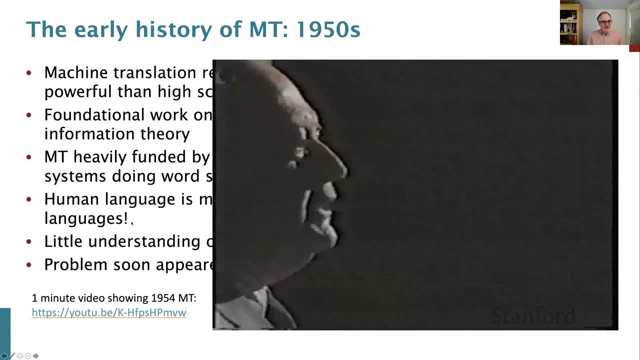 Mr McDaniel, thank you very much. And to save the hype, it ran into deep trouble. But leave me a minute. Yeah, stop there. So the experiments did not go well, And so in retrospect, it's not very surprising that the early work did not work out very well. 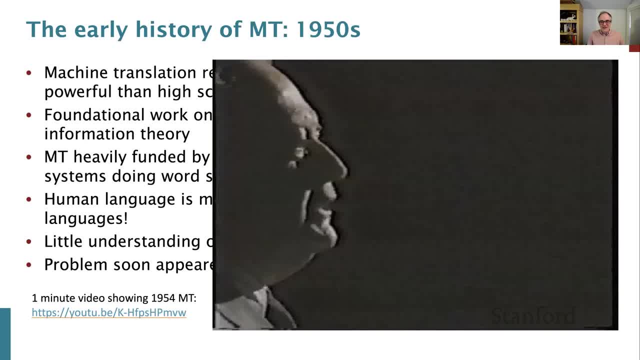 I mean this was in the sort of really beginning of the computer age in the 1950s, but it was also the beginning of, you know, people starting to understand, understand the science of human languages, the field of linguistics. So really people had not 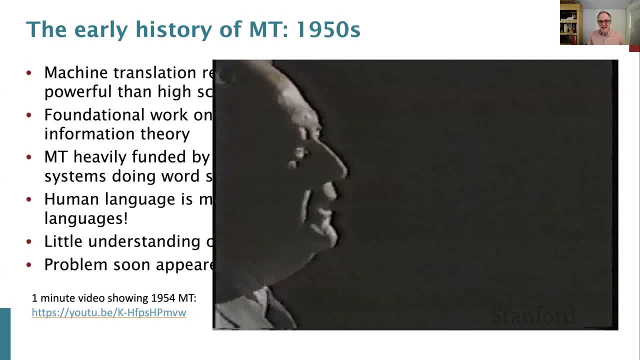 much understanding of either side of what was happening. So what you had was people were trying to write systems on really incredibly primitive computers. right, You know, it's probably the case that now, if you have a USB-C power brick, that it has more computational capacity inside it. 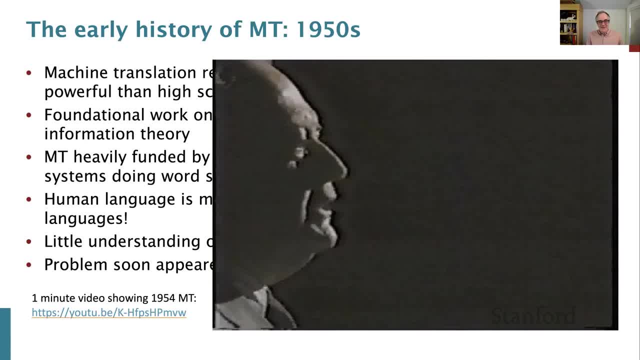 than the computers that they were using to translate, And so, effectively, what you were getting were very simple, rule-based systems and word lookup. So there was sort of like dictionary: lookup a word and get its translation, But that just didn't work well because human languages 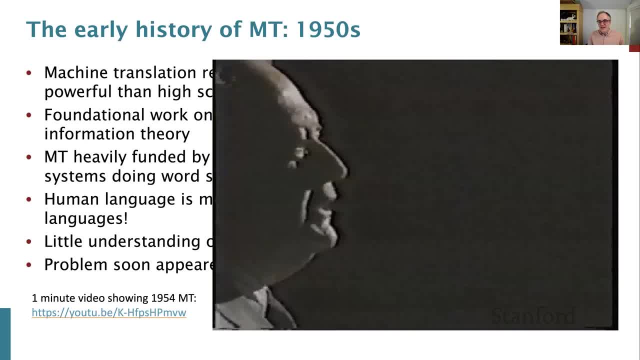 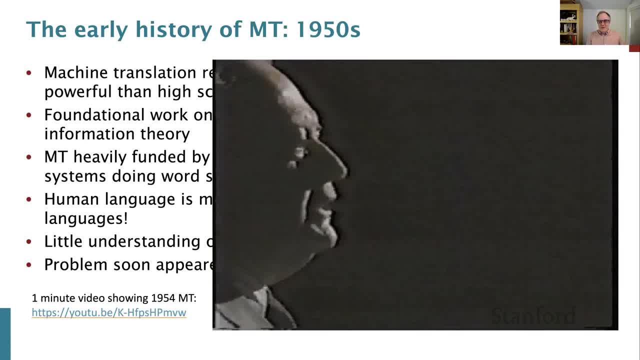 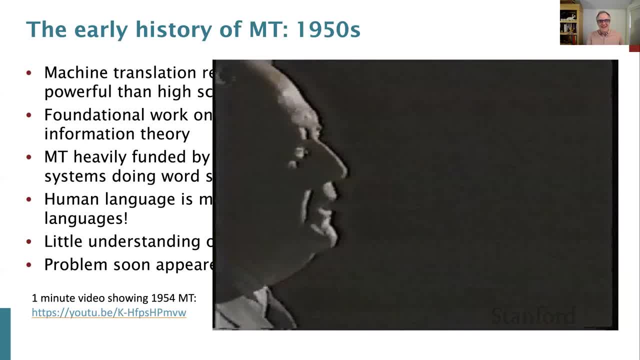 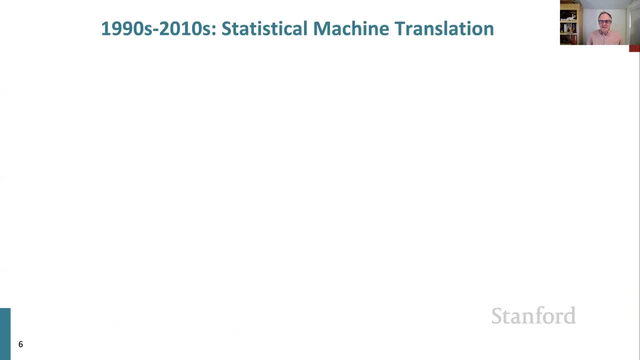 mid-1960s, the ALPAC report, which basically concluded this wasn't working. Oops, Okay. Work then did revive in AI at doing rule-based methods of machine translation in the 90s. But when things really became alive was once you got into the mid-90s and when they were in the period of 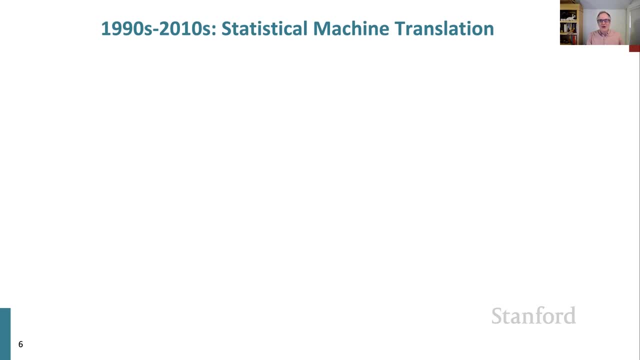 statistical NLP that we've seen in other places in the course. And then the idea began: can we start with just data about translation, ie sentences and their translations, and learn a probabilistic model that can predict the translations of fresh sentences? 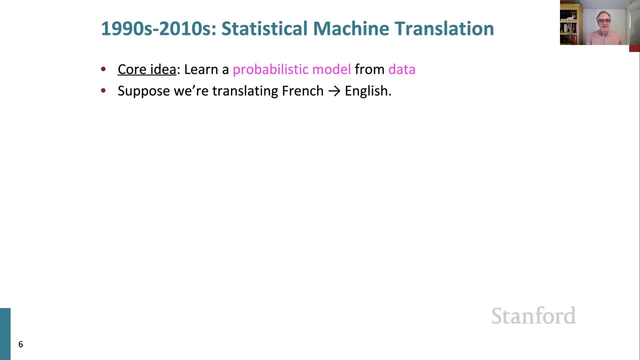 So suppose with translating French into English. So what we want to do is build a probabilistic model that, given a French sentence, we can say what's the probability of different English translations and then we'll choose the most likely translation. We can then found. it was found. 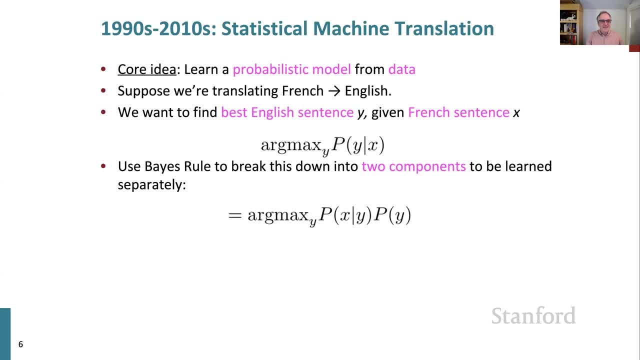 to Felicitas. to break this down into two components by just reversing this with Bayes' rule. So if, in this case, instead we had a probability over English sentences P of Y and then a probability of a French sentence, given an English sentence that people were able to make more progress And it's 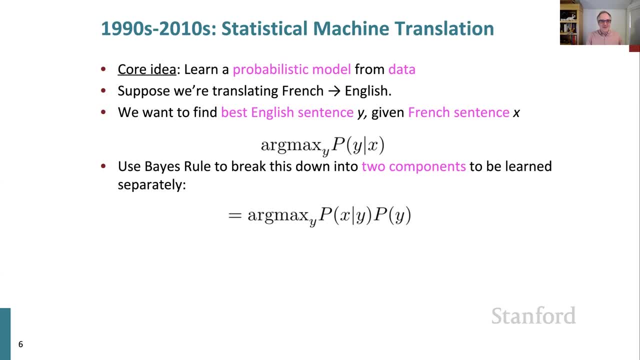 not immediately obvious as to why this should be, because this is just sort of a trivial rewrite with Bayes' rule, but it allowed the problem to be separated into two parts, which proved to be more tractable. So, on the other hand, if you look at this, if you look at this, if you look at the 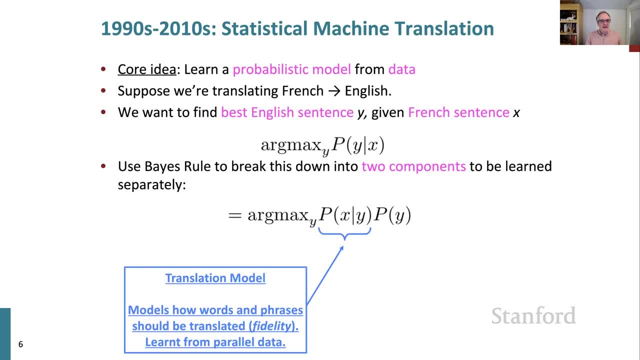 on the left-hand side, you effectively had a translation model where you could just give a probability of words or phrases being translated between the two languages without having to bother about the structural word order of the languages, And then, on the right hand, you saw precisely what. 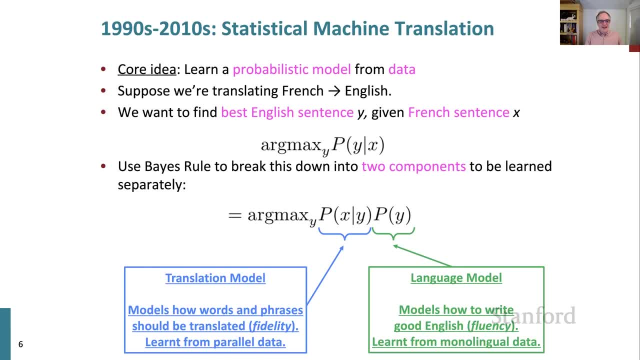 we spent a long time with last week, which is this is just a probabilistic language model. So if we have a very good model of what good fluent English sentences sound like, which we can build just from monolingual data, we can then get it to make sure we're producing sentences that sound good. 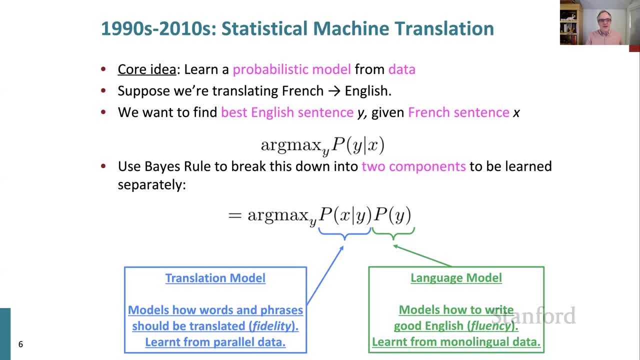 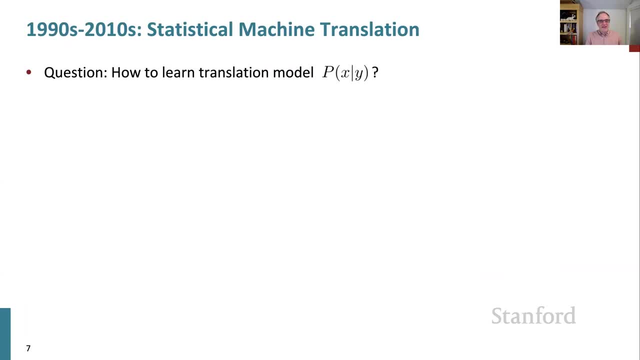 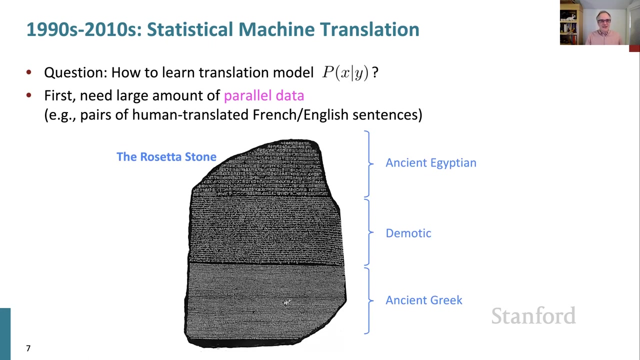 while the translation model hopefully puts the right words into them. So how do we learn the translation model, since we haven't covered that? So the starting point was to get a large amount of parallel data, which is human translated sentences. At this point, it's mandatory that I show a picture of the Rosetta Stone, which is the famous 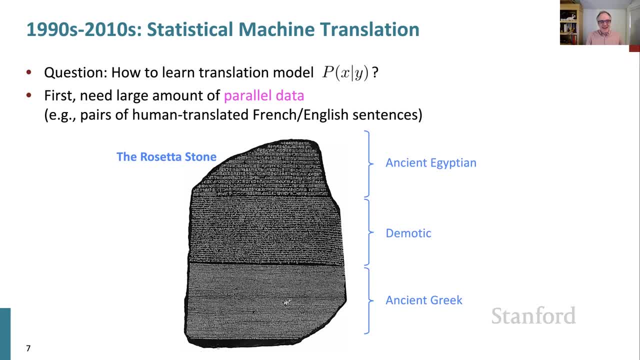 original piece of parallel data that allowed the decoding of Egyptian hieroglyphs because it had the same piece of text in different languages. In the modern world, there are, fortunately for people who build natural language processing systems, quite a few places where parallel data is produced. 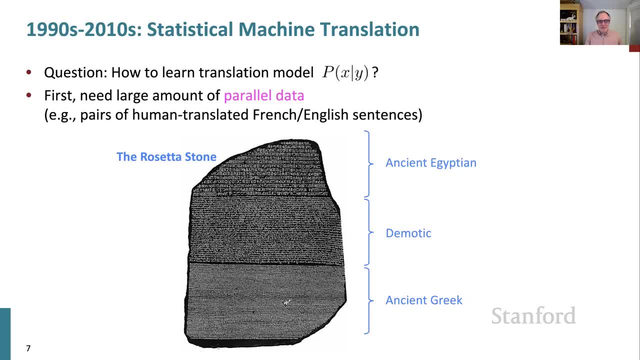 in large quantities. So the European Union produces a huge amount of parallel text across European languages: The French, sorry, not the French. the Canadian Parliament conveniently produces parallel text between French and English and even a limited amount in an institute, Canadian Eskimo. And then the Hong Kong Parliament produces: 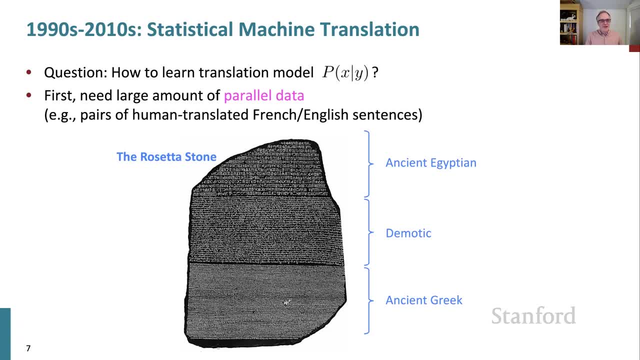 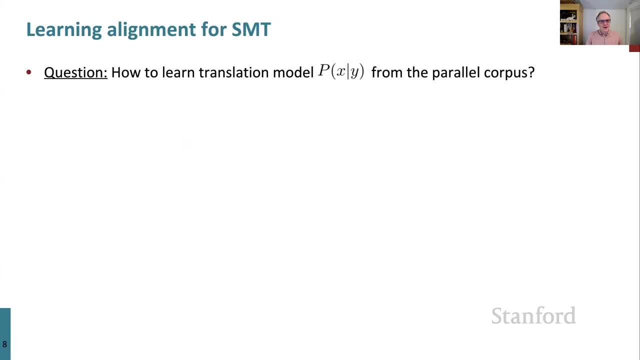 English and Chinese, So there's a fair availability from different sources, and we can use that to build models. So how do we do it, though? All we have is these sentences, and it's not quite obvious how to build a probabilistic model out of those. 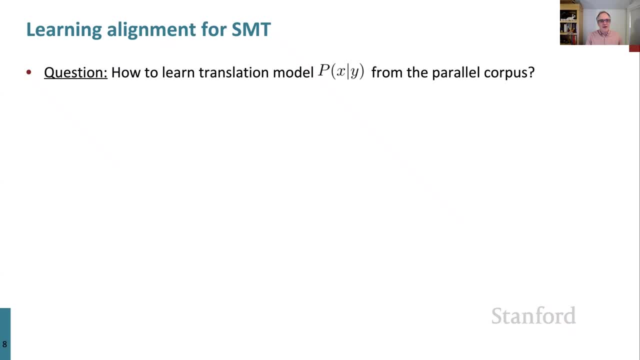 Well, as before, what we want to do is break this problem down. So in this case, what we're going to do is introduce an extra variable which is an alignment Variable. So A is the alignment variable, which is going to give a word level or, sometimes, phrase. 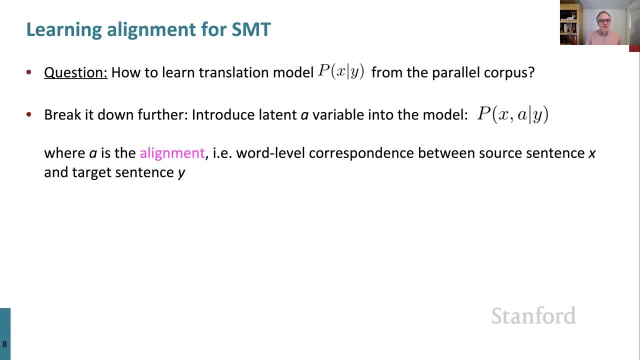 level correspondence between parts of the source sentence and the target sentence. So this is an example of an alignment And so if we could induce this alignment between the two sentences, then we have can have probabilities of pieces of how likely a word or a structure. 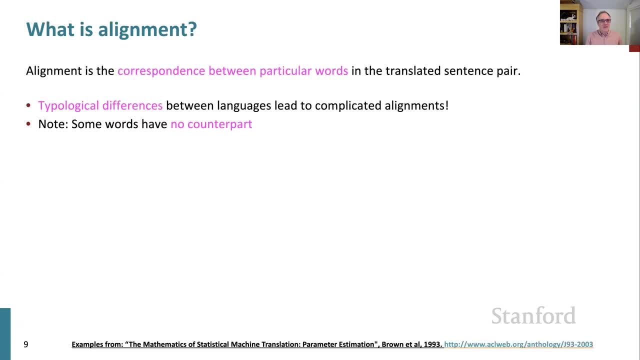 a short phrase is translated in a particular way And in general, you know, alignment is working out the correspondence between words, that is, capturing the grammatical differences between languages. So words will occur in different orders in different languages depending on whether it's a language that puts the subject. 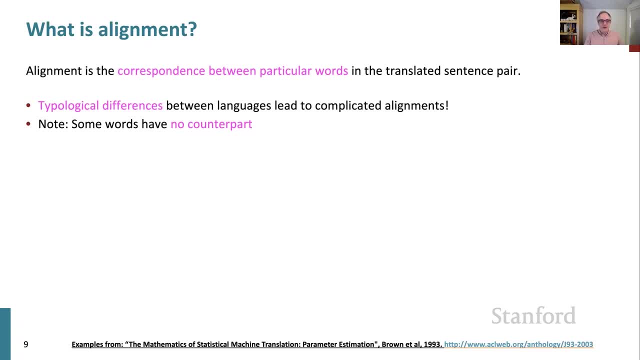 before the verb or the subject after the verb Or the verb before both the subject and the object. And the alignments will also capture something about differences, about the ways that word languages do things. So what we find is that we get every possibility of how words can align between languages. 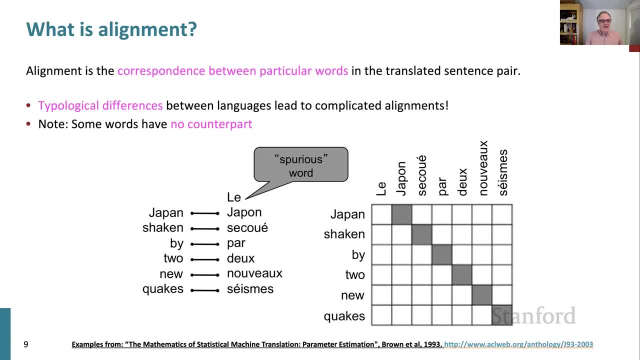 So you can have words that don't get translated at all in the other language. So in French you put a definite article. the before country names like le Japon. So when that gets translated into English you just get Japan. 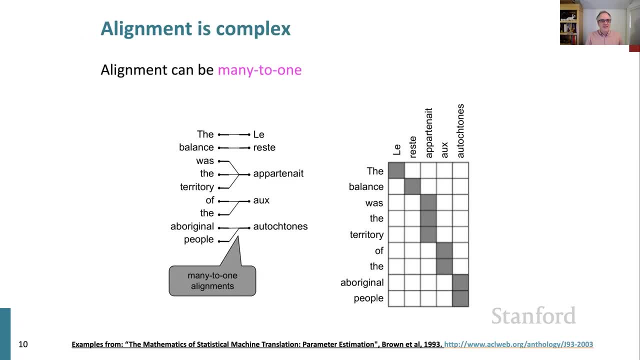 So there's no translation of the the, So it just goes away. On the other hand, you can get many to one translations where one French word gets translated as several English words. So for the last French word it's being translated as Aboriginal people. 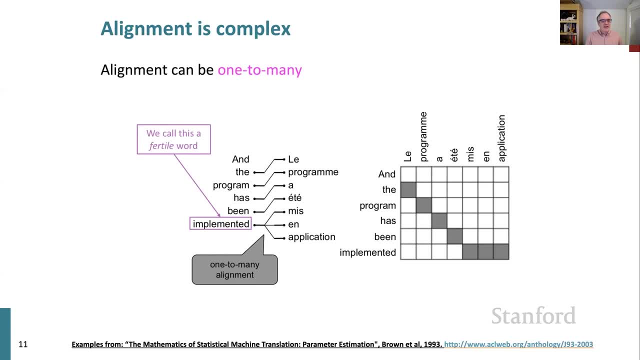 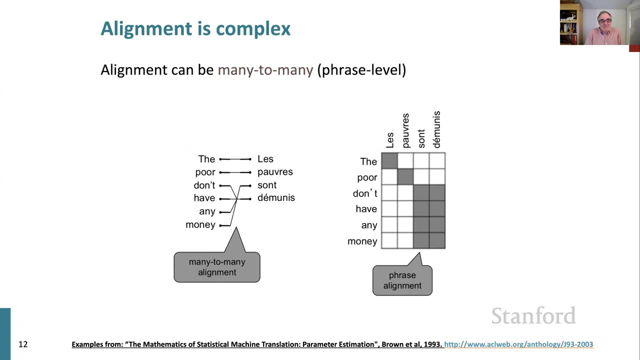 as multiple words. You can get the reverse, where you can have several French words that get translated as one English word. So mise en application is getting translators implemented, And you can get even more complicated ones. So here we sort of have four English words being translated as two French words, but they don't really break down. 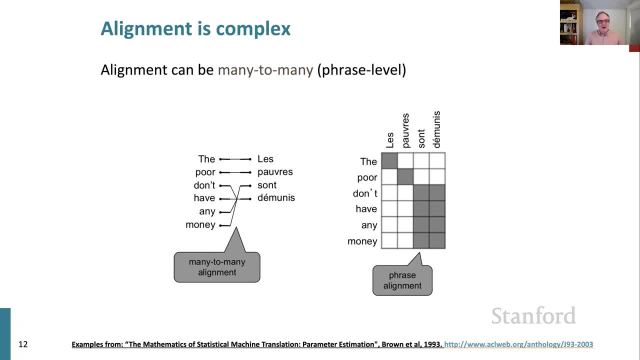 and translate each other well. I mean, these things don't only have to happen across languages, They also happen within the language, when you have different ways of saying the same thing. So another way you might have expressed: the poor don't have any money. 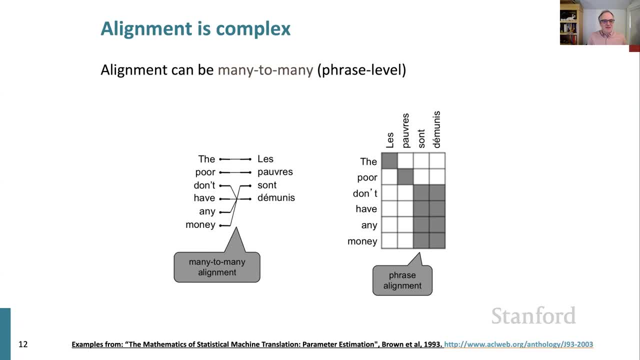 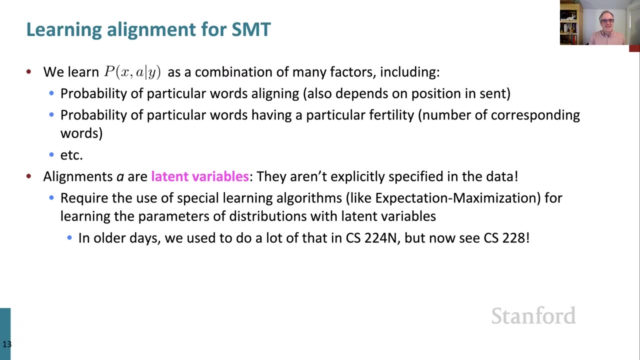 is to say the poor are moneyless, And that's much more similar to how the French is being rendered here, And so even English to English you have the same kind of alignment problem, So probabilistic or statistical machine translation is more common. 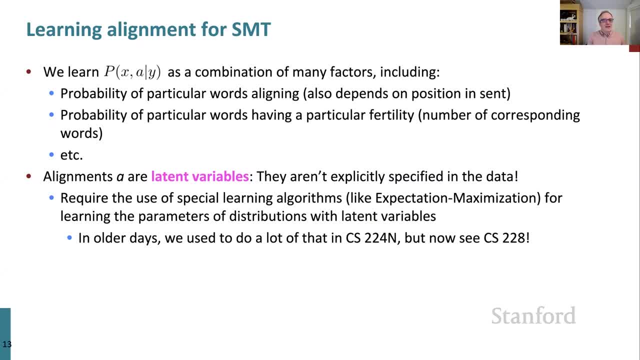 Born. What we wanted to do is learn these alignments And there's a bunch of sources of information you could use. If you start with parallel sentences, you can see how often words and phrases co-occur in parallel sentences. You can look at their. 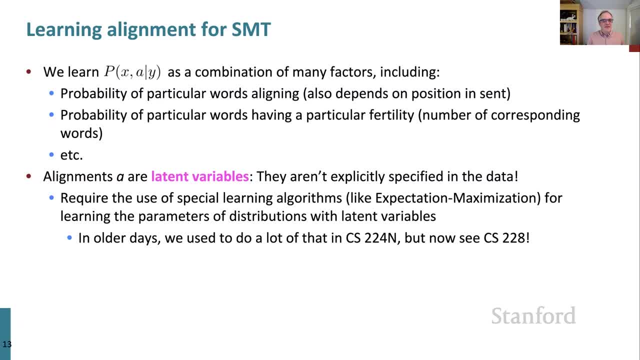 positions in the sentence and figure out what a good alignment is. But alignments are a categorical thing. They're not probabilistic and so they are latent variables, and so you need to use special learning algorithms, like the expectation maximization algorithm for learning about latent variables In the 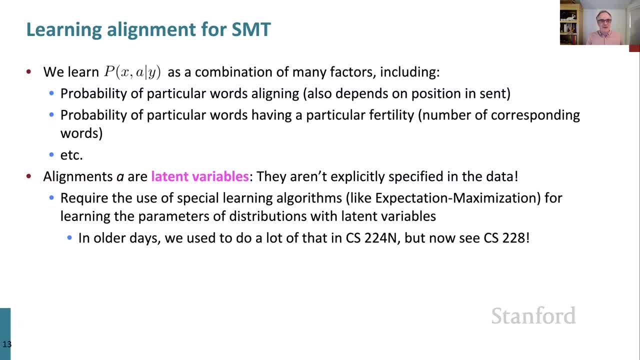 olden days of CS224n, before we started doing it all with deep learning, we spent tons of CS224n dealing with latent variable algorithms, but these days we don't cover that at all and you're going to have to go off and see CS228 if you want to know more about that, and you know we're not really. 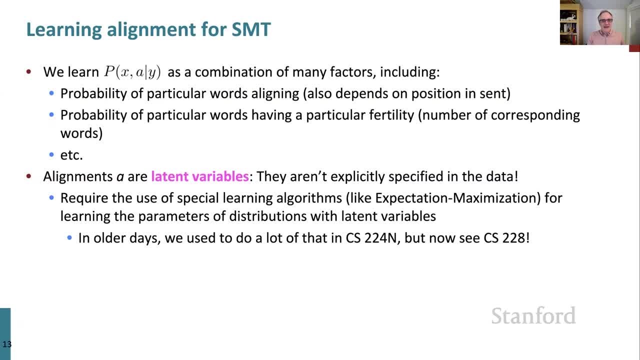 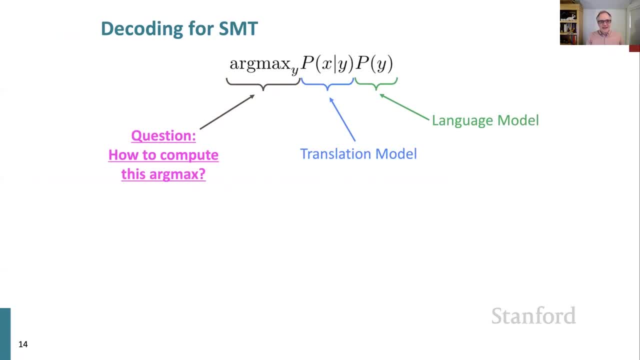 expecting you to understand the details here, but I did then want to say a bit more about how decoding was done in a statistical machine translation system. So what we wanted to do is to say we had a translation model and a language model, and we want to pick out the most likely. 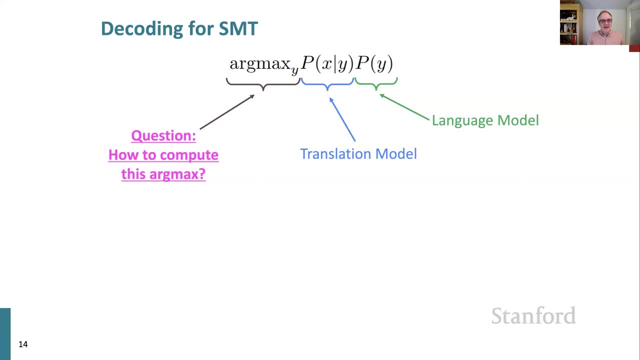 Y, there's the translation of the sentence. and what kind of process could we use to do that? Well, you know, the naive thing is to say: well, let's just enumerate every possible Y and calculate its probability. but we can't possibly do that because there's a number of translation sentences in the 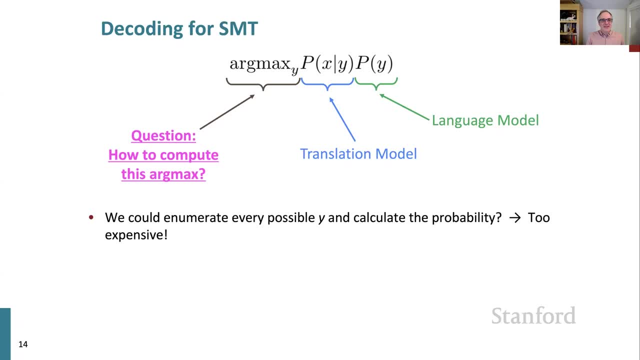 target language that's exponential in the length of the sentence, so that's way too expensive. So we need to have some way to break it down more and well, we had a simple way for language models: we just generated words one at a time and laid out the sentence, and so that seems a reasonable thing. 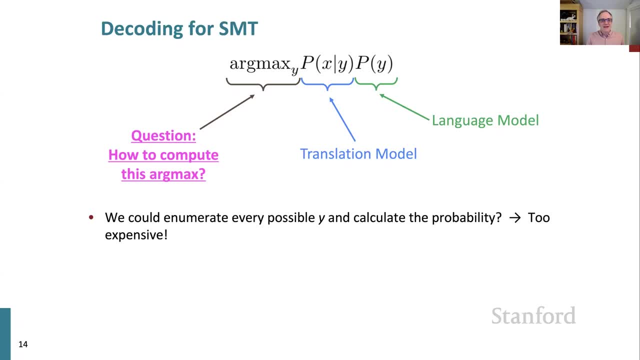 to do, but here we need to deal with the fact that things occur in different orders in source languages and in translations, And so we do that. We do want to break it into pieces with an independence assumption, like the language model, but then we want a way of breaking things apart and exploring it in what's called a decoding. 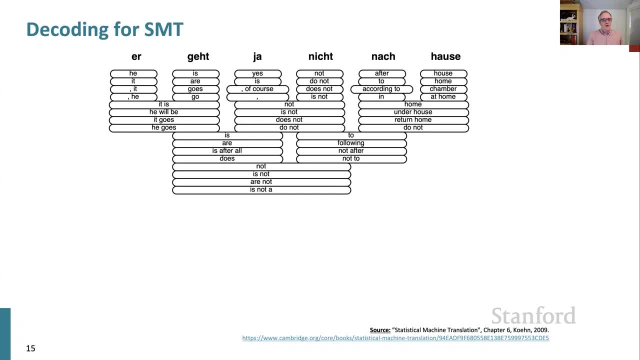 process. So this is the way it was done, So we'd start with a source sentence. so this is a German sentence and, as is standard in German, you're getting this second position verb, so that's probably not in the right place. This is the right position for where the English translation is going to be, so we might need to. 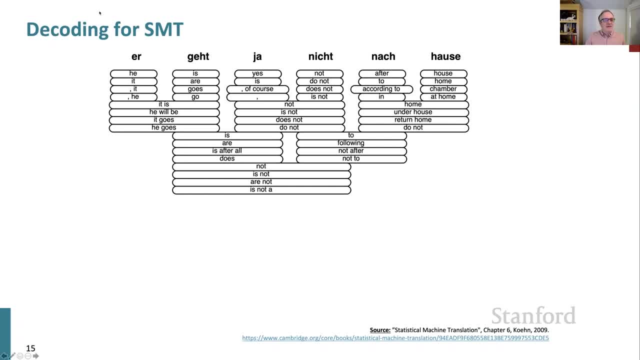 rearrange the words. So what we have is based on the translation model. we have words or phrases that are reasonably likely translations of each German word, or sometimes a German phrase. So these are effectively the Lego pieces out of which we're going to want to create the translation. 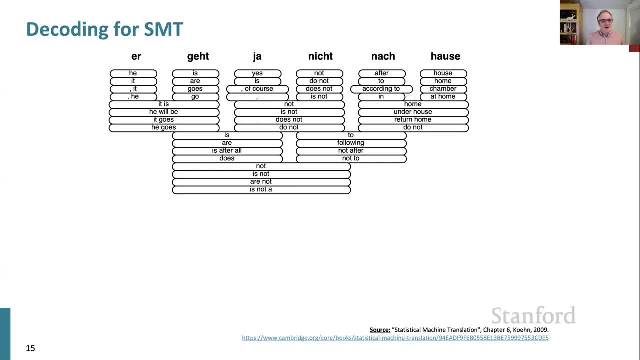 And so then, inside that, what we go, making use of this data, we're going to generate the translation piece by piece, kind of like we did with our newer language models. So we're going to start with an empty translation and then we're going to say, well, we want to use one of these Lego pieces. 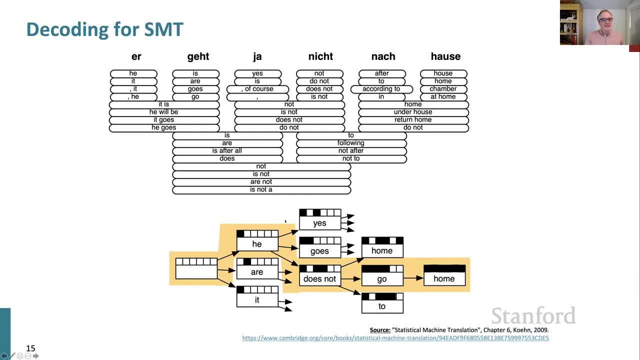 and so we could explore different possible ones. so there's a search process, but one of the possible pieces is we could translate er with he, or we could start the sentence with r, translating the second word. So we could explore various likely possibilities and if we're guided by our language, 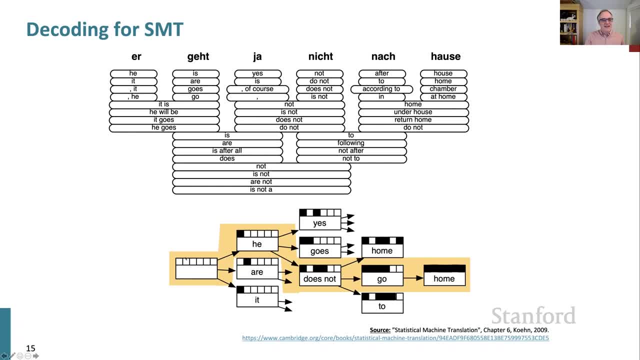 model, it's probably much more likely to start the sentence with he than it is to start the sentence with r, though r is not impossible. Okay, and then the other thing we're doing: with these little blotches of black up the top, we're sort of recording which German words we're going to use. 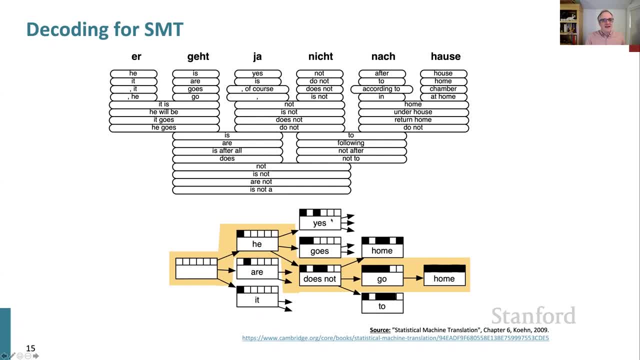 We've translated and so we explore forward in a translation process and we could decide that we could translate next the second word goes, or we could translate the negation here and translate that as does not. when we explore various continuations- and in the process I'll go through in more detail later- when we do the neural equivalent, We sort of do this search. 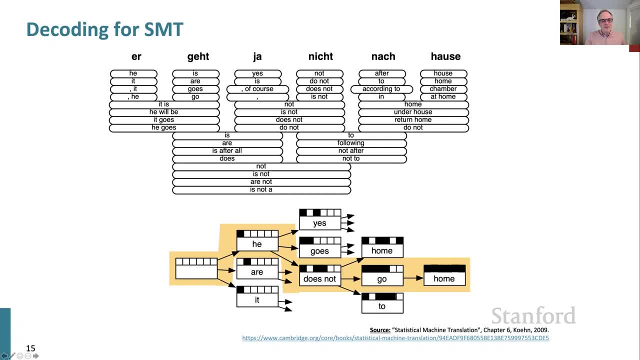 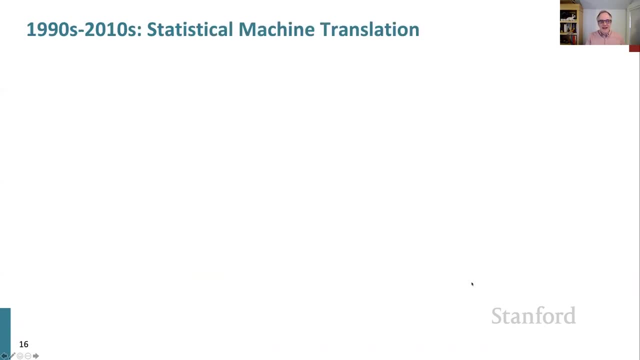 where we explore likely translations and prune, and eventually we've translated the whole of the input sentence and have worked out a fairly likely translation. he does not go home and that's what we'll use as the translation. Okay, so in the period from about 1997 to around 2013. 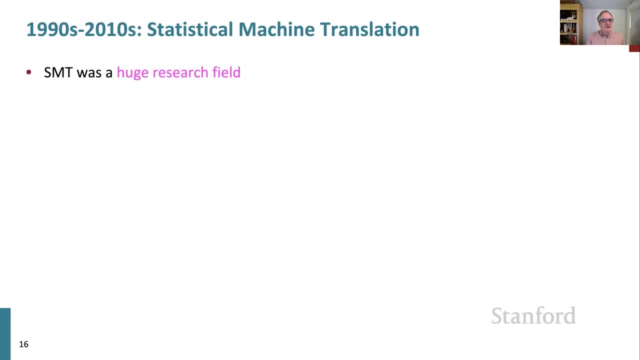 the introduction of machine translation was a huge research field. The best systems were extremely complex. They had hundreds of details that I certainly haven't mentioned here. The systems had lots of separately designed and built components. so I mentioned a language model and a translation model, but they had lots of other components for reordering models and inflection. 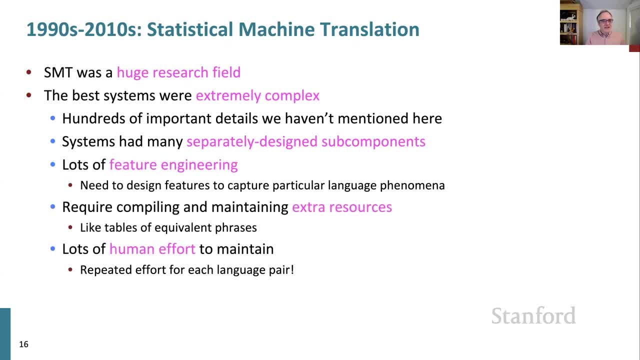 models and other things. There was lots of feature engineering. the models also made use of lots of extra resources and there were lots of human effort to maintain, But nevertheless they were already fairly successful. So Google Translate launched in the mid-2000s and people thought, wow, this is amazing, You could start to get. 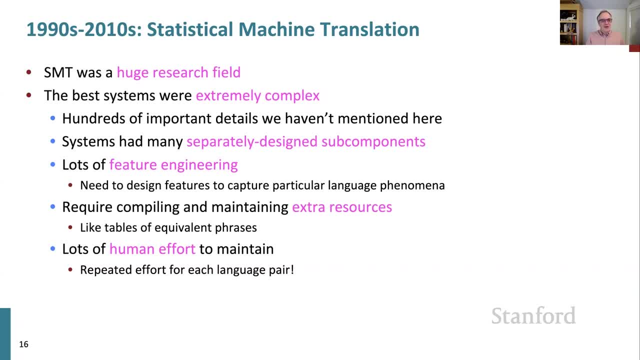 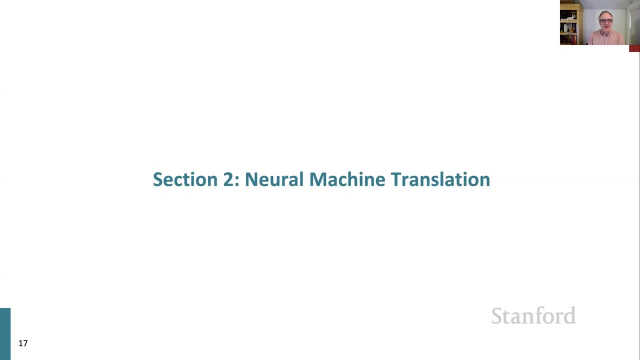 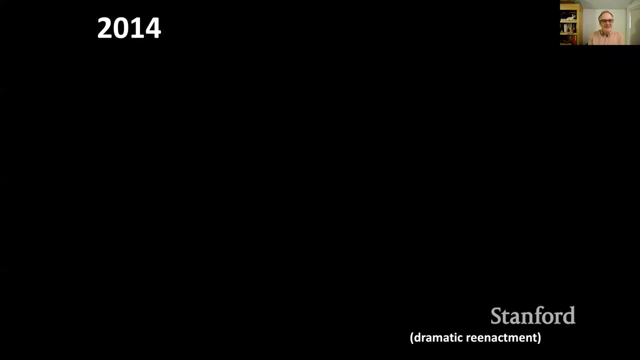 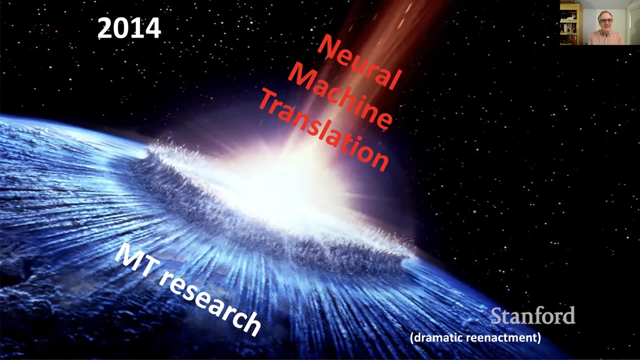 sort of semi-decent automatic translations for different webpages. But that was chugging along well enough, and then we got to 2014.. And really with enormous suddenness, people then worked out ways of doing machine translation using a large neural network. 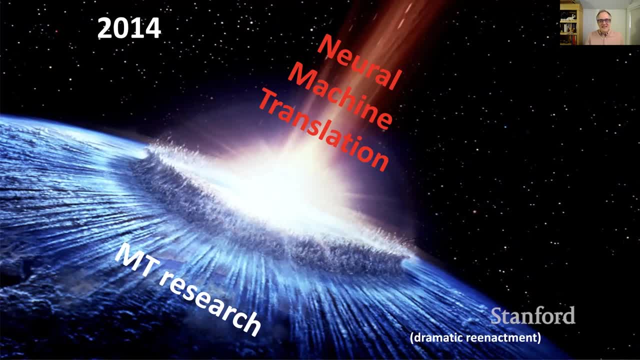 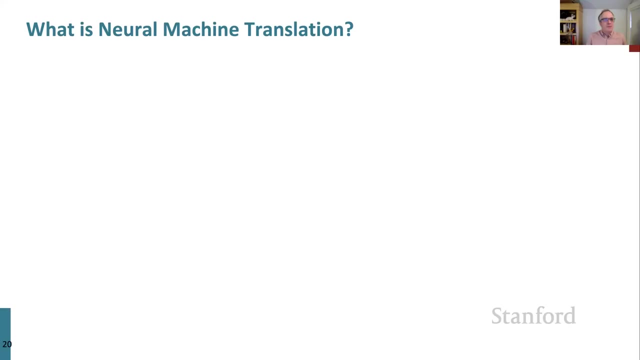 And these large neural networks proved to be just extremely successful and largely blew away everything that preceded it. So for the next big part of the lecture, what I'd like to do is tell you something about neural machine translation. Neural machine translation, well, it means you're using a neural network to do machine translation. 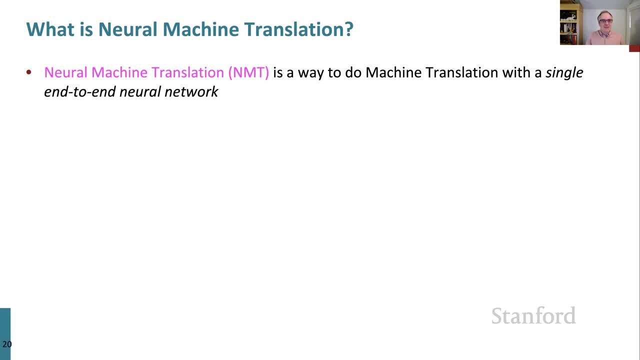 but in practice it's meant slightly more than that. It has meant that we're going to build one very large neural network which completely does translation end to end. So we're going to have a large neural network. We're going to feed in the source sentence into 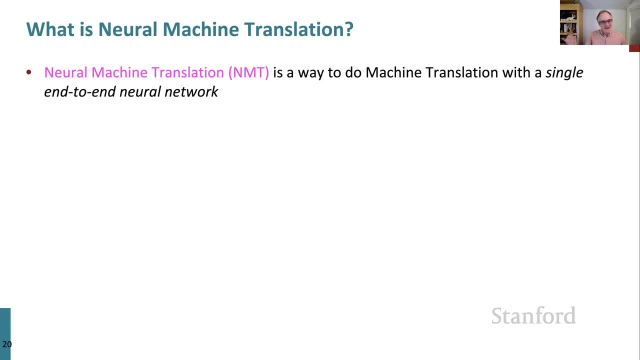 the input And what's going to come out as the output of the neural network is the translation of the sentence. We're going to train that model end to end on parallel sentences, And it's the entire system rather than being lots of separate components. 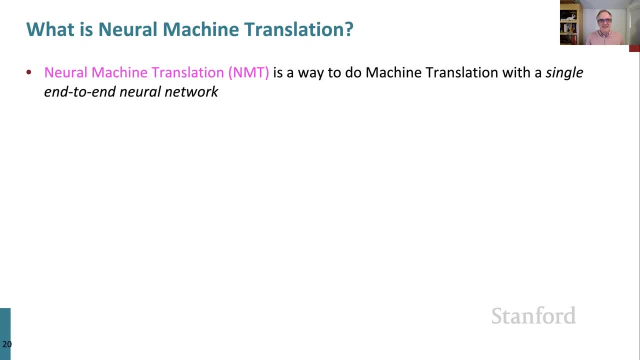 There's an old fashioned machine translation system and we'll see that in a bit. So these neural network architectures are called sequence to sequence models, or commonly abbreviated seek to seek, And they involve two neural networks. Here it says two RNNs, The 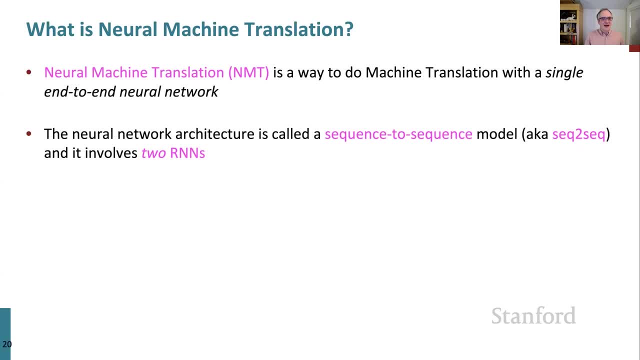 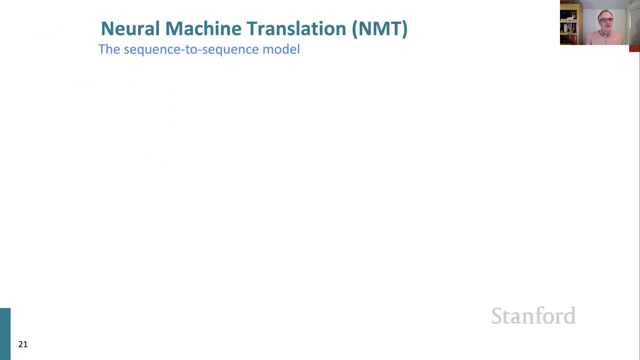 version I'm presenting now has two RNNs, but more generally they involve two neural networks. There's one neural network that is going to encode the source sentence. So if we have a source sentence here, we are going to encode that sentence And while we know about a way that we can do that, so using the kind of LSTMs that we 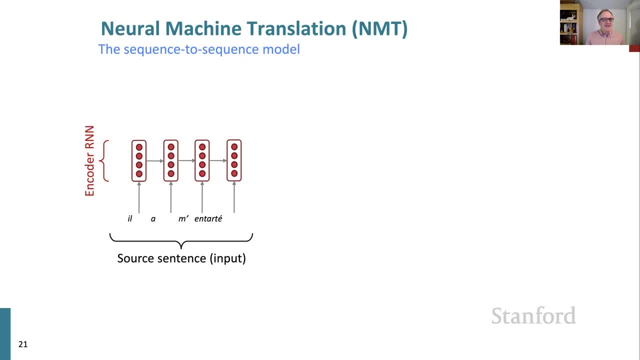 saw last class, we can start at the beginning and go through a sentence and update the hidden state each time, And that will give us a representation of the content of the source sentence. So that's the first step. So this is the first sequence model which encodes the source sentence, And we'll use the idea that. 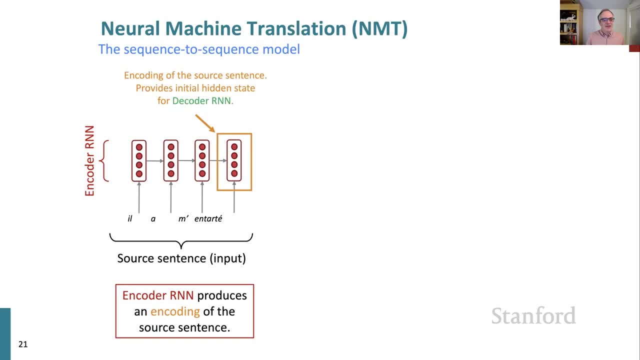 the final hidden state of the encoder RNN is going to, in a sense, represent the source sentence And we're going to feed it in directly as the initial hidden state for the decoder RNN. So then, on the other side of the picture, we have our decoder RNN. 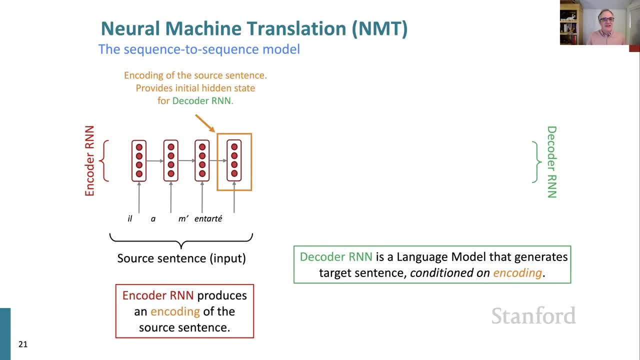 And it's a language that we're going to be using for the decoder RNN, And it's a language that we're going to be using for the decoder RNN, And it's a language model that's going to generate a target sentence conditioned on the 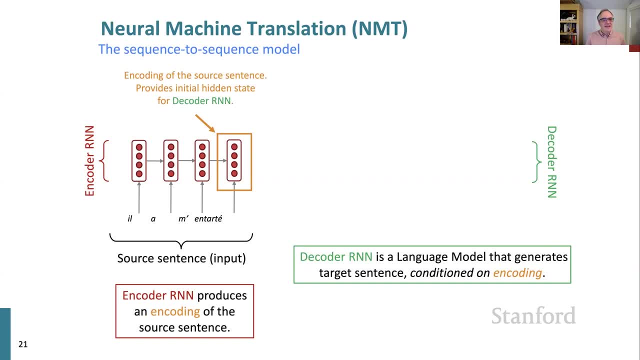 final hidden state of the encoder RNN. So we're going to start with the input of start symbol, We're going to feed in the hidden state from the encoder RNN And now this second green RNN has completely separate parameters. I might just emphasize, But we do the same kind of LSTM. 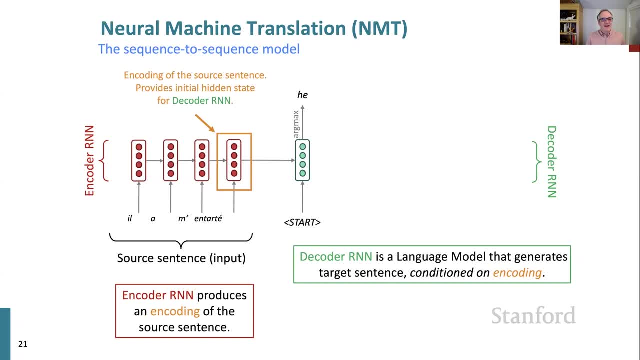 computations and generate the encoder RNN. And so on the left-hand side we have the first word of the sentence, he. And so then doing LSTM generation, just like last class. we copy that down as the next input. We run the next step of the LSTM generate: another word hit, copy it down and chug along. 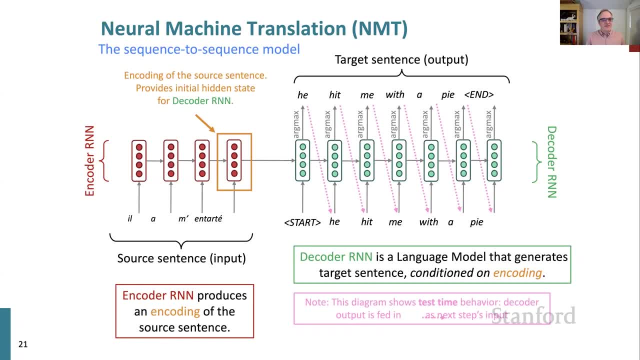 And we've translated the sentence. So this is showing the test time behavior when we're generating the next sentence For the training time behavior. when we have parallel sentences, we're still using the same kind of sequence-to-sequence model, but we're doing it. 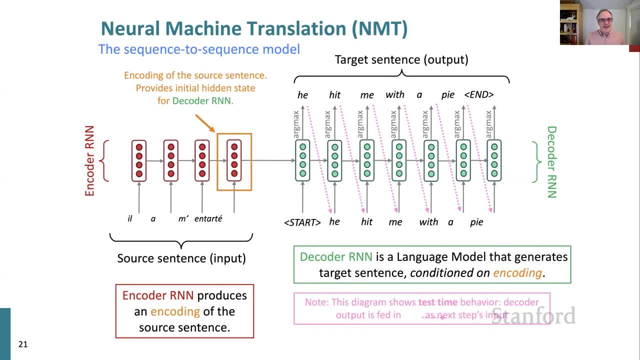 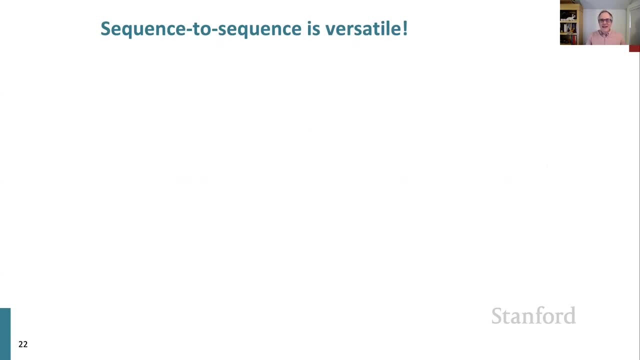 with the decoder part, just like training a language model where we're wanting to do teacher forcing and predict each word that's actually found in the source language sentence. Sequence-to-sequence models have been an incredibly powerful, widely used workhorse in neural networks for NLP. 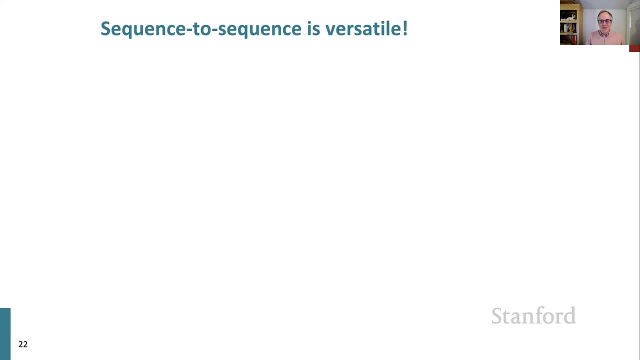 So although historically machine translation was the first big use of them and is sort of the canonical use, they're used everywhere else as well. So you can do many other NLP tasks for them. So you can do summarization, You can think of text. 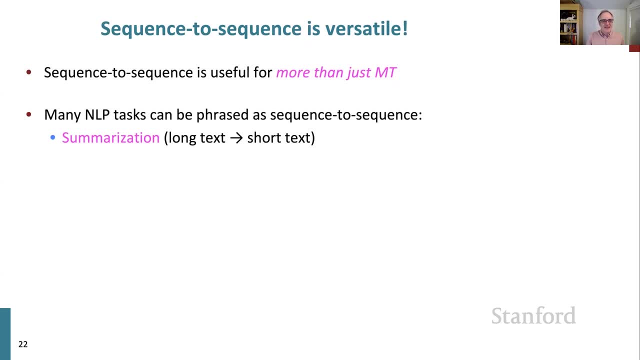 summarization as translating a long text into a short text. But you can use them for other things that are in no way a translation whatsoever. So they're commonly used for neural dialogue systems. So the encoder will encode the previous two utterances, say, and then you will use the decoder. 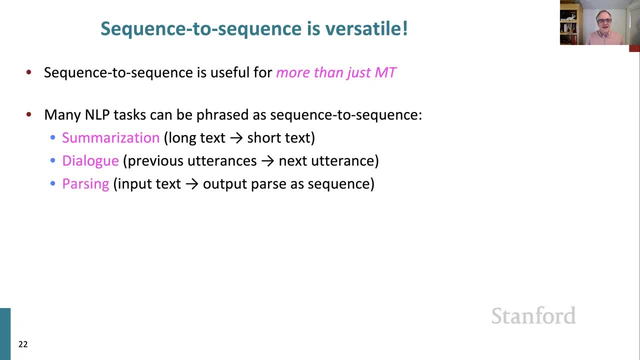 to generate a next utterance. Some other uses, for example, are even freakier but have proven to be quite successful. So if you have any way of representing the pars of a sentence as a string, and if you sort of think a little, it's fairly obvious how you can turn the pars of a sentence. 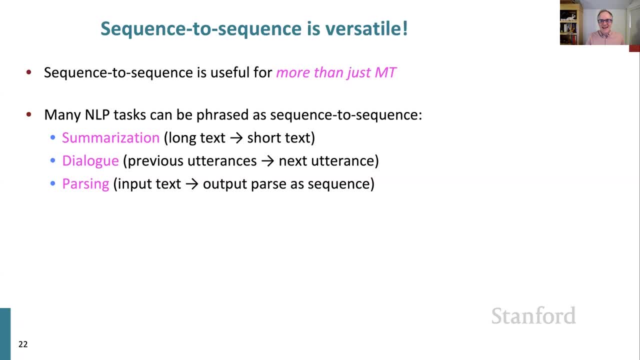 into a string by just making use of extra syntax like parentheses, or putting in explicit words: left arc, right arc shifts, like the transition systems that you used for assignment three. well then, we could say: let's use the encoder. feed the input sentence to the encoder. 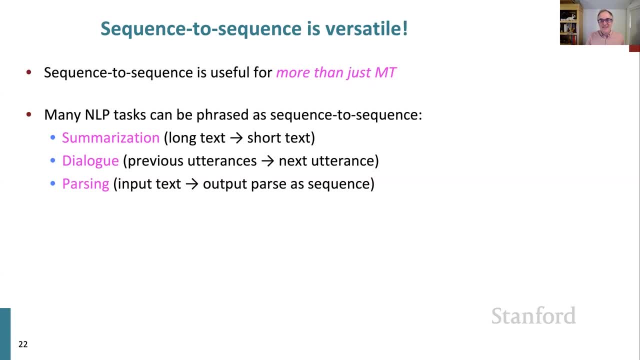 and let it output the transition sequence of our dependency parser And, somewhat surprisingly, that actually works well as another way to build a dependency parser or other kinds of parser. These models have also been applied not just to natural languages, but to other kinds of languages, including music and also programming language code, So you can. 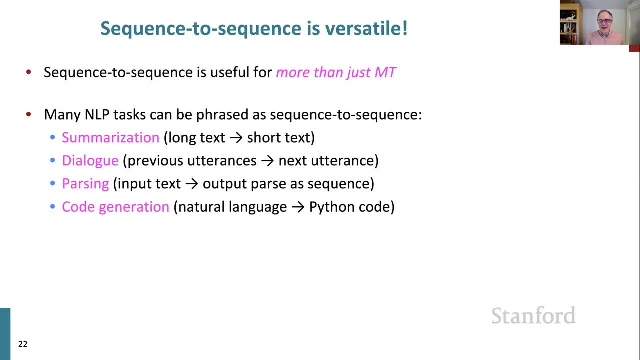 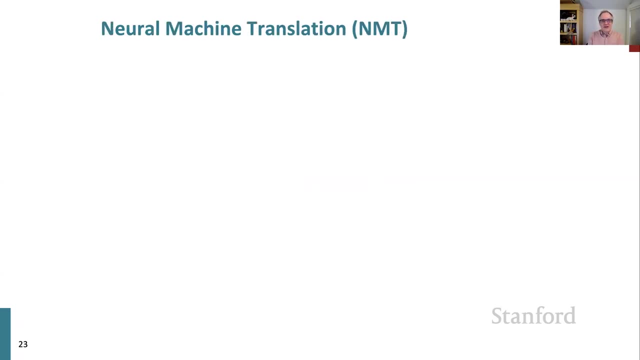 train a seek-to-seek system where it reads in pseudocode in natural language and it generates out python code And if you have a good enough one, it can do the assignment for you. So the essential new idea here with our sequence to sequence models is we have an example of 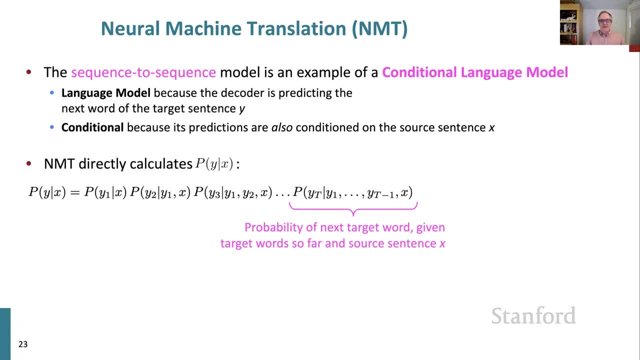 conditional language models. So previously, the main thing we were doing was just to start at the beginning of the sentence and generate a sentence based on nothing. But here we have something that is going to determine, that is going to condition what we should produce. So we have a 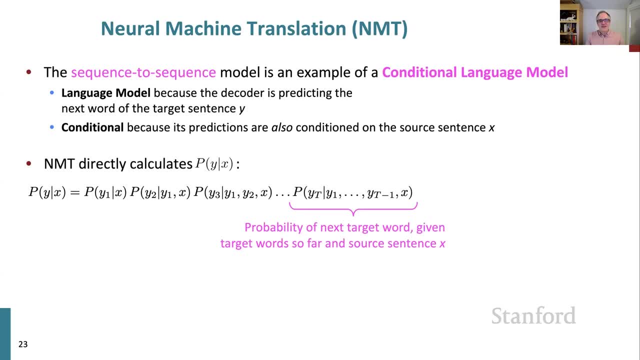 a source sentence and that's going to strongly determine what is a good translation. And so, to achieve that, what we're going to do is have some way of transferring information about the source sentence from the encoder to trigger what the decoder should do And the two standard ways of 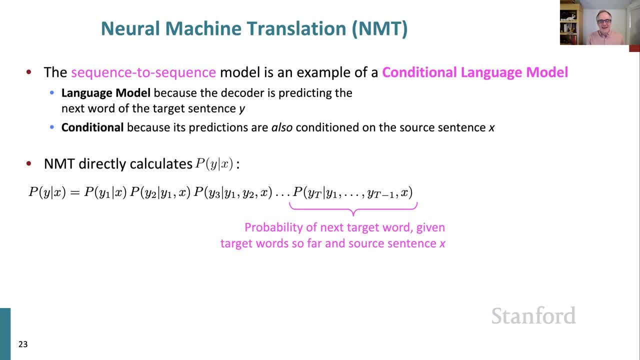 doing that are you either feed in a hidden state as the initial hidden state to the decoder, or sometimes you will feed something in as the initial input to the decoder, And so in neural machine translation we're directly calculating this conditional model: probability of target. 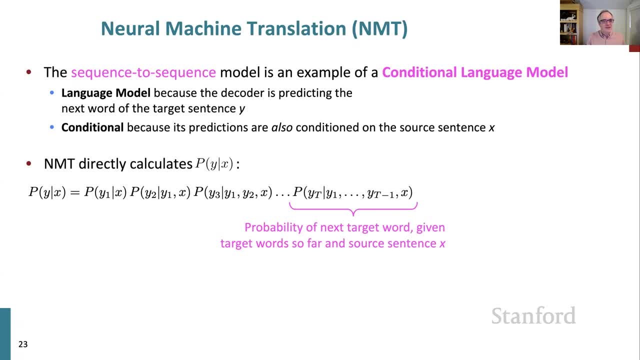 language sentence given source language sentence. And so, at each step, as we break down the word by word, we're going to be able to calculate the probability of target language sentence. And so, at each step, as we break down the word by word, we're going to be able to calculate the 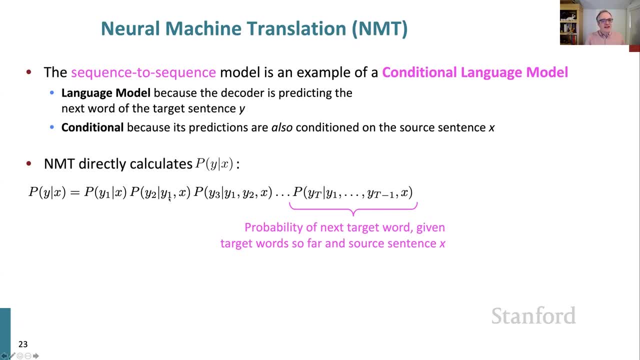 probability of target language sentence. And so, at each step, as we break down the word by word, generation, that we're conditioning not only on previous words of the target language, but also each time on our source language, sentence X. Because of this, we actually know a ton more. 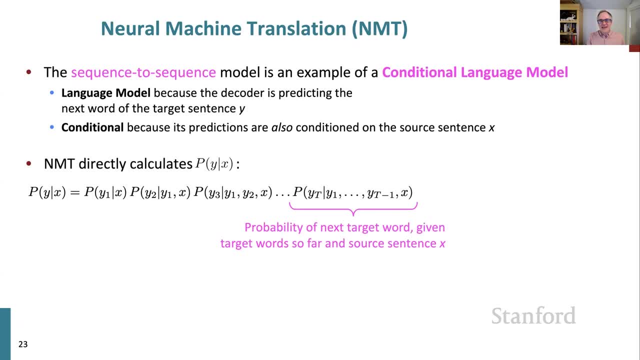 about what our sentence that we generate should be. So if you look at the perplexities of these kind of conditional language models, you will find that, like the numbers I showed last time, they usually are the same. So if you look at the perplexities of these kind of conditional 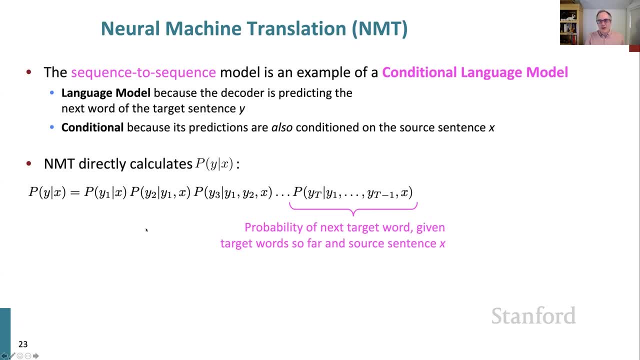 language models. you will find that, like the numbers I showed last time, they usually have almost freakily low perplexities- that you will have models with perplexities that are something like four or even less. sometimes you know 2.5, because you get a lot of information about what 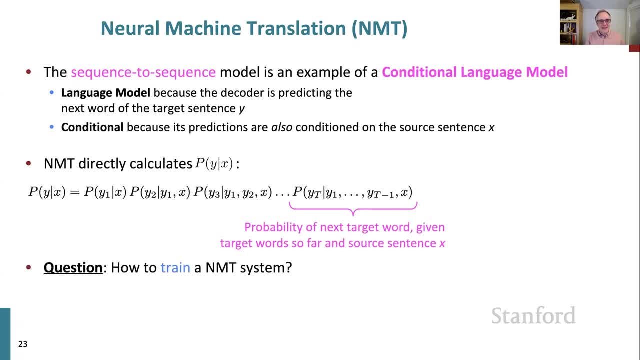 words you should be generating. Okay, So then we have the same questions as we had for language models in general: how to train a neural machine translation system and then how to use it at runtime. So let's go through some of the questions that we have. So let's go through some of the 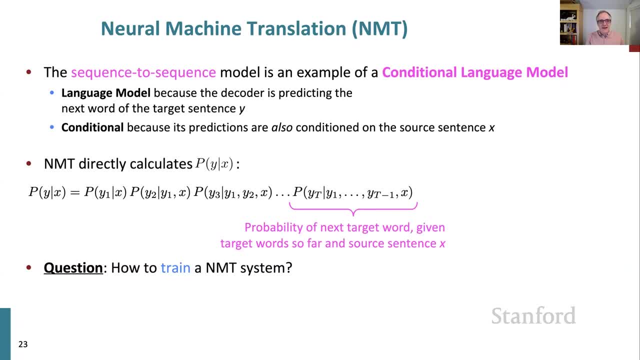 questions that we have. So let's go through some of the questions that we have. So let's go through both of those in a bit more detail. So the first step is we get a large parallel corpus. So we run off to the European Union, for example, and we grab a lot of parallel English, French data from. 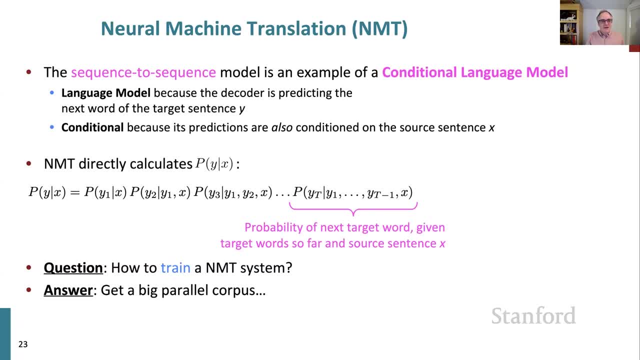 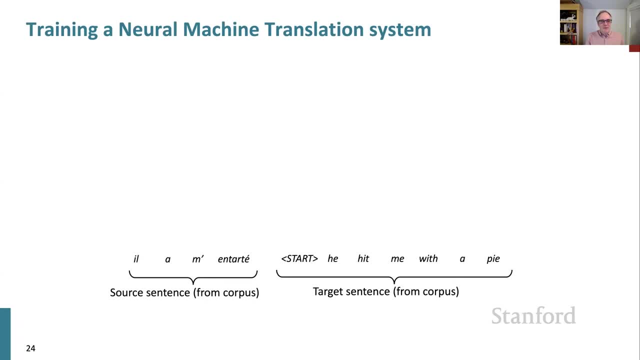 the European Parliament proceedings. So then, once we have our parallel sentences, what we're going to do is take batches of sentences, and we're going to take batches of sentences and we're going to gather them and run them into an effective, consistent grid, And then we take the number of 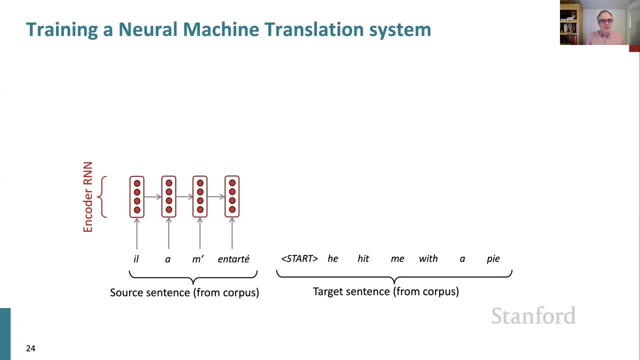 of source sentences and target sentences will encode the source sentence without encoder lst m, will feed its final hidden state into a target lst m, And this one we're now then going to train word by word by comparing what it predicts as the most likely word to be produced. So it's a very useful 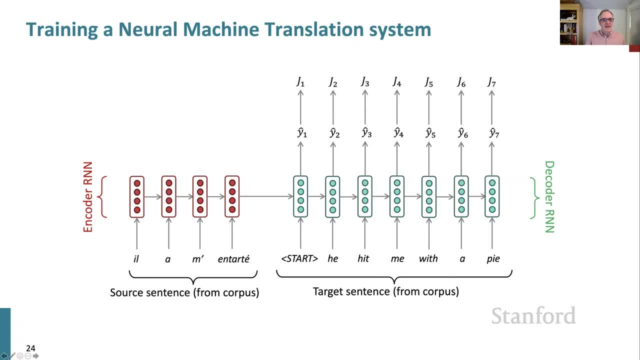 opportunity versus what the actual first word and then the actual second word is, And to the extent that we get it wrong, we're going to suffer some loss. So this is going to be the negative log probability of generating the correct next word: he. 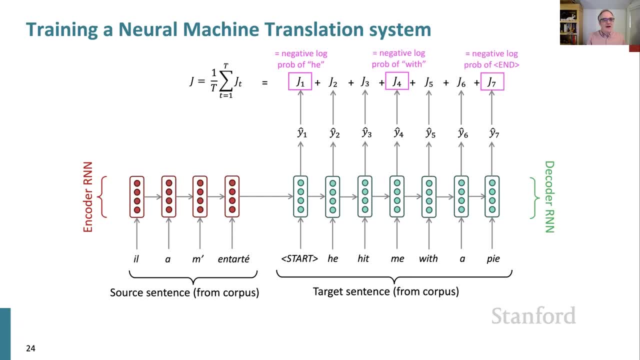 and so on along the sentence. And so, in the same way that we saw last time for language models, we can work out our overall loss for the sentence doing this teacher forcing style: generate one word at a time. calculate a loss relative to the word. 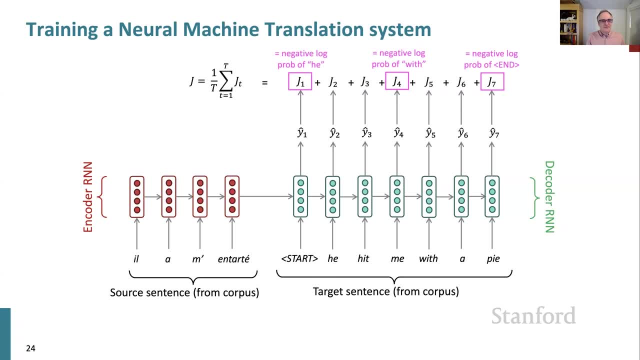 that you should have produced, And so that loss then gives us information that we can back propagate through the entire network. And the crucial thing about these sequence to sequence models that has made them extremely successful in practice is that the entire thing is optimized as a single system, end-to-end. 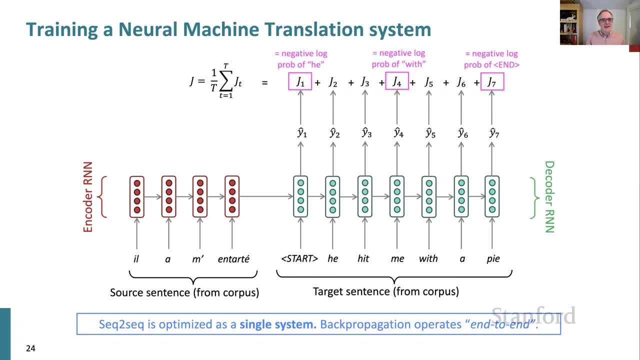 So, starting with our final loss, we back, propagate it right through the system. So we not only update all the parameters of the decoder model, but we also update all of the parameters of the encoder model, which in turn will influence what conditioning gets passed over from the encoder to the decoder. 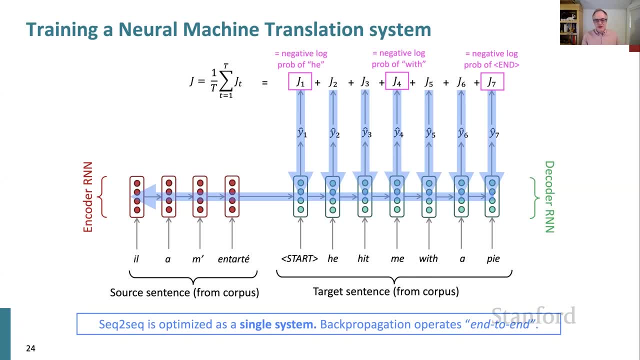 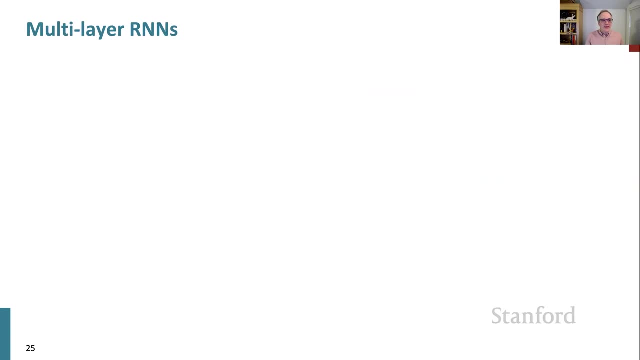 So this moment is a good moment for me to return to the three slides that I skipped running out of time at the end of last time, which is to mention multi-layer RNNs, So the RNNs that we've looked at so far. 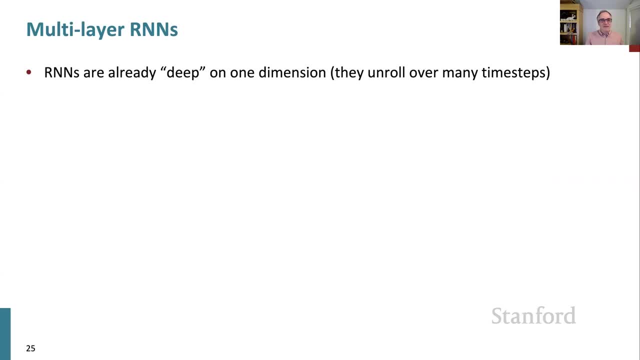 are already deep on one dimension then unroll horizontally over many time steps, but they've been shallow in that there's just been a single layer of recurrent structure above our sentences. We can also make them deepen the other dimension by applying multiple RNNs on top of each other. 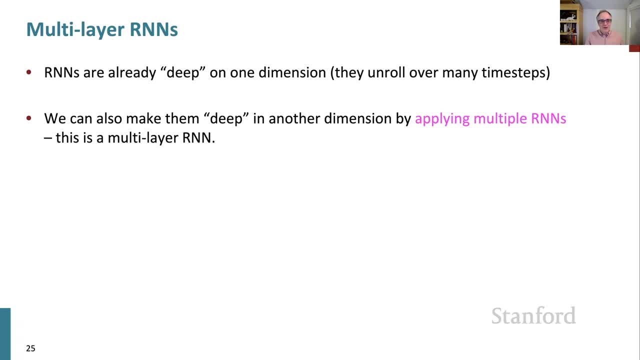 And this gives us a multi-layer RNN, often also called a stacked RNN. And having a multi-layer RNN allows us the network to compute more complex representations. Simply put, the lower RNNs tend to compute lower level features and the higher RNNs should compute higher level features. 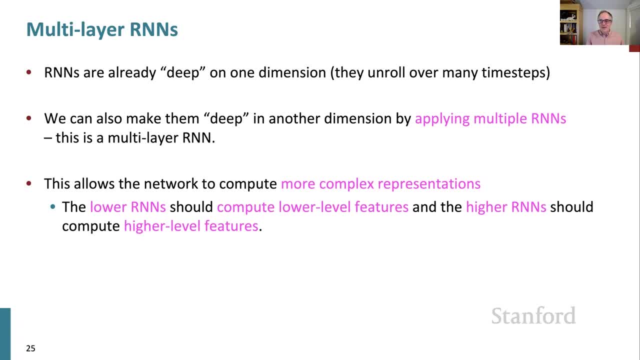 And just like in other neural networks, whether it's feed forward networks or the kind of networks you see in vision systems- you get much greater power and success by having a stack of multiple layers of recurrent neural networks. right That you might think. 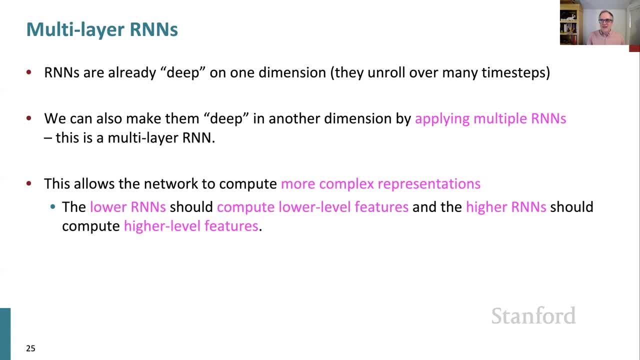 that. oh, there are two things I could do. I could have a single LSTM with a hidden state of dimension 2000,. or I could have four layers of LSTMs with a hidden state of 500 each, And it shouldn't make any difference. 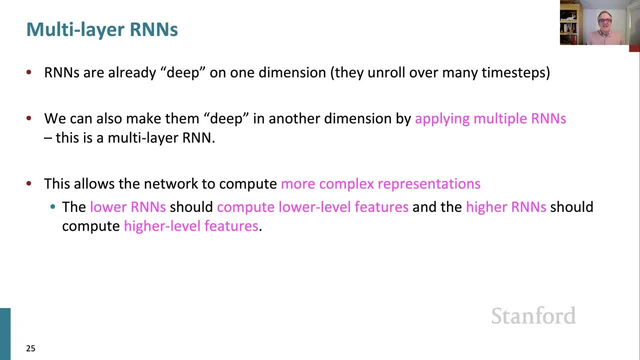 because I've got the same number of parameters roughly. but that's not true. In practice it does make a big difference and multi-layer or stacked RNNs are more powerful, And I think that's a good thing. There's a good student question here. 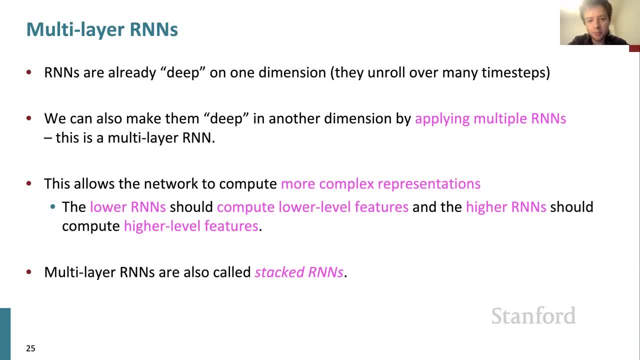 about what lower level versus higher level features mean in this context. Sure, Yeah, so I mean in some sense- these are kind of somewhat flimsy ways you know terms, those meaning isn't precise, But typically what that's meaning. 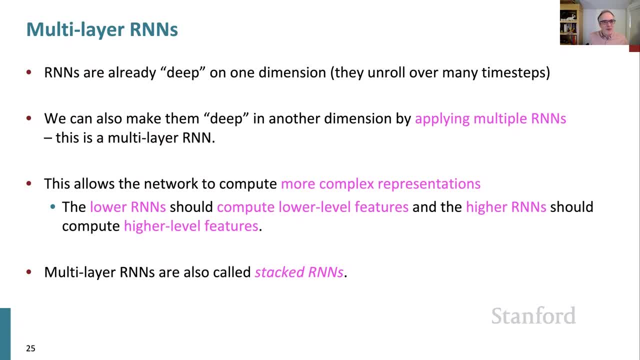 is that lower level features and knowing sort of more basic things about words and phrases, So that commonly might be things like what part of speech is this word Or are these words the name of a person or the name of a company, Whereas higher level features refer to things. 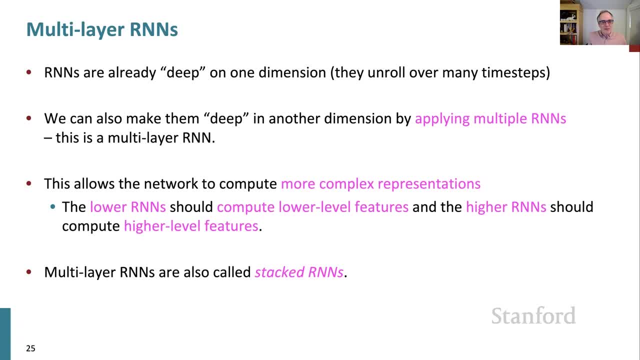 that are at a higher semantic level. So knowing more about the overall structure of a sentence, knowing something about what it means whether a phrase has positive or negative connotations, what it's semantics are when you put together several words into an idiomatic phrase. 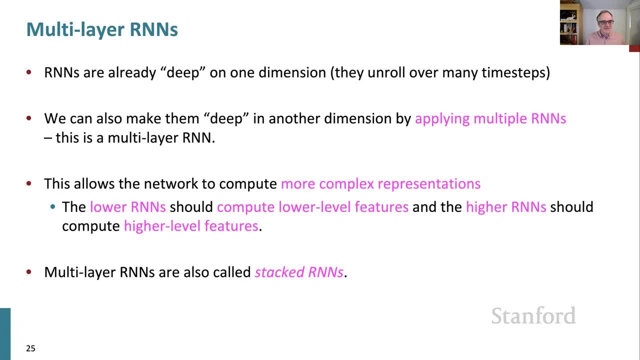 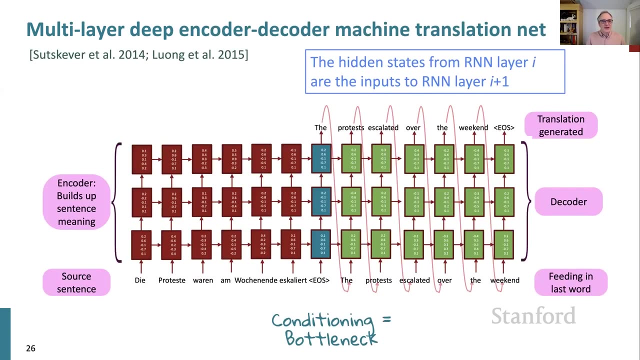 are roughly the higher level kinds of things. Okay, Jump ahead. Okay. so when we build one of these end-to-end neural machine translation systems, if we want them to work well, single layer LSTM encode to decode in your machine translation systems just don't work well. 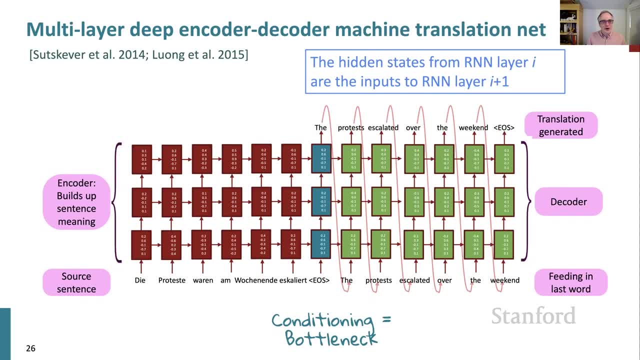 But you can build something that is no more complex than the model that I've just explained. now that does work pretty well by making it, but is more neural. So it's more like a multiple layer stack LSTM neural machine translation system. So, therefore, the picture looks like this: 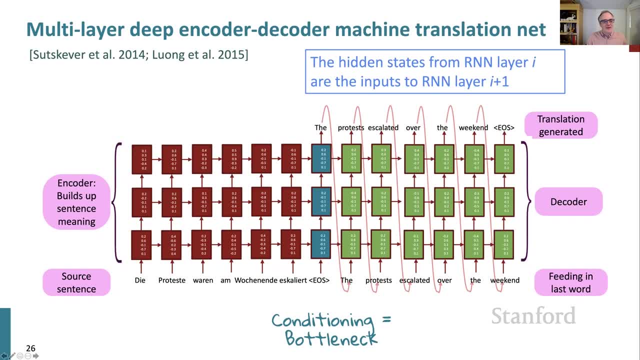 So we've got this multi-layer LSTM that's going through the source sentence, And so now, at each point in time, we calculate a new hidden representation that, rather than stopping there, we sort of feed it as the the input into another layer of LSTM. 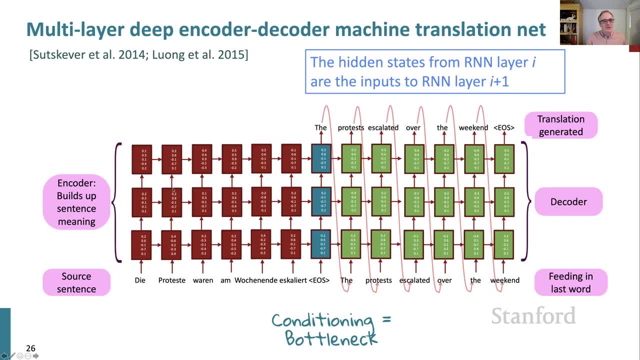 in the standard way. it's new hidden representation and the output of it. we feed into a third layer of lstm and so we run that right along, and so our representation of the source sentence from our encoder is then this stack of three hidden layers, and then that we use um to then feed in as the 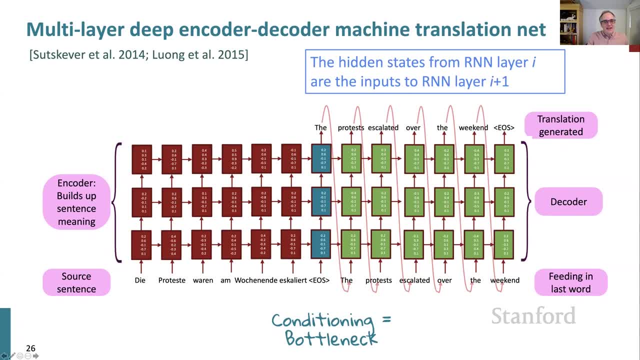 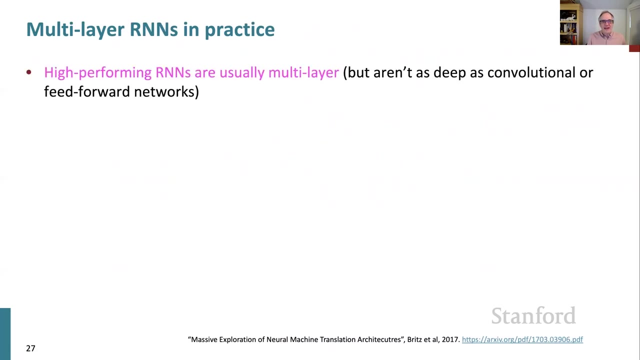 initial um as the initial hidden layer into then sort of generating um translations or um for training, the model of comparing to losses. so this is kind of what the picture of a lstm encoder, decoder, neural machine translation system really looks like. so in particular, um you know to give. 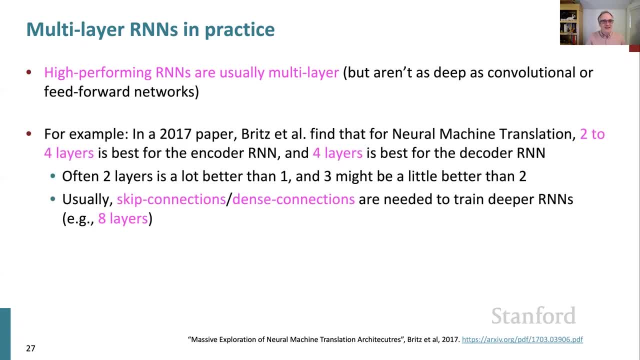 you some idea of that? um. so a 2017 paper by denny brits and others that what they found was that for the encoder rnn um, it worked best if it had two to four layers and um four layers was best for the decoder rnn um and the details. 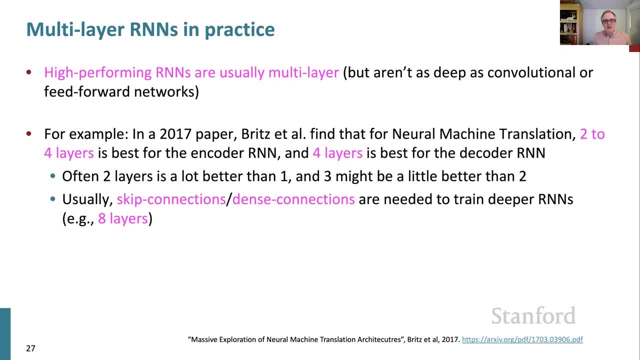 here, like for a lot of neural nets, depends so much on what you're doing and how much data you have and things like that. but you know as rules of thumb to have in your head it's almost perfectly the case that having a two-layer lstm works a lot better than having a one-layer lstm. 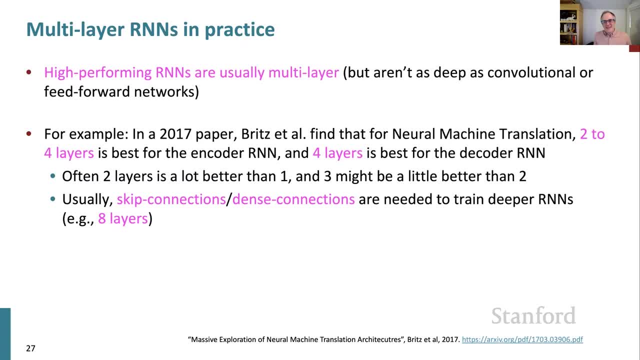 after that things become much less clear. you know it's not so infrequent that if you try three layers it's a fraction better than two, but not really. and if you try four layers it's actually getting worse again. you know it depends on how much data etc you have. at any rate, um, it's normally very hard. 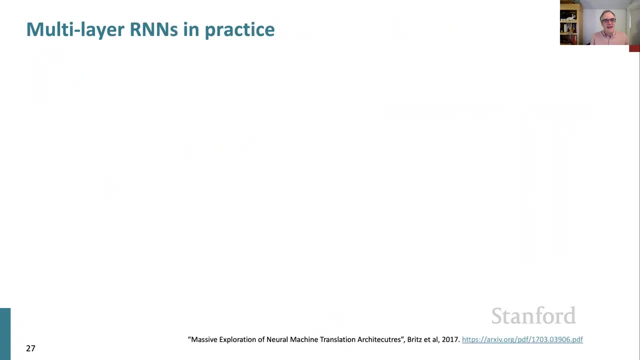 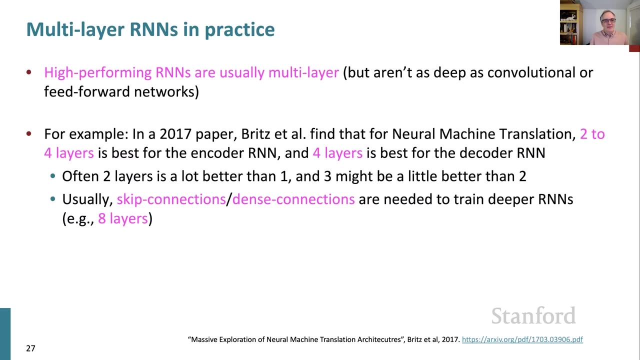 to get better results with the model architecture that i just showed back here. um to get better results with more than four layers of lstm um normally to do deeper um lstm models and get even better results you have to be adding extra skip connections of the kind that i talked about. 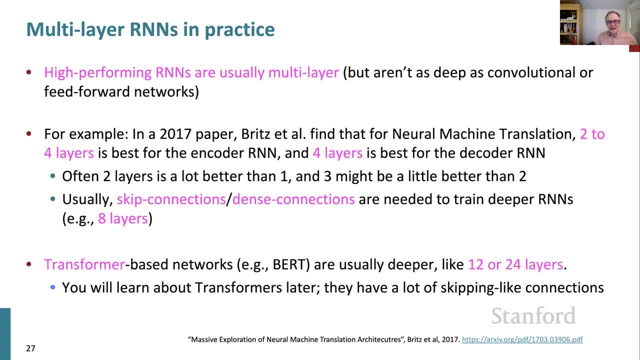 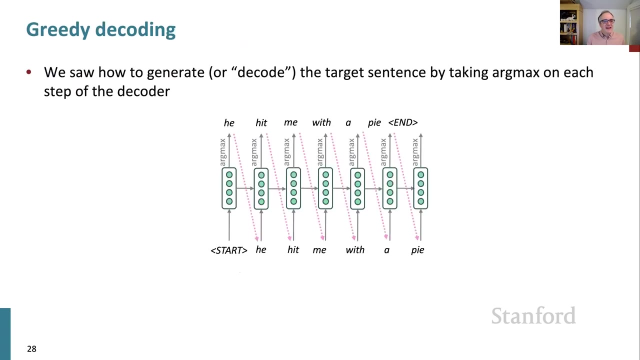 at the very end of the last class um next week, john is going to talk about transformer based contrast. for fairly fundamental reasons, they're typically um much deeper, but we'll leave discussing them until we get on further um. so that was how we trained the model um, so let's. 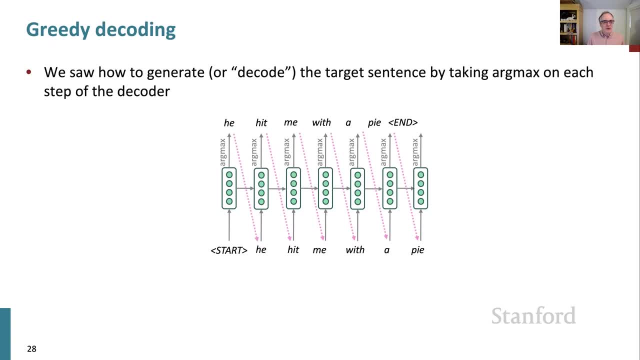 just go a bit more through what the possibilities are for decoding and explore a more complex form of decoding than we've looked at. the simplest way to decode is the one that we presented so far. so that we have our lstm, we start generate a hidden state. um, it has a probability distribution. 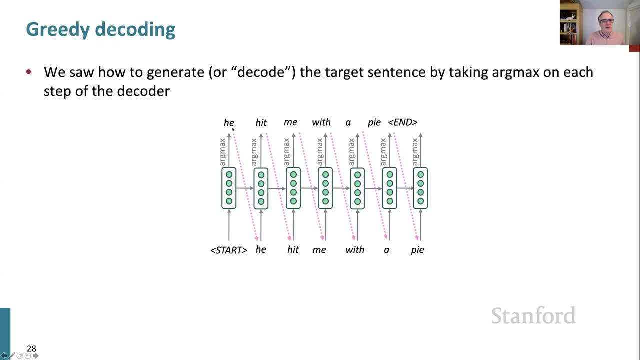 over words and you choose the most probable one, the argmax, and you say he and you copy it down and you repeat over. so doing this is referred to as greedy decoding- taking the most reasonable probable word on each step, and it's sort of the obvious thing to do and doesn't seem like it could. 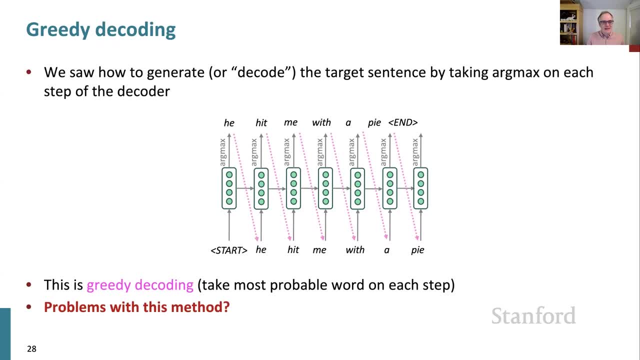 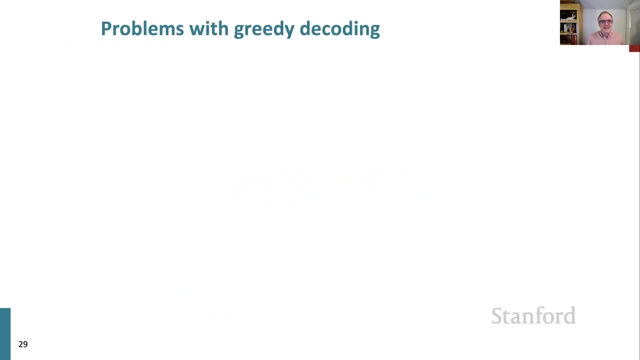 be a bad thing to do, but it turns out that it actually can be a fairly problematic thing to do, and the idea of that is that, you know, with greedy decoding you're sort of taking locally what seems the best choice and then you're stuck with it and you have no way to undo decisions. um so, 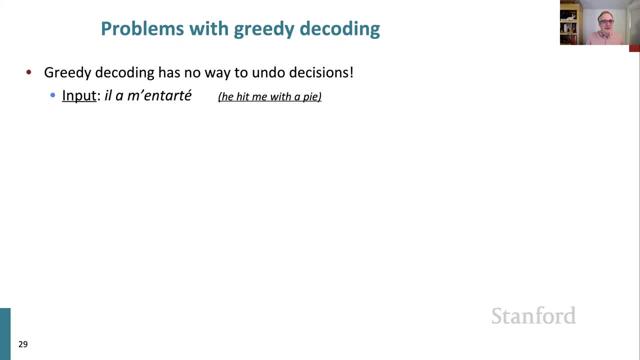 if these examples have been using this sentence about, he hit me with a pie going from translating from french to english. so you know, if you start off and you say okay, il, the first word in the translation should be he? um, that looks good. but then you um, and then you say, well, hit, i'll generate. 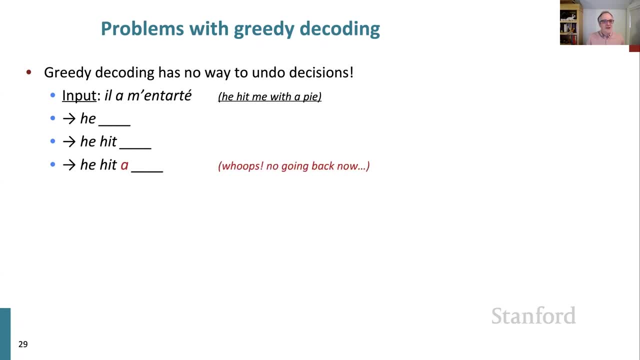 hit. um, then somehow the model thinks that the most likely next word is hit. after hitters are and. And there are lots of reasons it could think so, because after hit, most commonly there's a direct object noun. And you know, he hit a car, He hit a roadblock, Right. 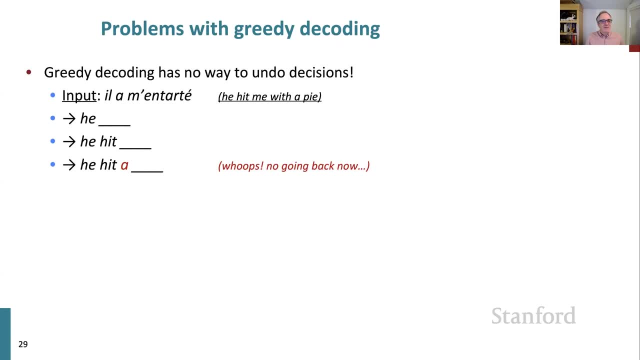 So that's pretty sounds, pretty likely. But you know, once you've generated it, there's no way to go backwards, And so you just have to keep on going from there and you may not be able to generate the translation you want. 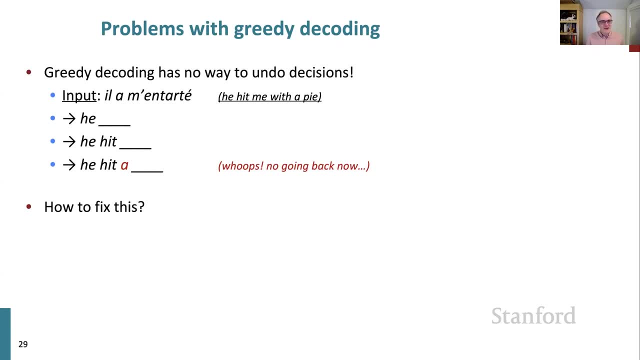 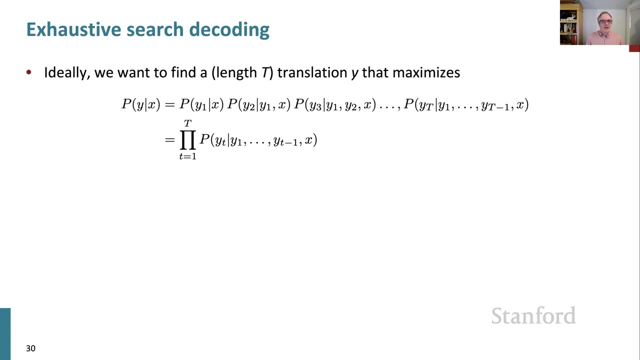 At best you can generate. he hit a pie, Oops, Something. So we'd like to be able to explore a bit more in generating our translations. And well, you know, what could we do? Well, you know, I sort of mentioned this before looking at the statistical MT models. 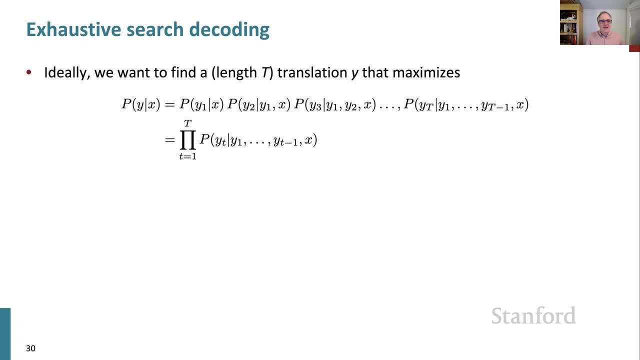 Overall, what we'd like to do is find translations, Translations that maximize the probability of Y given X, And at least if we know what the length of that translation is, we can do that as a product of generating a word at a time. 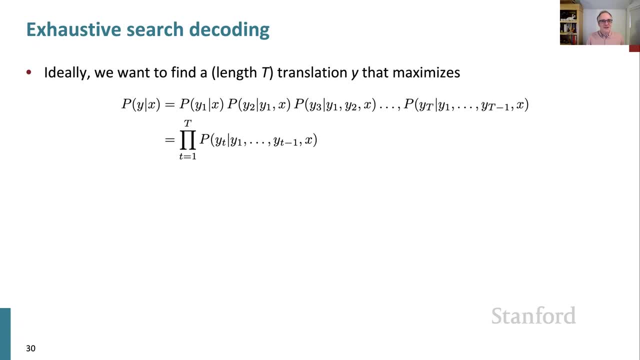 And so to have a full model, we also have to have a probability distribution over how long the translation length would be. So we could say: this is the model and let's you know, generate and score All All possible sequences Y using this model. 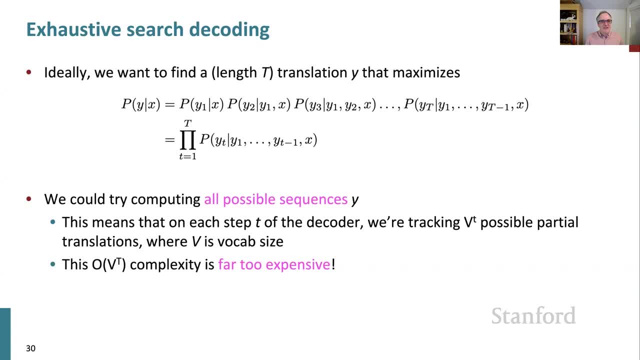 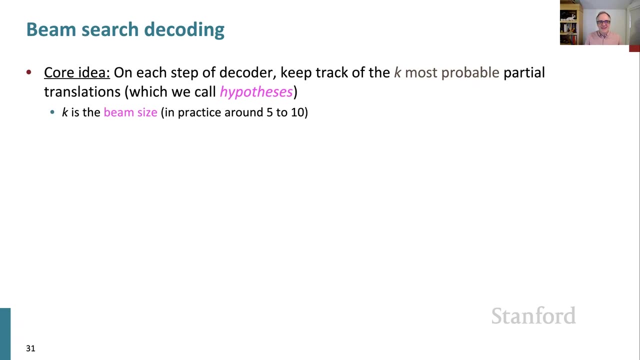 And that's where that then requires generating an exponential number of translations and is far, far too expensive. So, beyond greedy decoding, the most important method that is used- and you'll see lots of places- is something called beam search decoding, And so this isn't what neural well- any kind of machine- can do. 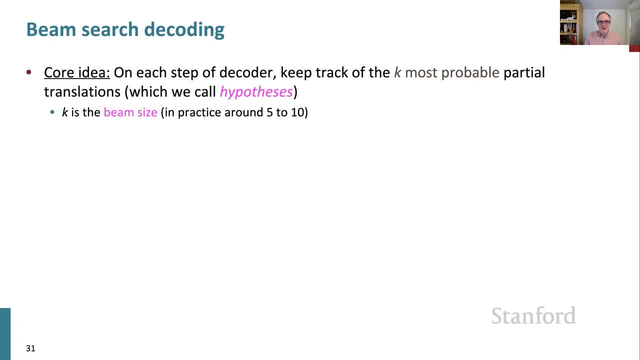 So this isn't what neural well, any kind of machine, can do. This is not just a single method. Again, machine translation is one place where it's commonly used, But this isn't a method that's specific to machine translation. You find lots of other places, including in all other kinds of sequence to sequence models. 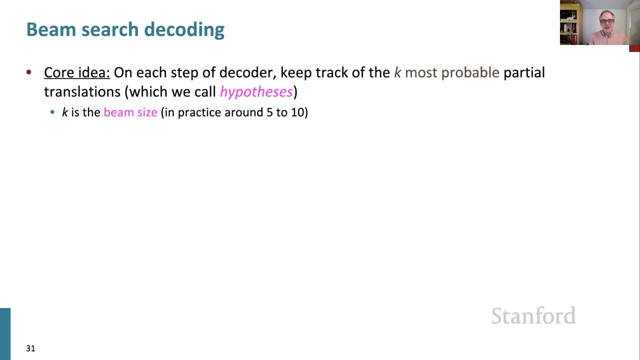 It's not the only other decoding method. When we got onto the language generation class, we'll see a couple more, But this is sort of the next one that you should know about. So beam search's idea is that you're going to keep some height of that code. 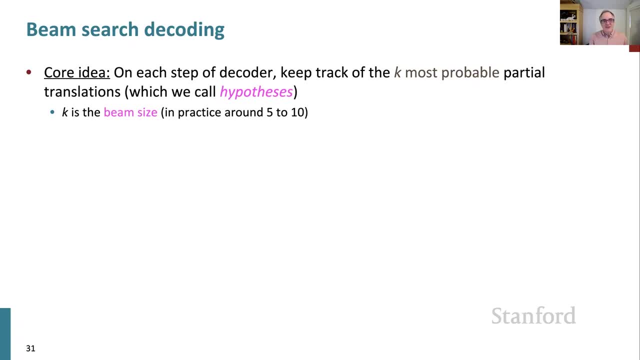 some hypotheses to make it more likely that you'll find a good generation while keeping the search tractable. So what we do is choose a beam size, And for neural MT the beam size is normally fairly small, something like 5 to 10.. 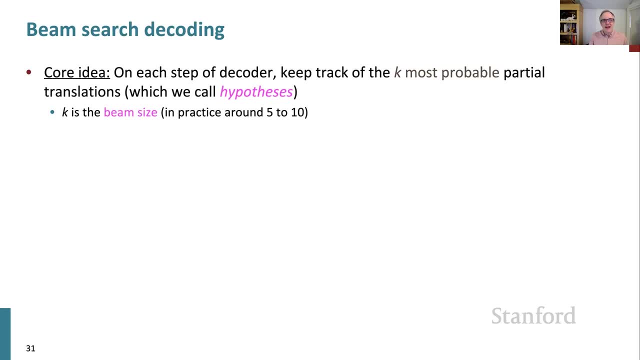 And at each step of the decoder we're going to keep track of the k most probable partial translations, so initial subsequences of what we're generating, which we call hypotheses. So a hypothesis, which is then the prefix of a translation, has a score which is this log probability up. 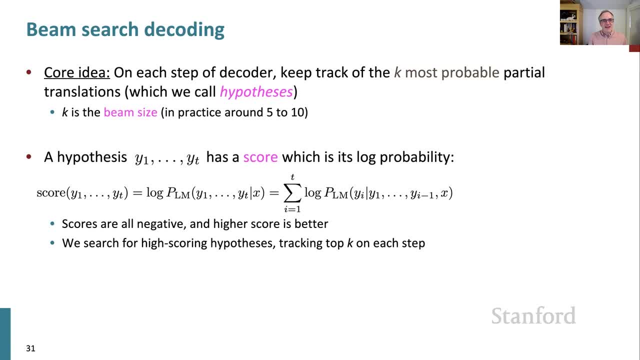 to what's been generated so far, So we can generate that in the typical way using our conditional language model. So, as written, all of the scores are negative, And so the least negative one, ie the highest probability one, is the best one. 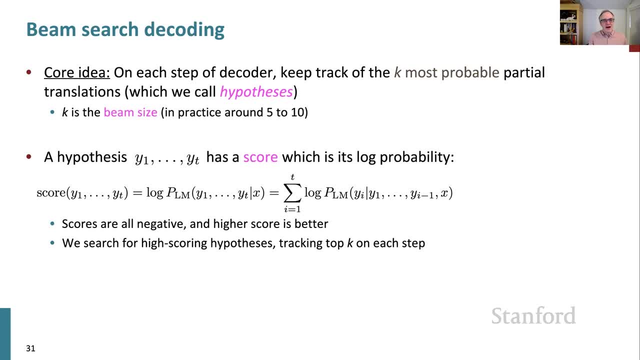 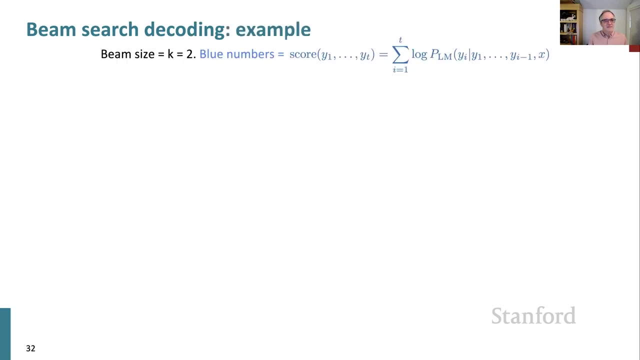 So if what we want to do is search for high probability hypotheses. So this is a heuristic method. It's not guaranteed to find the highest probability decoding, but at least it gives you more of a shot than simply doing greedy decoding. So let's go through an example to see how it works. 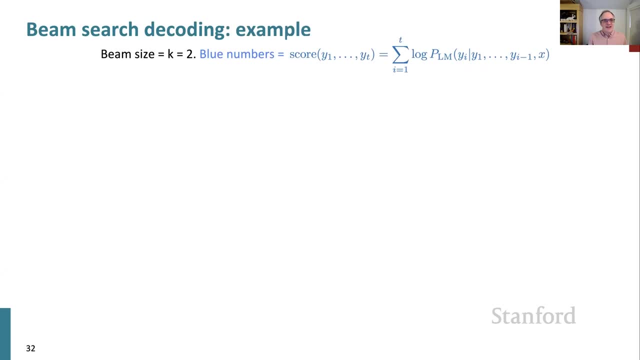 So, in this case, so I can fit it on a slide the size of our decoder. So let's go through an example to see how it works. So, in this case, so I can fit it on a slide the size of our. decoder. So let's go through an example to see how it works. So, in this case, so I can fit it on a slide the size of our decoder. So, in this case, so I can fit it on a slide the size of our. 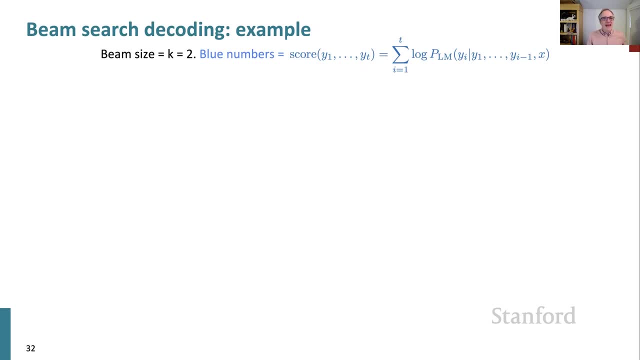 decoder. So normally our beam is just two- though normally it would actually be a bit bigger than that- And the blue numbers are the scores of the prefixes. So these are these log probabilities of a prefix. So we start off with our start symbol. 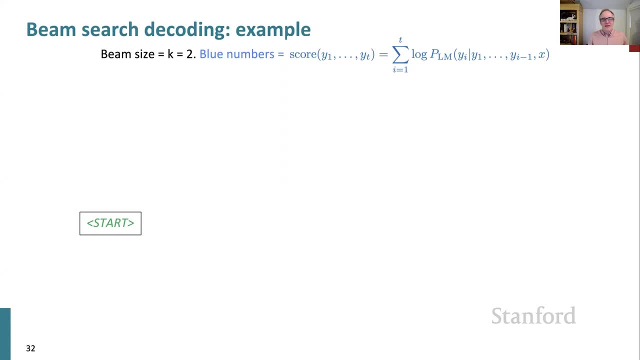 And we're going to say, OK, what are the two most likely words to generate first according to our language model? And so maybe the first two most likely words are he and I and they- i, and there are their log probabilities. 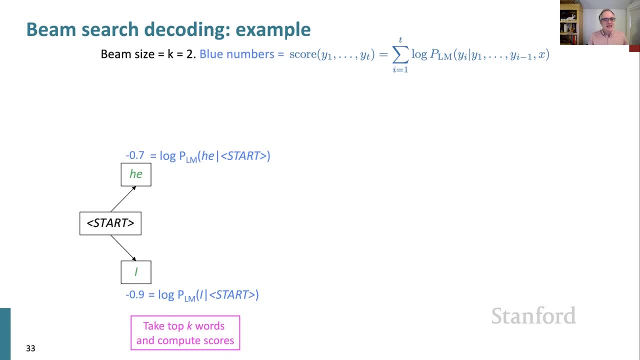 Then what we do next is, for each of these k hypotheses, we find what are likely words to follow them. In particular, we find what are the k most likely words to follow each of those, So we might generate: he hit, he struck, I was, I got. 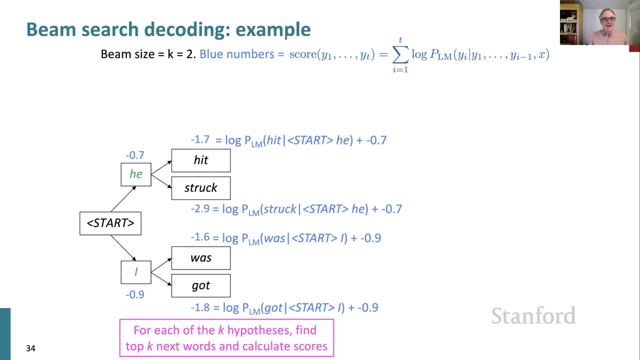 OK, so at this point it sort of looks like we're heading down what will turn into an exponential size tree structure again. But what we do now is we work out the scores of each of these partial hypotheses. So we have four partial hypotheses. he hit, he struck. 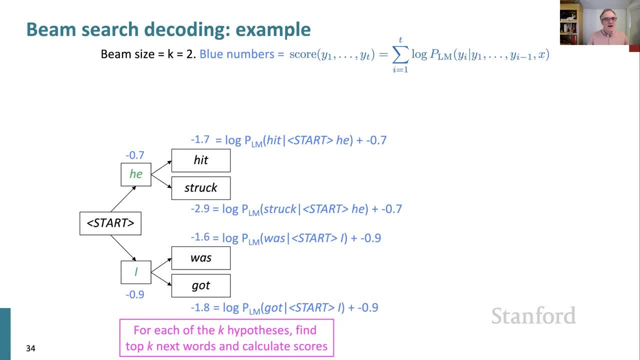 I was, I got. And we can do that by taking the previous score that we had for the partial hypothesis and adding on the log probability of generating the next word he hit. So this gives us scores for each hypothesis And then we can say which of those two partial hypotheses 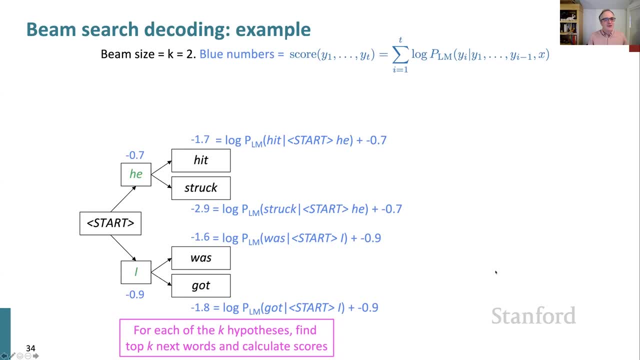 because our beam size k equals 2, have the highest score, And so they are. I was and he hit, So we keep those two and ignore the rest. And so then, for those two we're going to generate k hypotheses for the most likely following word. 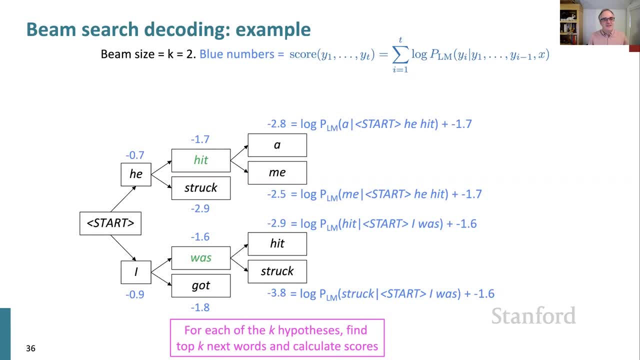 He hit a, he hit me, I was hit, I was struck, And again. now we want to find the k most likely hypotheses out of this full set, And so that's going to be. he struck me and I was- oh no. 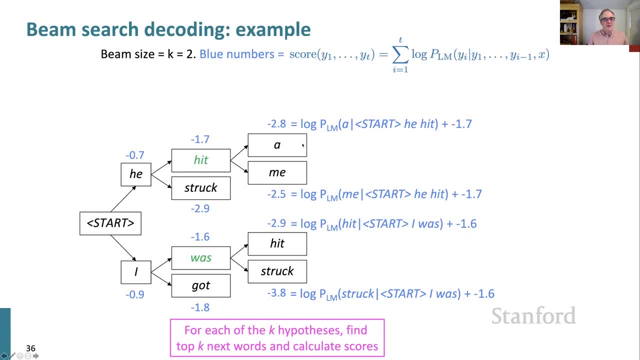 He struck me and he hit a. So we keep just those ones, And then for each of those we generate the k most likely. next words: tart pie with on. And then again we filter back down to size k by saying: OK. 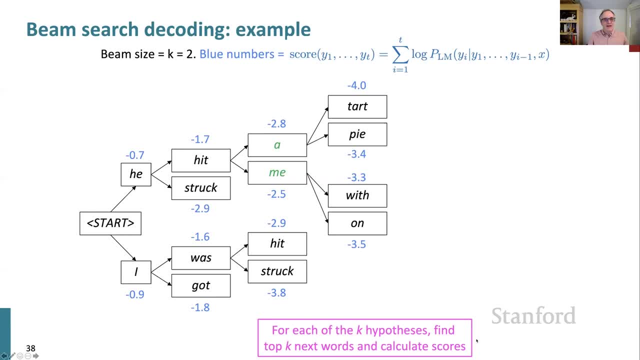 the two most likely things here are pie or with. So we continue working on those. generate things, find the two most likely. generate things, find the two most likely. And at this point we would generate end of string and say, OK, we've got a complete hypothesis. 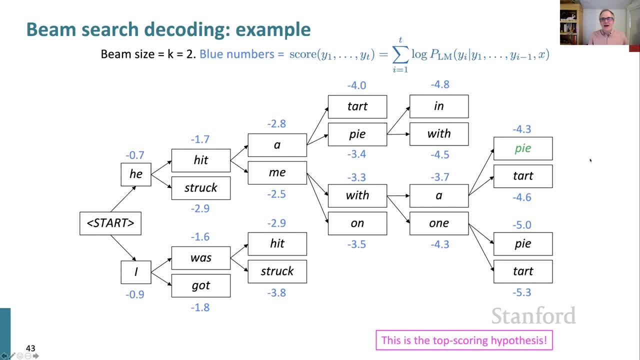 He struck me with a pie, And we could then trace back through the tree to obtain the full hypothesis for this sentence. So that's most of the algorithm. There's one more detail, And that's the end of string, which is the stopping criterion. 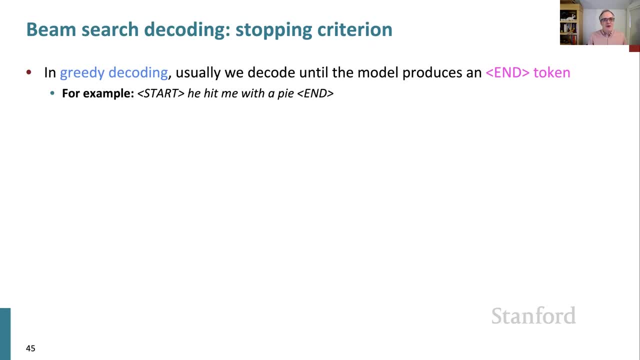 So in greedy decoding we usually decode until the model produces an end token, And when it produces the end token we say we are done. In beam search decoding different hypotheses may produce end tokens on different time steps, And so we don't want to stop as soon as one path through the search tree. 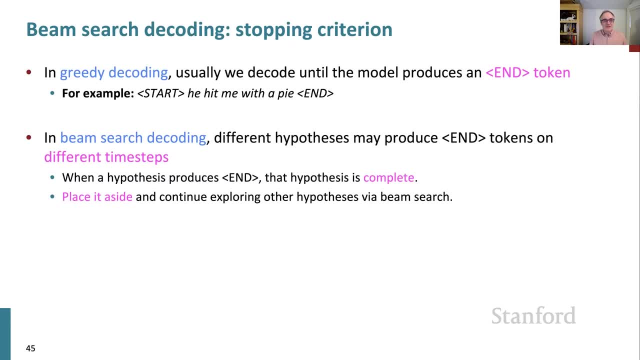 generated end, because it could turn out that there's a different path through the search tree which will still prove to be better. So what we do is sort of put it aside as a complete hypothesis and continue exploring other hypotheses via our beam search. 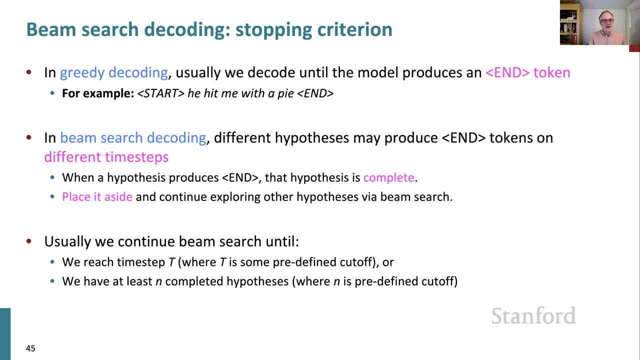 And so usually we will then either stop when we've hit a cutoff length or when we've completed end, And then we'll look through the hypotheses that we've completed and say which is the best one of those And that's the one we'll use. 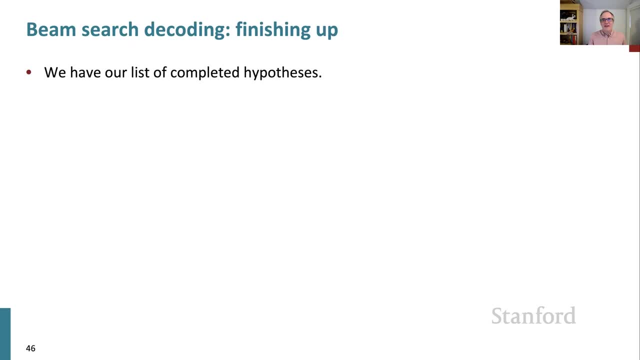 So at that point, we have our list of completed hypotheses And we want to select the top one with the highest score. Well, that's exactly what we've been computing. Each one has a list of completed hypotheses And we want to use that list of completed hypotheses. 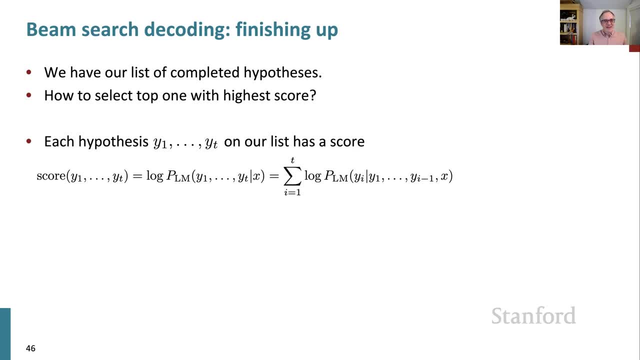 to find the most accurate probability that we've worked out. But it turns out that we might not want to use that just so naively, because there turns out to be a kind of a systematic problem, which is not as a theorem but in general longer hypotheses. 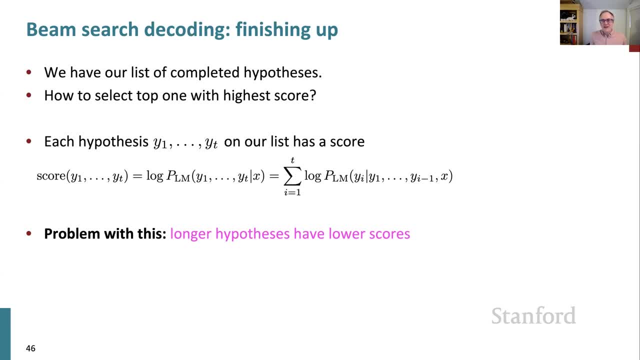 have lower scores. So if you think about this as probabilities of successively generating each word And if you think about this as probability of successively generating each word, then you're going to have a higher chance of generating the next word probability, And commonly those might be 10 to the minus 3,, 10 to the minus 2.. 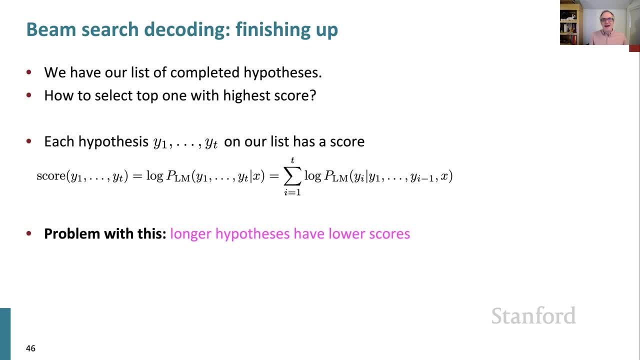 So, just from the length of the sentence, your probabilities are getting much lower the longer that they go on, in a way that appears to be unfair, Since although in some sense extremely long sentences aren't as likely as short ones, they're not less likely by that much. 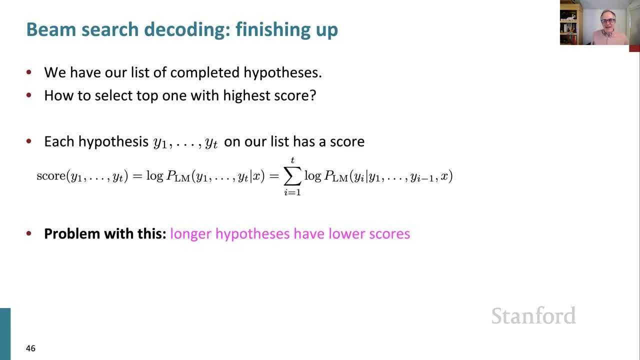 For example, in a newspaper, the median length of sentences is over 20.. So you wouldn't want to be having a decoding model when translating news articles that sort of says: oh, just generate two-word sentences. They're just way higher probability. 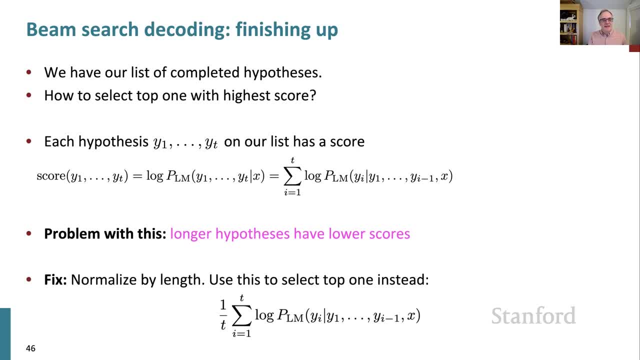 according to my language model. So the commonest way of dealing with that is that we normalize by length. So if we're working in log probabilities, that means again dividing through by the length of the sentence And then you have a per-word log probability score. 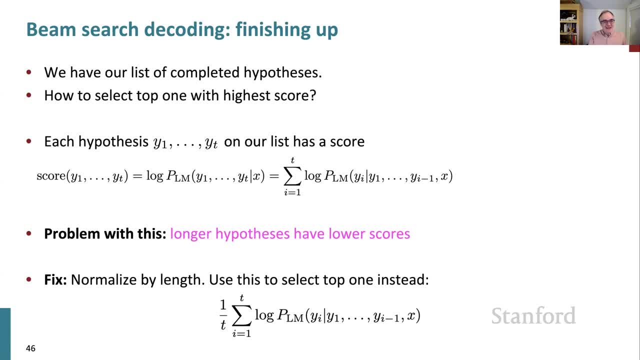 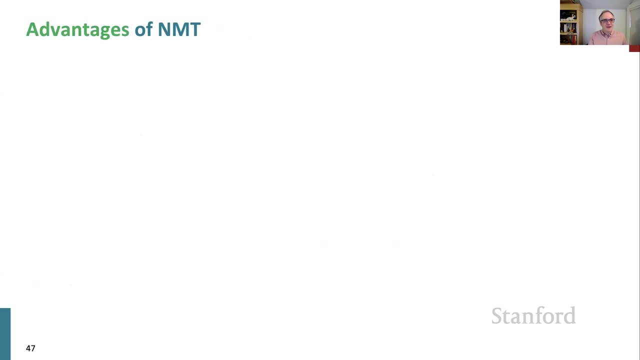 And you can argue that this isn't quite right in some theoretical sense, But in practice it works pretty well And it's very commonly used. Neural translation has proven to be much, much better. I'll show you a couple of statistics about that in a moment. 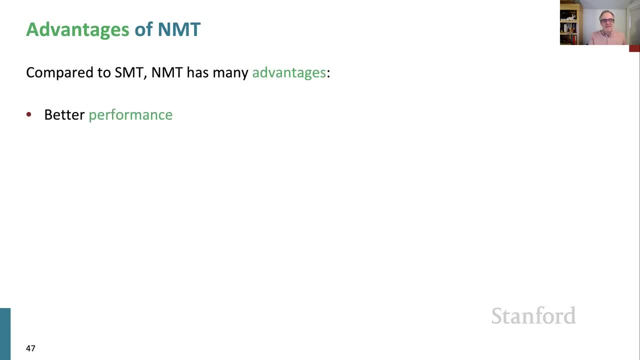 It has many advantages: It gives better performance, The translations are better. In particular, they're more fluent, because neural language models produce much more fluent sentences. But also they much better use context because neural language models, including conditional neural language models. 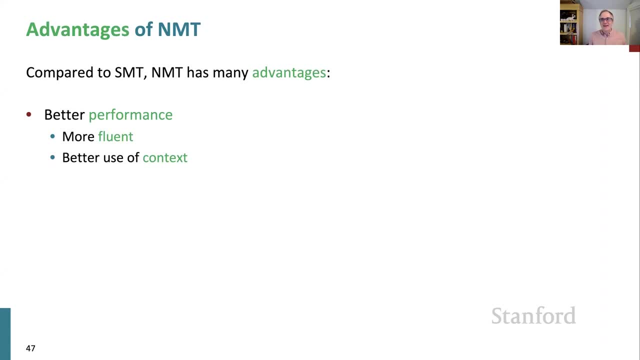 give us a very good way of conditioning on a lot of context. in particular, we can just run a long encoder and condition on the previous sentence, Or we can translate words well in context by making use of neural context. Neural models better understand phrase similarities and phrases. 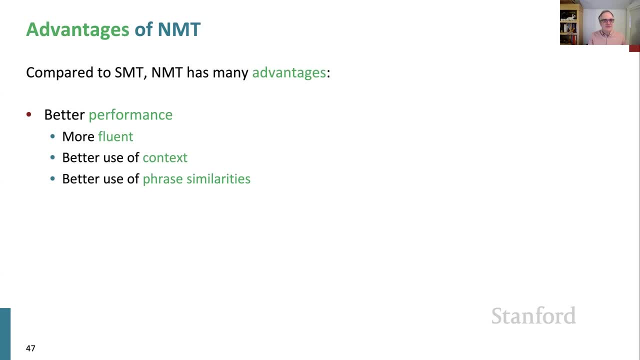 that mean approximately the same thing. And then the technique of optimizing all parameters of the model, end-to-end, in a single line. in a single line, and all methods and everything else we think of. the method is really called the neural network, And that's a direct reflection. 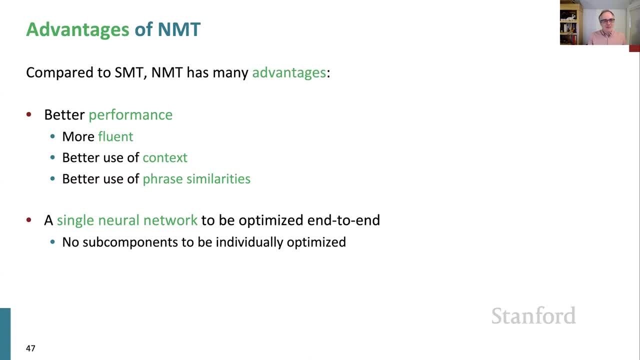 of what it's supposed to look like And what this new network looks like has a lot of risks to it And the process has probably been very popular among the dorsal networks and the neural networks that are now ehaving extremely valuable effects for the neural networks that we're building. 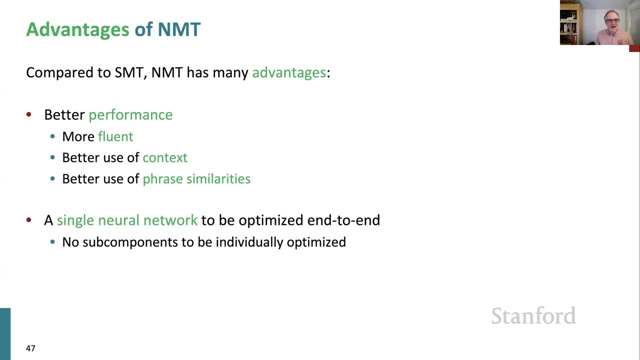 and really use in real time as well. But the last one I'll mention: it's again very important: end-to-end. that will give you much better performance than component-wise systems. We'll come back to the costs of that later in the course. 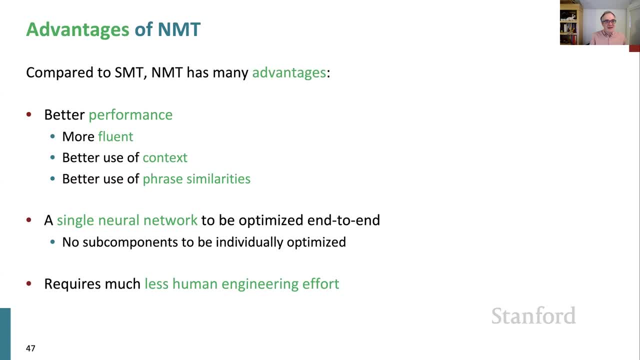 The models are also actually great in other ways. They actually require much less human effort to build. There's no feature engineering. There's, in general, no language-specific components. You're using the same method for all language pairs. Of course, it's rare for things to be perfect in every way. 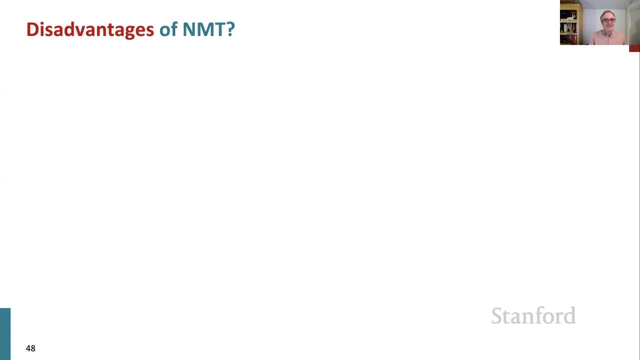 So neural machine translation systems also have some disadvantages compared to the older statistical machine translation systems. They're less interpretable. It's harder to see why they're doing what they're doing where before you could actually look at phrase tables and they were useful. 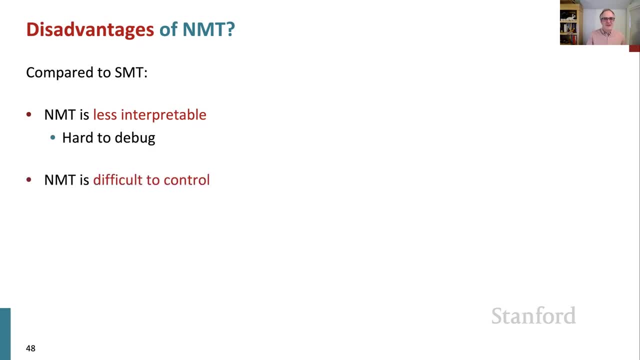 So they're hard to debug. They also tend to be sort of difficult to control. So, Compared to anything like writing rules, you can't really give much specification if you'd like to say, oh, I'd like my translations to be more casual, or something like that. 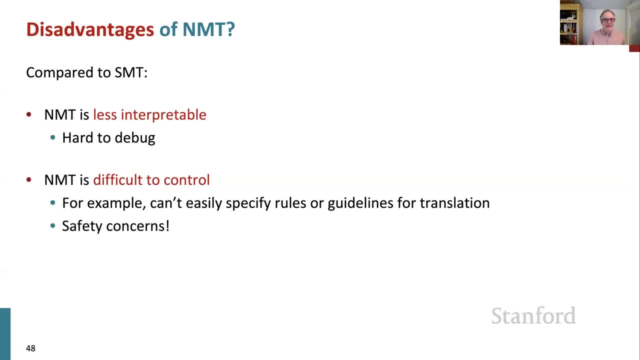 It's hard to know what they'll generate. So there are various safety concerns. I'll show a few examples of that in just a minute, But first, before doing that quickly, how do we evaluate machine translation? The best way to evaluate machine translation. 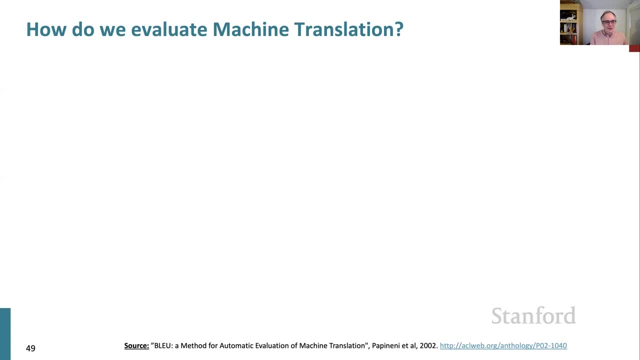 is to show a human being who's fluent in the source and target languages, the sentences and get them to give judgment on how good a translation it is. But that's expensive to do and might not even be possible if you don't have the right human beings around. 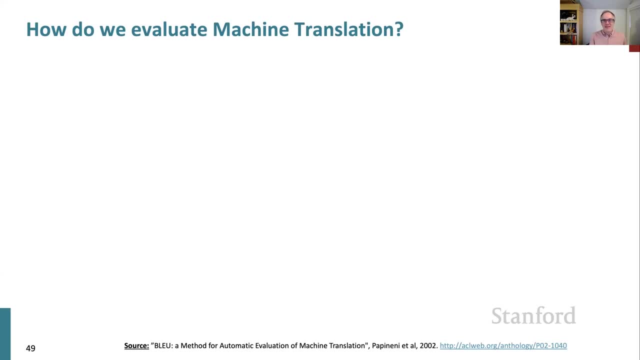 So a lot of work was put into finding automatic methods of scoring translation, And the most famous method of doing that is what's called BLEU. And the way you do BLEU is you have a human translation, or several human translations of the source sentence. 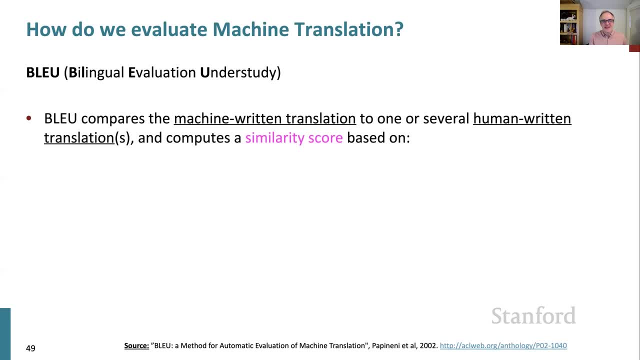 And you're comparing a machine-generated translation to those pre-given human written translations And you score them for similarity by calculating n-grams of the source sentence And you're going to get a result, And then you're going to calculate n-gram precision. 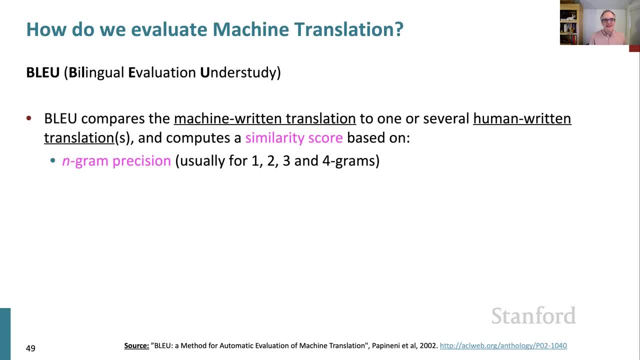 a words that overlap between the computer and human written translation, bigrams, trigrams and fourgrams, and then working out geometric average between overlaps of n-grams. Plus there's a penalty to short system translations. So BLEU has proven to be a really useful measure. 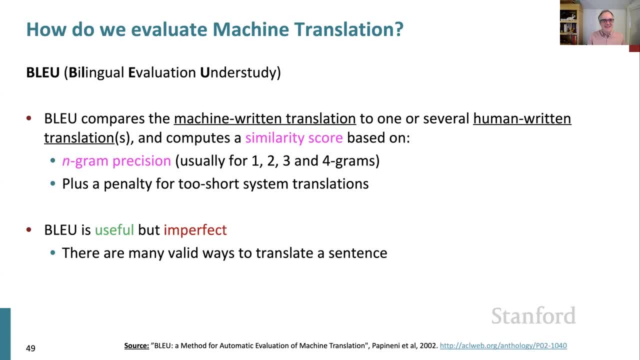 But it's an imperfect measure ways to translate a sentence, and so there's some luck as to whether the human written translations you have happen to correspond to which to what might be a good translation from the system. There's more to say about the details of blue and how it's implemented, but 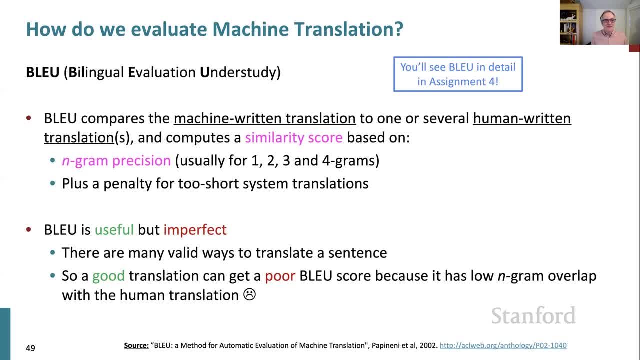 you're going to see all of that doing. assignment four, because you will be building neural machine translation systems and evaluating with them with the blue algorithm, and there are full details about blue in the assignment handout. At the end of the day, blue gives the score between zero and 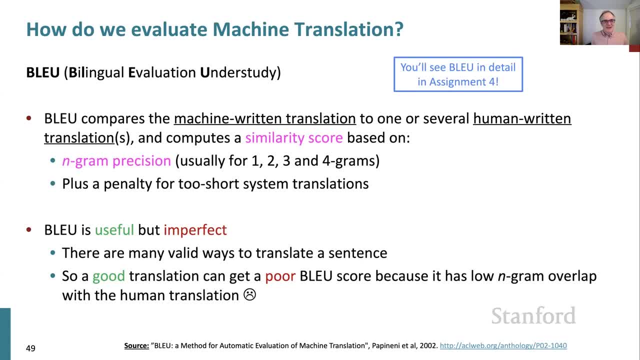 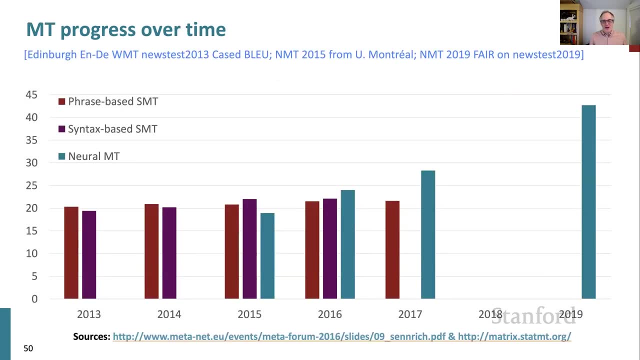 a hundred where your score is: a hundred if you're exactly producing one of the human written translations and zero if you're. there's not even a single unigram that overlaps between the two. With that rather brief intro, I wanted to show you sort of what happened in machine translation. 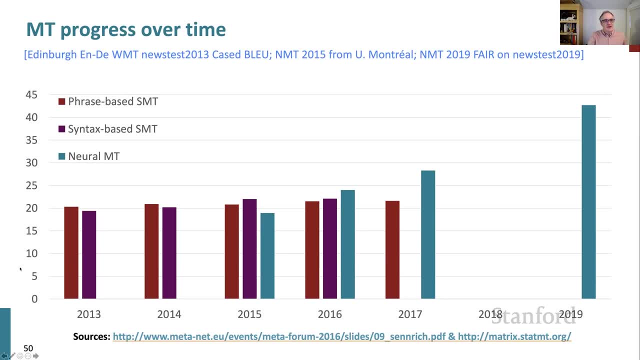 So machine translation with statistical models, phrase-based statistical machine translation that I showed at the beginning of the class- had been going on since the mid-2000s decade and it had produced sort of semi-good results of the kind that are in Google Translate in those days, but by 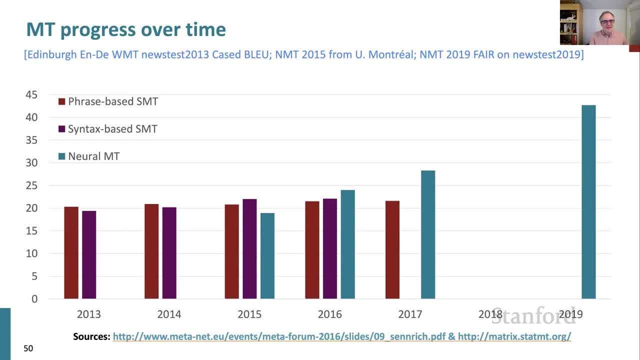 the time we entered the 2010s, basically progress and statistical machine translation had stalled and you are getting barely any increase over time, and most of the increase and time you were getting over time was simply because you're training your models on more data in those years around the early 2010s. 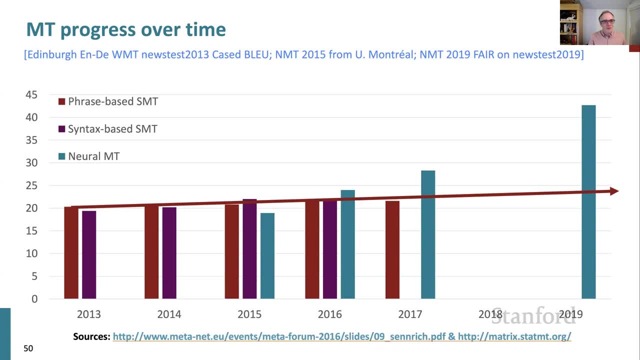 Um, The b? b hope that most people had. someone asked: what is the y-axis here? this y-axis is this blue score that I told you about on the previous slide In the early 2010s, the big hope that most people in. 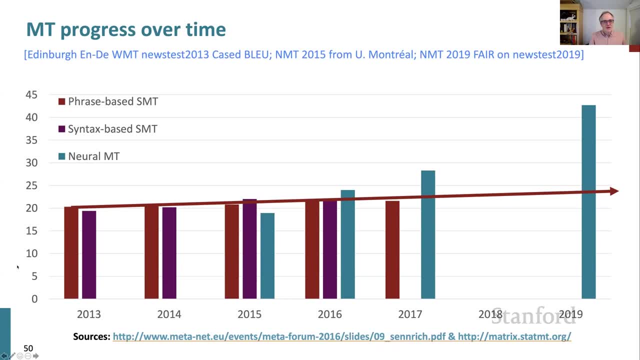 the machine translation field had was well. if we built a more complex kind of machine translation model that knows about the syntactic structure of languages, that makes use of tools like dependency parsers, we'll be able to build much better translations. And so those are the purple systems. 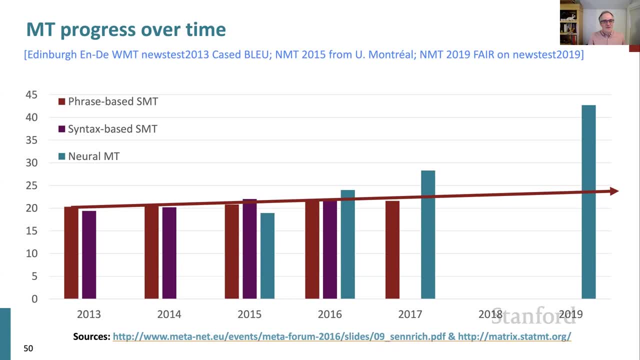 here, which I haven't described at all, But it's sort of. as the years went by, it was pretty obvious that that barely seemed to help. And so then in the mid-2010s- so in 2014 was the first modern attempt to build a neural network for machine translation. And then in the mid-2010s, 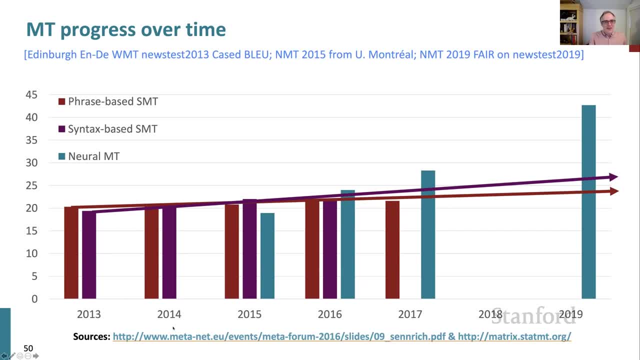 we started to build a new model for machine translation as an encoder-decoder model And by the time it was sort of evaluated in bake-offs in 2015,. it wasn't as good as what had been built up over the preceding decade, but it was already getting pretty good. But what was? 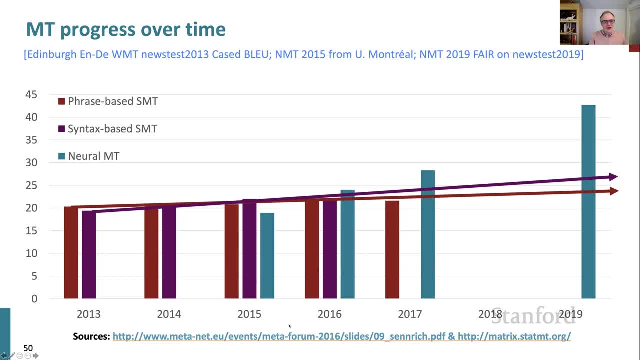 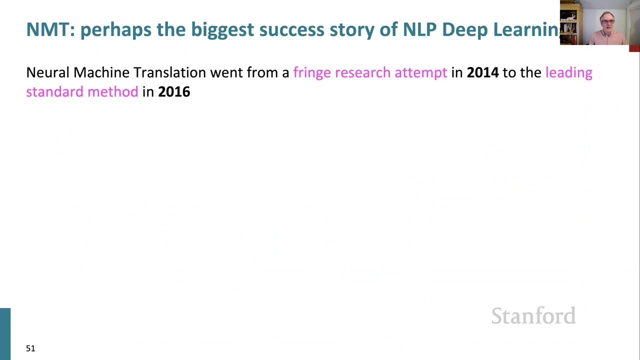 found was that these neural models just really opened up a whole new pathway to start building much, much better machine translation systems. And since then things have just sort of taken off and the neural machine translation systems are getting much better and far better than anything we had preceding that. So for you know, at least the early part of 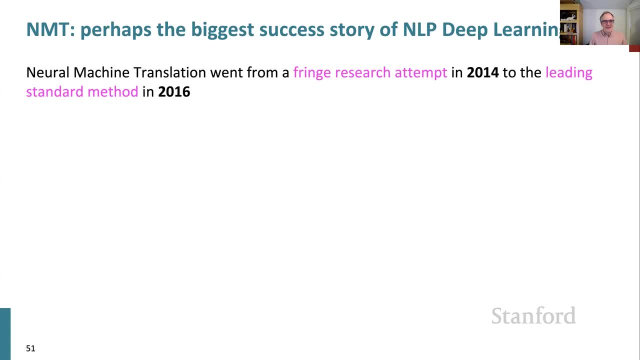 application of deep learning and natural language processing. neural machine translation was the huge big success story In the last few years when we've had models like GPT-2 and GPT-3 and other huge neural models like BERT. improving web search, you know it's a bit more complex. 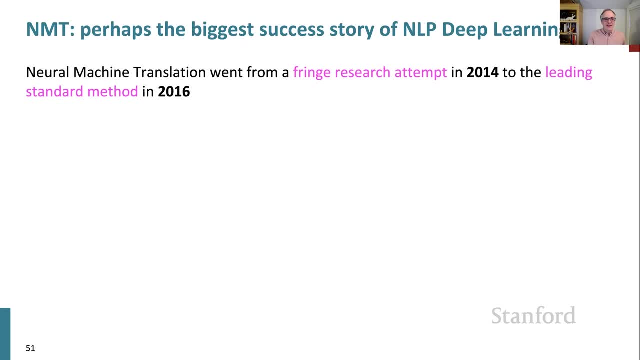 But this was the first area where there was a neural network which was hugely better than what had preceded and was actually solving a practical problem that lots of people in the world need, And it was stunning with the speed at which success was achieved. So 2014 were the first what I call here fringe research attempts to build a neural machine. 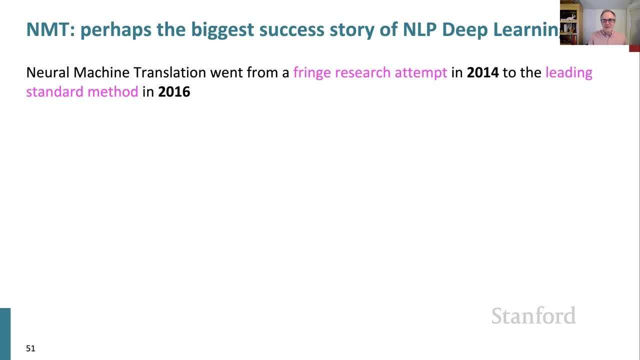 translation system, meaning that three or four people who were working on neural network models thought: oh, why don't we see if we can use one of these to translate, learn to translate sensors, where they weren't really people with a background in machine translation at all. 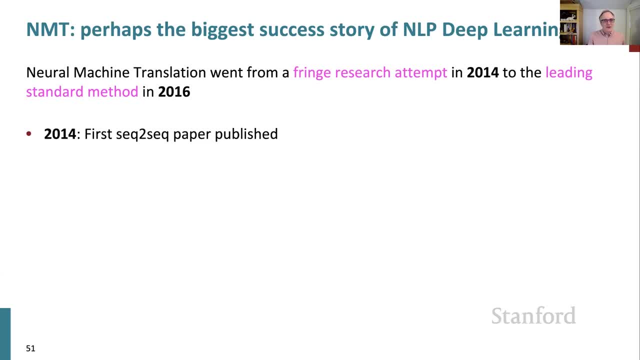 But success was achieved so quickly that within two years' time, Google had switched to using neural machine translation for most languages, And by a couple of years later after that, essentially anybody who does machine translation is now deploying live neural machine translation systems and getting much, much better results. 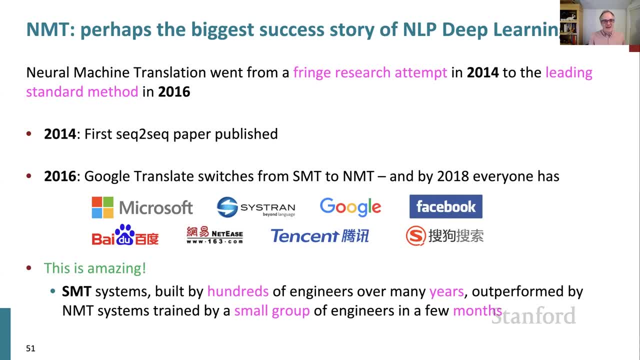 So that was sort of just an amazing technological transition that for the preceding decade the big statistical machine translation systems, like the previous generation of Google Translate, had literally been built up by hundreds of engineers over years But a comparatively small group of people who were using Google Translate 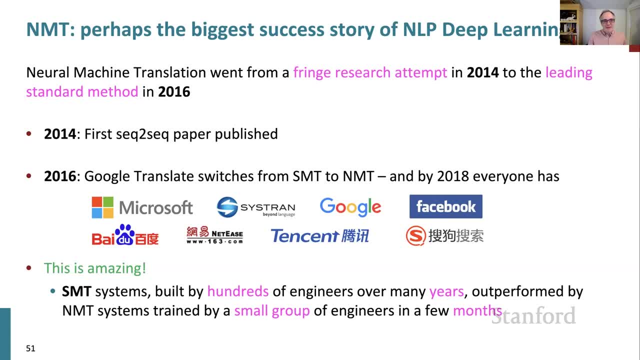 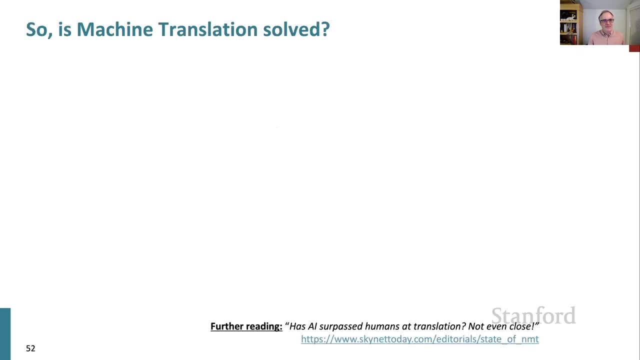 and deep learning people. in a few months, with a small amount of code- and hopefully you'll even get a sense of this doing assignment four, were able to build neural machine translation systems that proved to work much better. Does that mean that machine translation is solved? 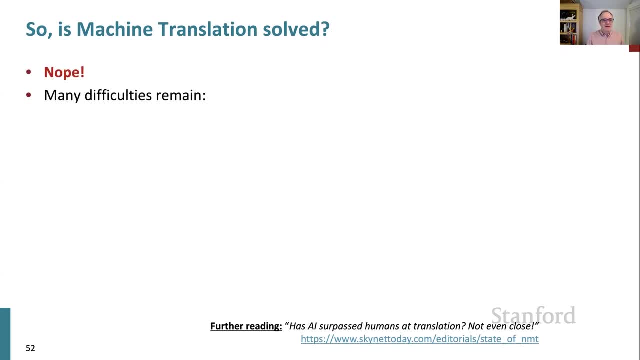 No, There are still lots of difficulties which people continue to work on very actively And you can see more about it in the slideshow. But there are lots of problems with out-of-vocabulary words. There are domain mismatches between the training and test data. 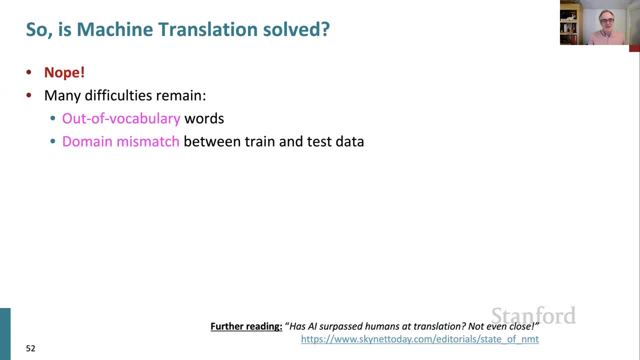 So it might be trained mainly on newswire data, but you want to translate people's Facebook messages. There are still problems with maintaining context over longer text. We'd like to translate languages for which we don't have much data, And so these methods. 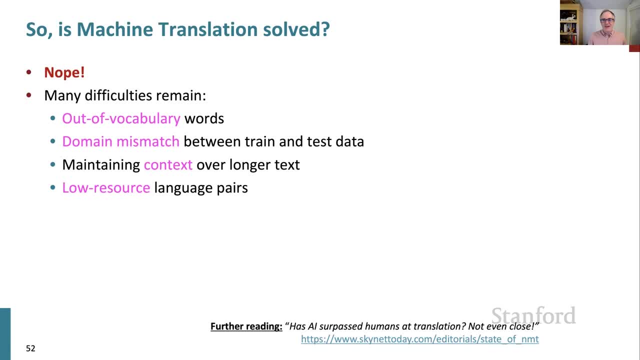 we're going to have to work by far the best when we have huge amounts of parallel data. Even our best multi-layer LSTMs aren't that great at capturing sentence meaning. There are particular problems, such as interpreting what pronouns refer to or in languages like Chinese. 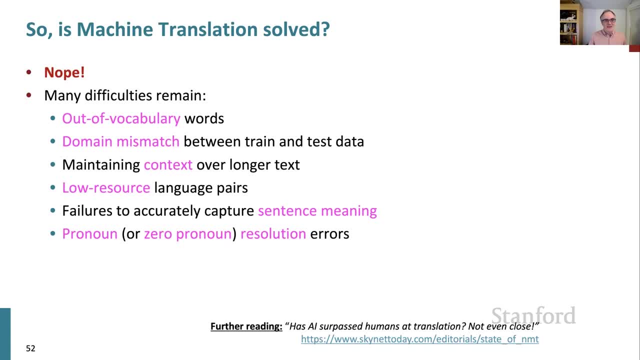 or Japanese, where there's often no pronoun present, but there is an implied reference to some person working out how to translate that. For languages that have lots of inflectional forms of nouns, verbs and adjectives, these systems often get them wrong. 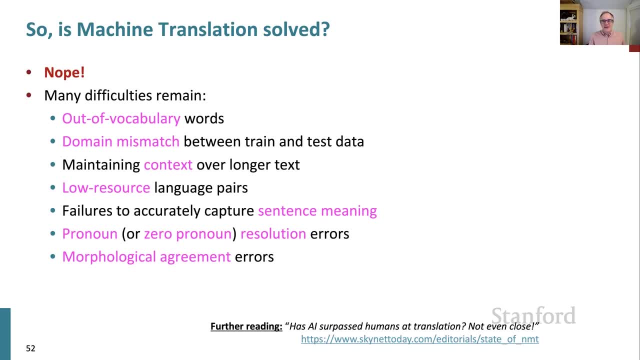 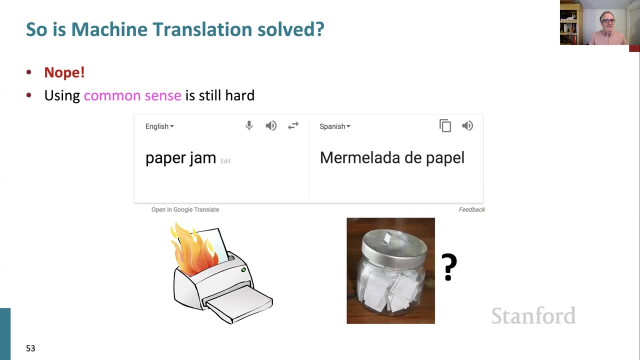 So there's still tons of stuff to do, So here's just sort of quick, funny examples of the kind of things that go wrong, right? So if you ask to translate paper jam, Google Translate is deciding that this is a kind of jam. 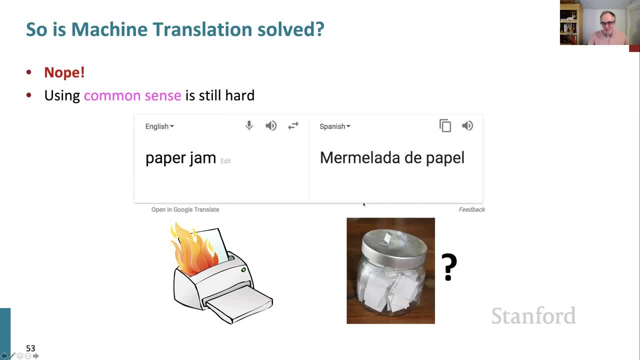 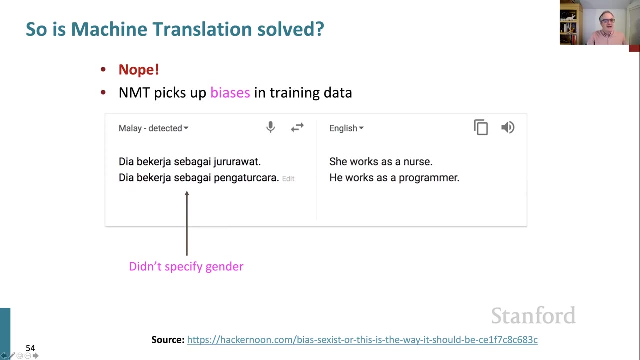 just like there's raspberry jam And strawberry jam, and so this becomes a jam of paper. There are problems of agreement and choice, So if you have many languages, don't distinguish gender, And so the sentences are neutral between things are masculine or feminine. 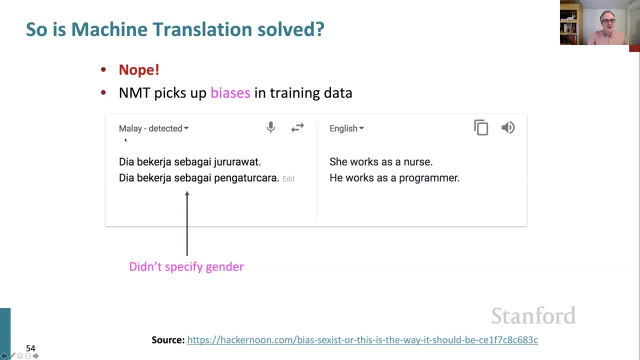 So Malay or Turkish are two well-known languages of that sort. But what happens when that gets translated into English by Google Translate is that the English language model just kicks in and applies stereotypical biases, And so these gender neutral sentences get translated into: she works as a nurse, he works as a programmer. 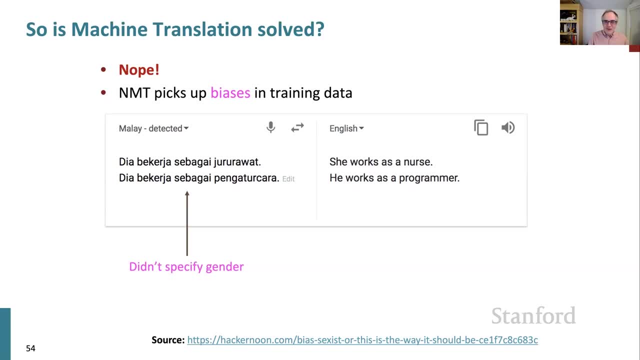 So if you wanna help solve this problem, you- all of you- can help by using singular they in all contexts when you're putting material online right, And that could then change the distribution of what's generated. But people also work on modeling improvements to try and avoid this. 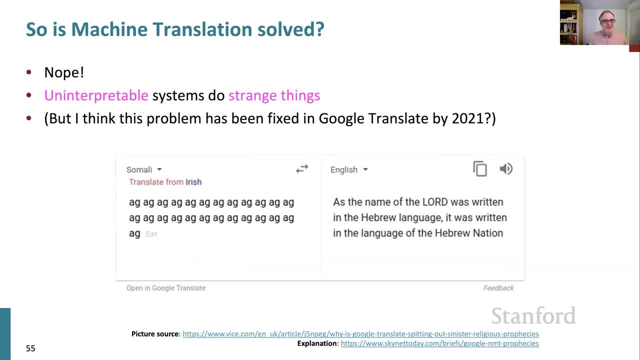 Here's one more example. that's kind of funny. People noticed a couple of years ago that if you choose one of the rarer languages that Google will translate, such as Somali, and you just write in some rubbish like ag, ag, ag, ag. 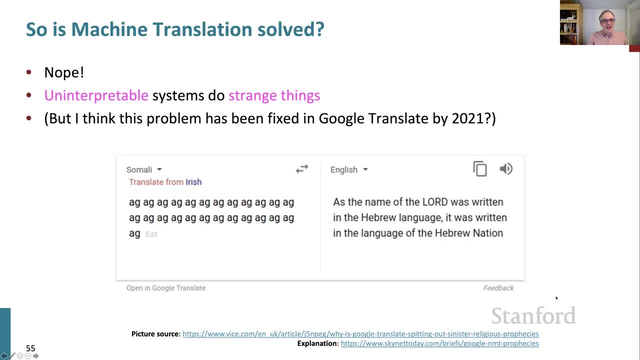 frequently, it would produce out of nowhere prophetic and biblical texts, as the name of the Lord was written in the Hebrew language. It was written in the language of the Hebrew nation, which makes no sense at all. We're about to see a bit more about why this happens. 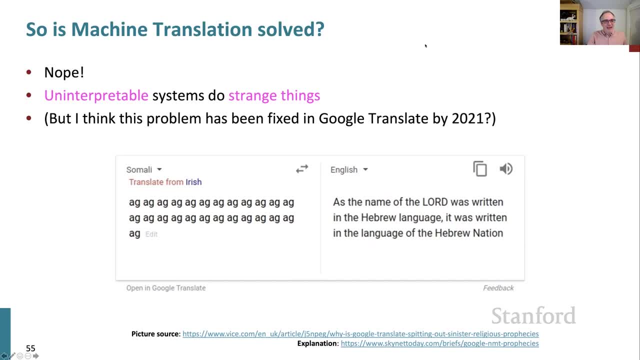 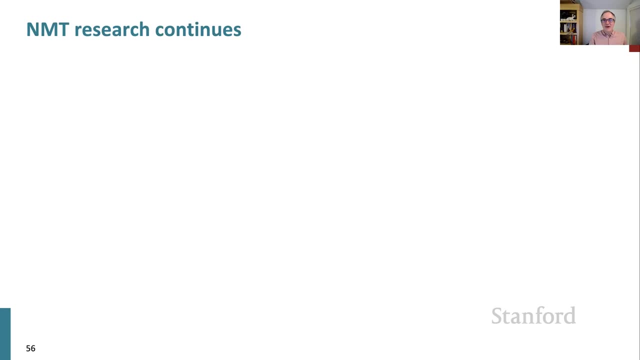 but that was sort of a bit worrying. As far as I can see, this problem is now fixed in 2021.. I couldn't actually get Google Translate to generate examples like this anymore, But so there are lots of ways to keep on doing research. 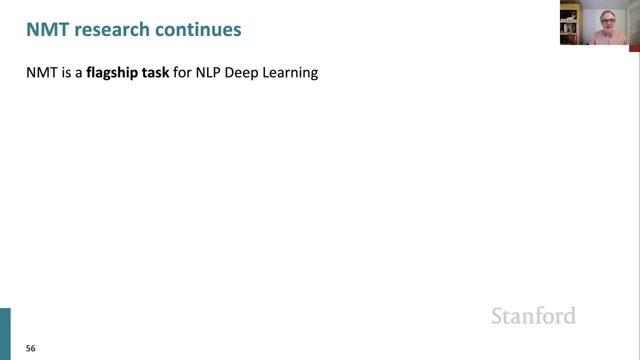 NMT is certainly a flagship task for NLP and deep learning And it was a place where many of the innovations of deep learning, NLP, were pioneered And people continue to work hard on it. People have found many, many improvements, And actually for the last bit of the class in a minute. 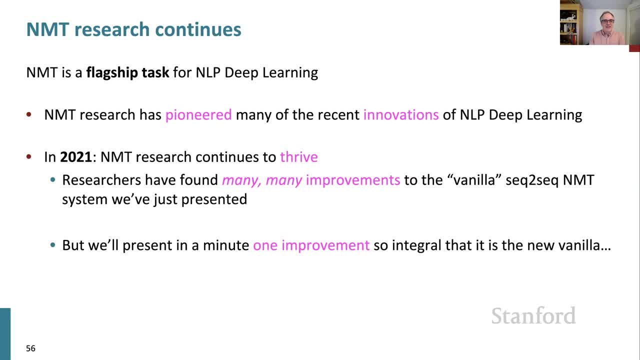 I'm going to present one huge improvement which is so important that it's really come to dominate the whole of the recent field of neural networks for NLP, And that's the idea of attention. But before I get on to attention, I want to spend. 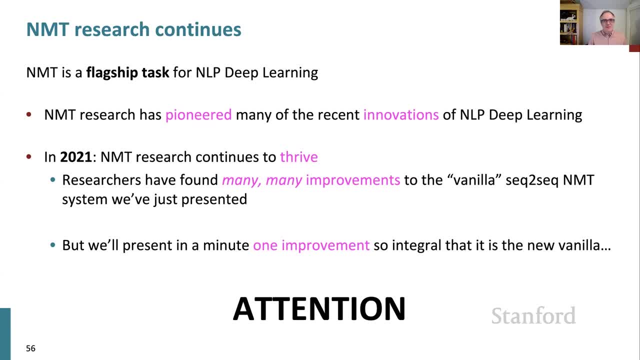 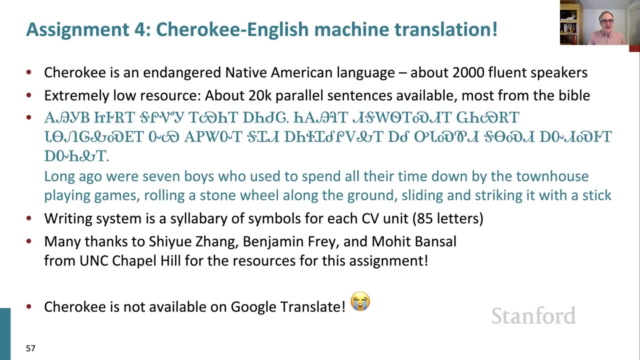 Three minutes on our assignment four. So for assignment four this year we've got a new version of the assignment which we hope will be interesting, but it's also a real challenge. So for assignment four this year we've decided to do Cherokee English machine translation. 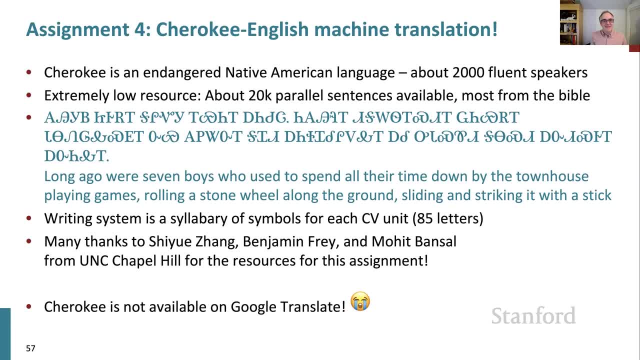 So Cherokee is an endangered Native American language. It has about 2,000 fluent speakers. It's an extremely low-resource language, So it's just. there isn't much written Cherokee data available period And particularly there's not a lot of parallel sentences between Cherokee and English. 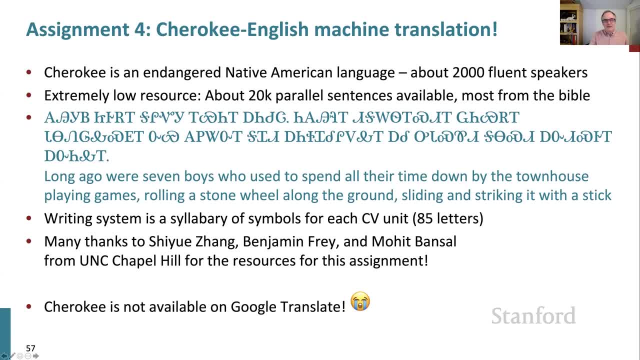 And here's the answer to Google's freaky prophetic translations For languages for which there isn't much parallel data available. commonly, the biggest problem is that there isn't a lot of parallel data available for any of the three languages, And so the biggest place where you can get parallel data- 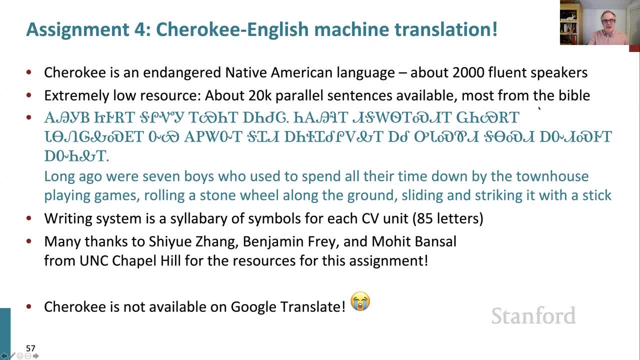 is from Bible translations, So you can have your own personal choice, wherever it is over the map, as to where you stand with respect to religion. But the fact of the matter is, if you work on Indigenous languages, what you very, very quickly? 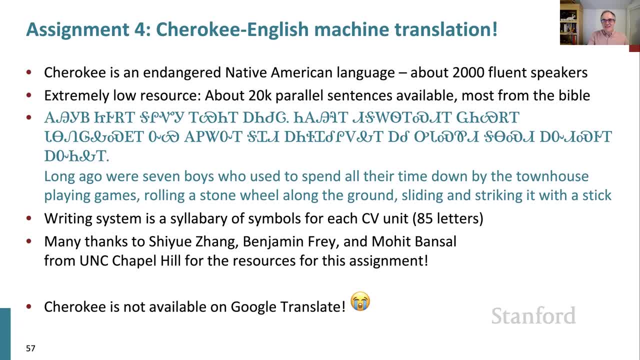 find is that a lot of the work that's done on collecting data and the material that is available in written form for many Indigenous languages is Bible translations. Yeah, OK, So this is what Cherokee looks like, And so you can see that the writing system has. 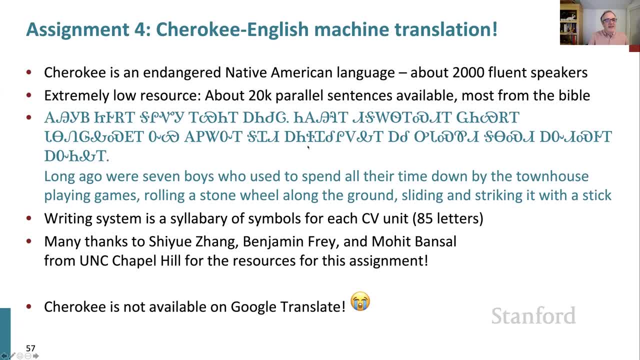 a mixture of things that look like English letters and then all sorts of letters that don't, And so here's the initial bit of a story long ago about boys who used to spend all their time down by the townhouse, So this is a piece of parallel data that we can learn from. 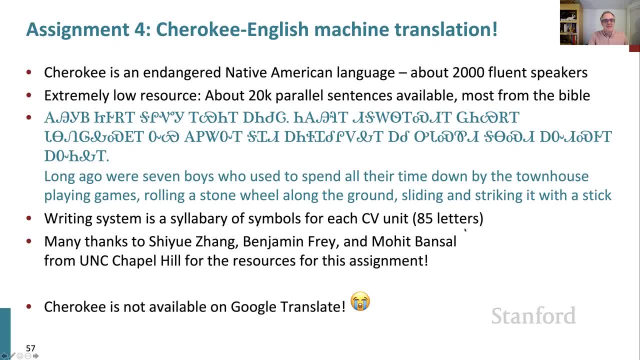 So the Cherokee writing system has 85 letters, And the reason why it has so many letters is that each of these letters actually represents a syllable. So many languages of the world have strict consonant-vowel syllable structures, So you have words like or something. 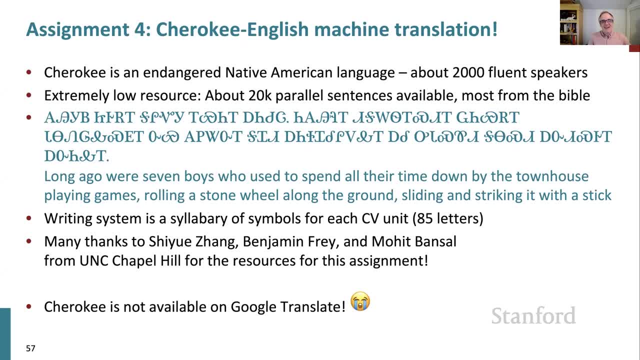 like that, or Cherokee right, And another language like that's Hawaiian, And so each of the letters represents a combination of a consonant and a vowel, And that's the set of those. You then get 17 by 5, gives you 85 letters. 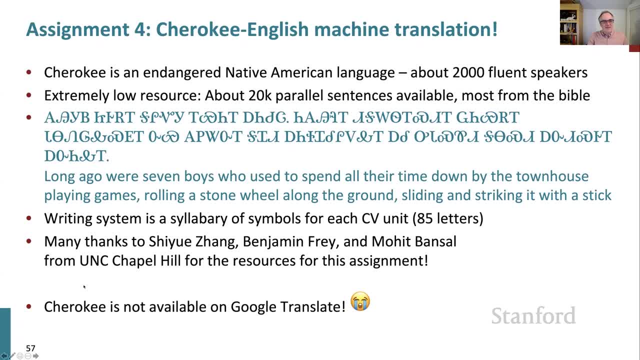 Yeah, So being able to do this assignment. big thanks to people from University of North Carolina, Chapel Hill, who've provided the resources we're using for this assignment. Although you can do quite a lot of languages on Google Translate, Cherokee is not a language. 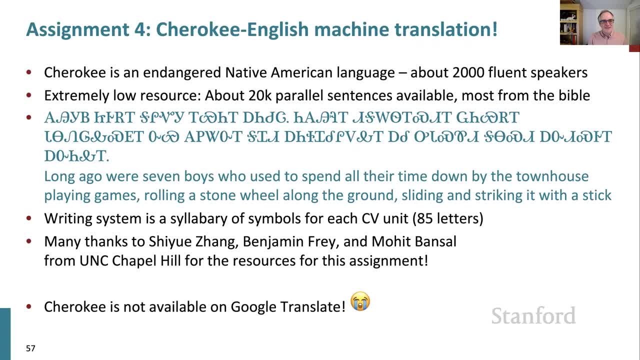 that Google offers on Google Translate. So we can see how far we can get. But we have to be modest in our expectations because it's hard to build a very good MT system with only a fairly limited amount of data. So we'll see how far we can get. 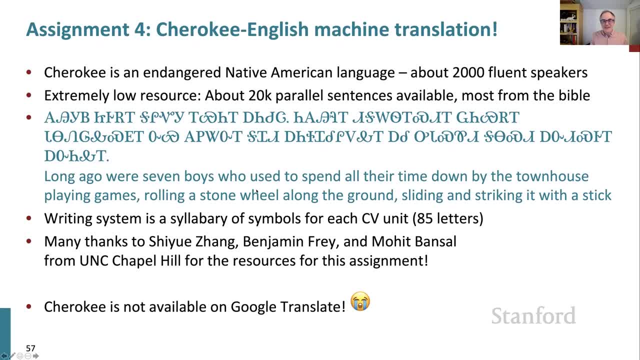 There is a flip side, which is for you students doing the assignment. The advantage of having not too much data is that your models will train relatively quickly. So we'll actually have less troubles than we did last year with people's models taking hours to train. 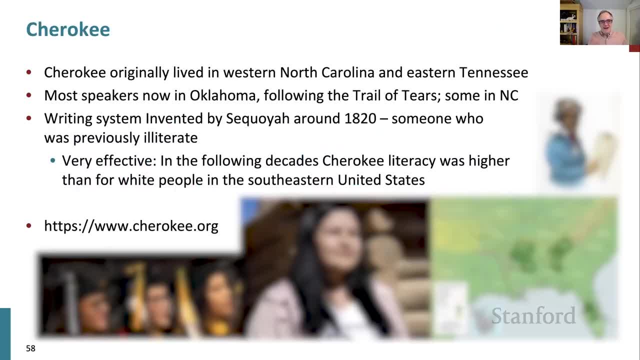 as the assignment deadline closed. in There's a couple more words about Cherokee, so we have some idea of what we're talking about. So the Cherokee originally lived lived in western North Carolina and eastern Tennessee. They then sort of got shunted southwest from that. 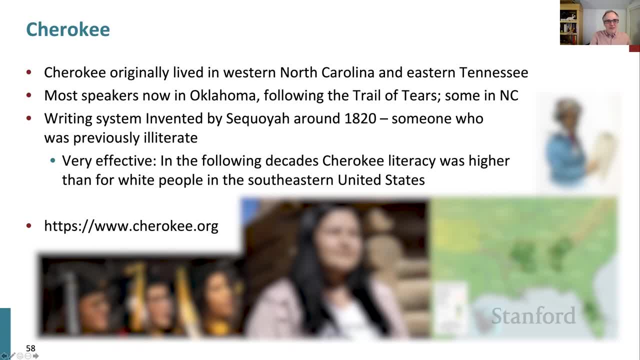 And then, in particular, for those of you who went to American high schools and paid attention, you might remember discussion of the Trail of Tears, when a lot of the Native Americans from the southeast of the US got forcibly shoved into a long way further west. 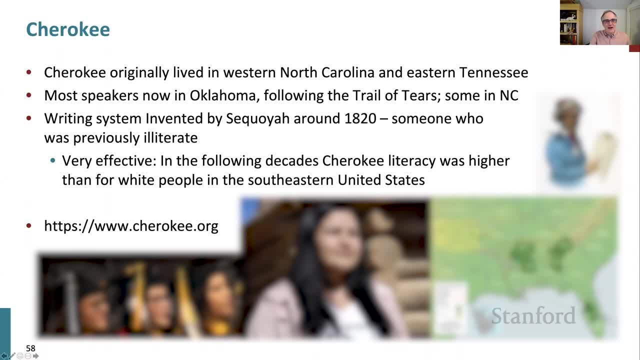 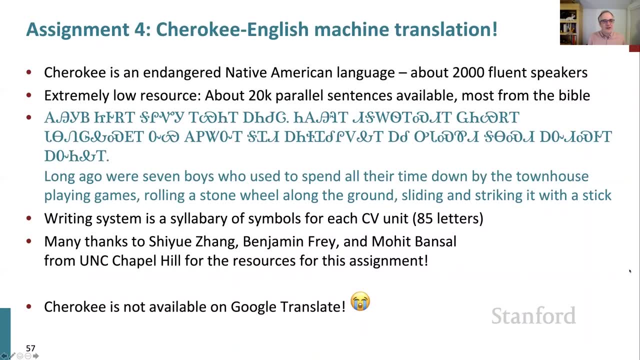 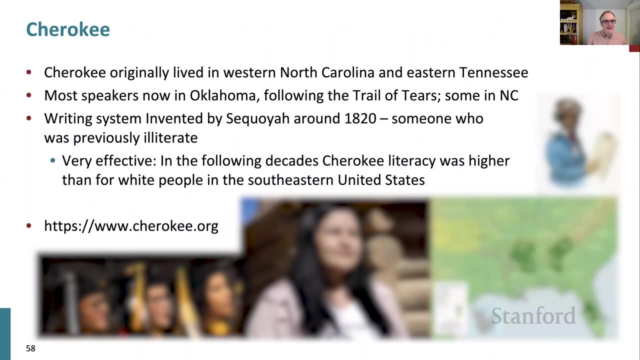 And so most Cherokee now live in Oklahoma, though there are some that are in North Carolina. The writing system that I showed on this previous slide. it was invented by a Cherokee man, Sequoyah. That's a drawing of him there, And that was actually a kind of incredible thing. 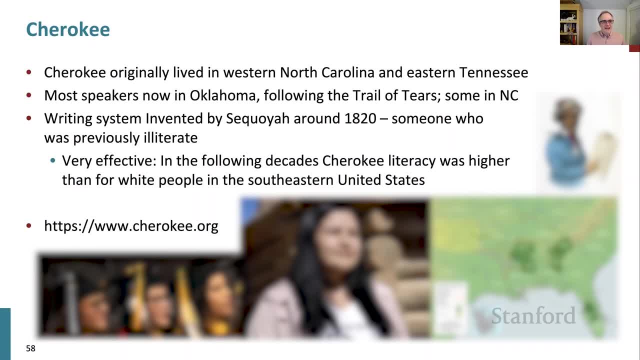 So he started off a literate and worked out how to write or produce a writing system that would be good for Cherokee, And, given that it has this consonant vowel structure, he chose a syllabary, which turned out to be a good choice. 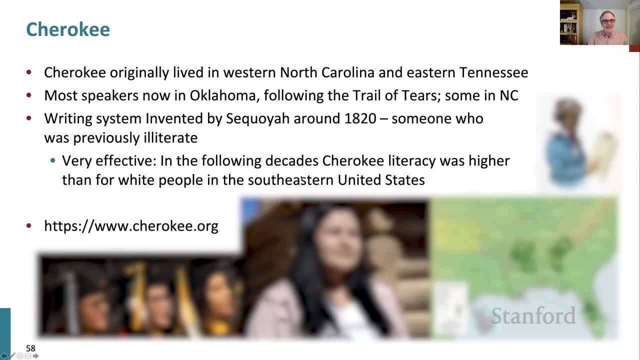 So here's a neat historical fact. So in the 1830s and 1840s the percentage of Cherokee that were literate in Cherokee written like this was actually higher than the percentage of white people in the southeastern United States at that point in time. 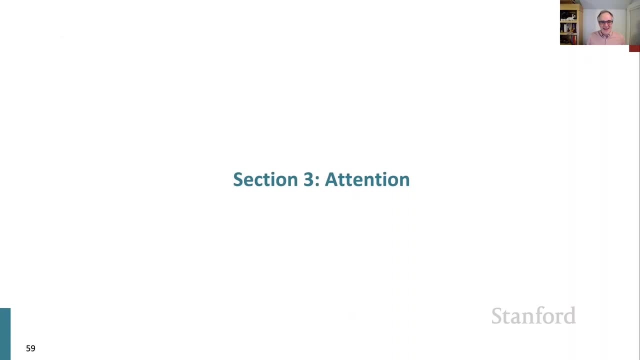 Okay, before time disappears- oops, time has almost disappeared- I'll just start to say: and then I'll have to do a bit more of this, I'll have to do a bit more of this next time. That'll be okay, right. 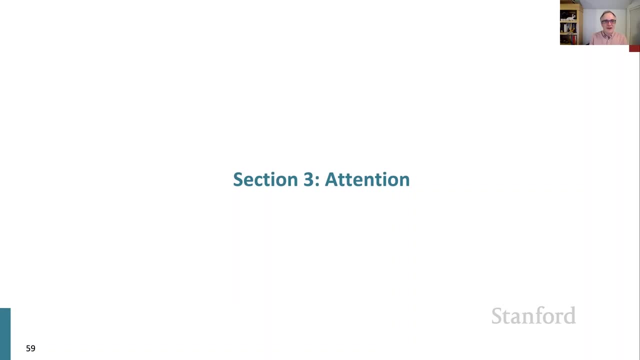 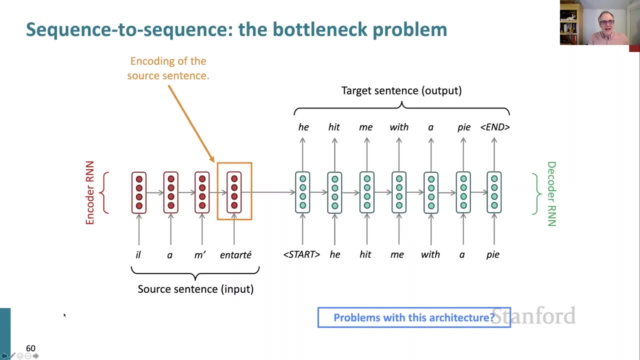 So the final idea that's really important for sequence-to-sequence models is the idea of attention, And so we had this model of doing sequence-to-sequence models, such as for neural machine translation, And the problem with this architecture is that we have this one hidden state. 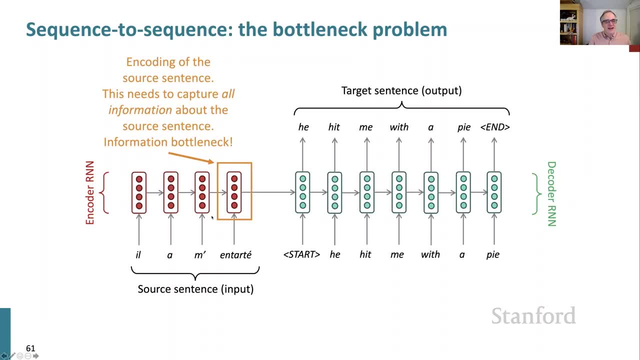 which has to encode all the information about the source sentence. So it acts as a kind of an information bottleneck, and that's all the information that the generation is conditioned on. Well, I did already mention one idea last time of how to get more information, where I said: 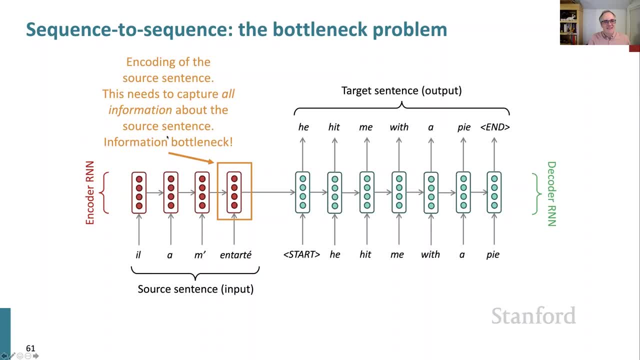 look, maybe you could kind of average all of the vectors of the source to get a sentence representation. But you know that method turns out to be better for things like sentiment analysis and not so good for machine translation, Where the order of words is very important to preserve. 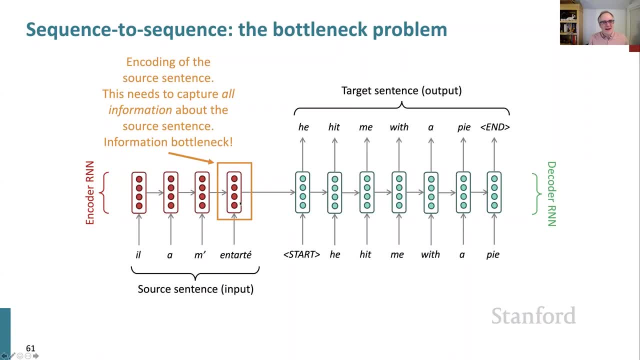 So it seems like we would do better if somehow we could get more information from the source sentence while we're generating the translation, And in some sense this just corresponds to what a human translator does. right, If you're a human translator, you read the sentence that you're meant to translate. 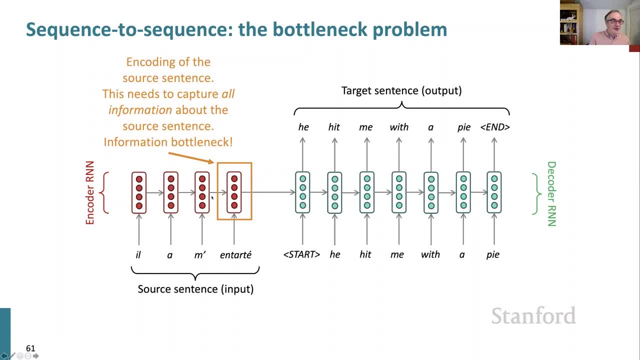 and you maybe start translating a few words, but then you look back at the source sentence to see what else was in it and translate some more words, So very quickly. after the first neural machine translation systems, people came up with the idea of maybe we could build a better neural MT model. 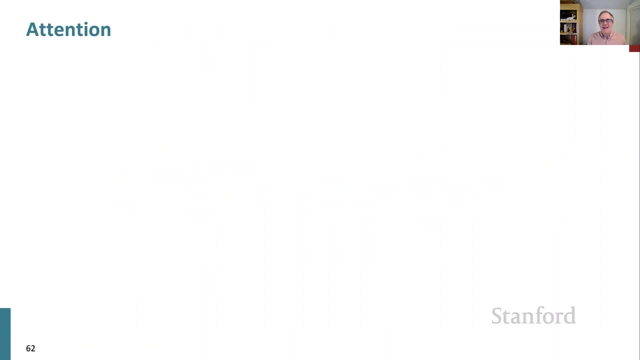 that did that And that's the idea of attention. So the core idea is: on each step of the decoder we're going to use a direct model and a direct link between the encoder and the decoder. that will allow us to focus on a particular word. 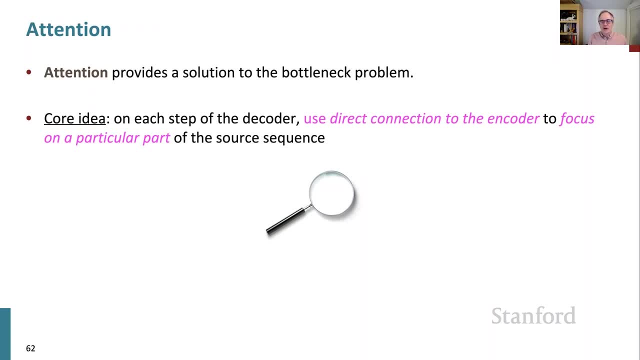 or words in the source sequence and use it to help us generate what words come next. I'll just go through now showing you the pictures of what attention does, And then, at the start of next time, we'll go through the equations in more detail. 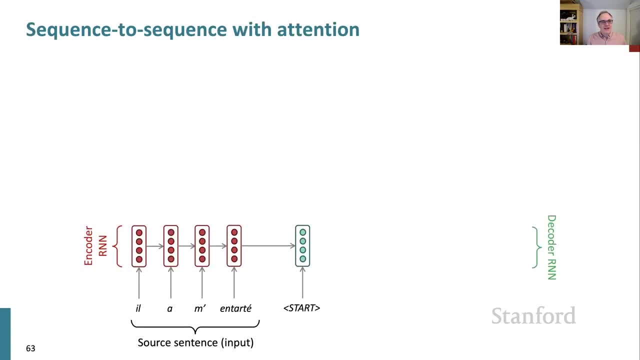 So we generate, we use our encoder just as before and generate our representations, feed in our conditioning as before and say we're starting our translation. But at this point we take this hidden representation and say I'm going to use this hidden representation. 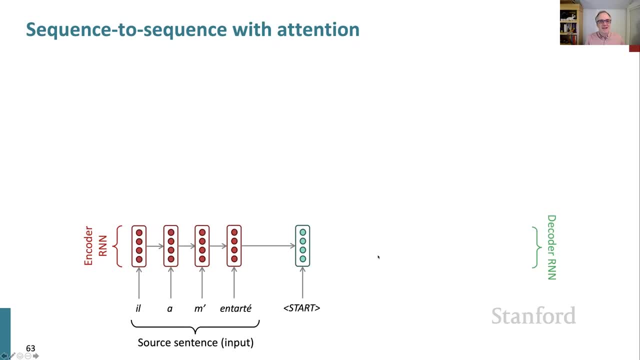 to look back at the source to get information directly from it. So what I will do is I will compare the hidden state of the decoder with the hidden state of the encoder at each position and generate an attention score, which is a kind of similarity score, like a dot product. 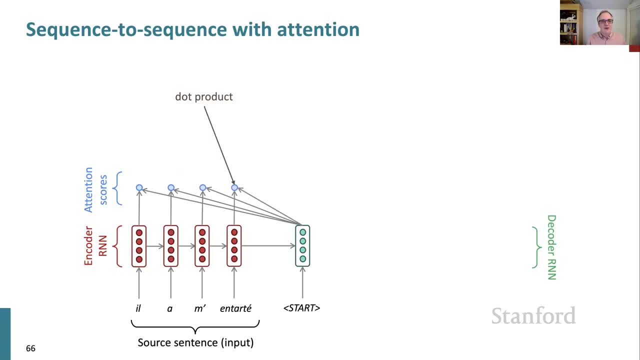 And then, based on those attention scores, I'm going to calculate a probability distribution as to, by using a softmax as usual, to say which of these encoder states is most like my decoder state. And so we'll be training the model here to be saying: 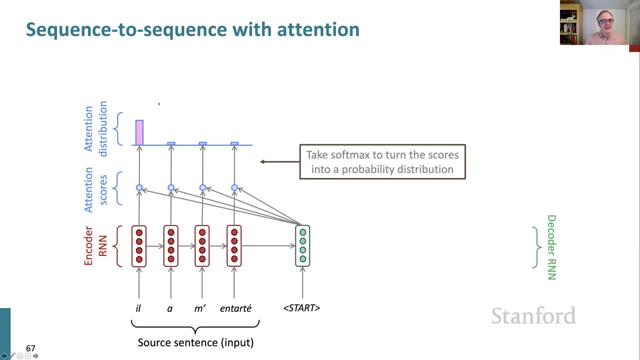 well, probably you should translate the first word of the sentence first, So that's where the attention should be placed. So then, based on this attention distribution, which is a probability distribution coming out of the softmax, we're going to generate a new attention output. 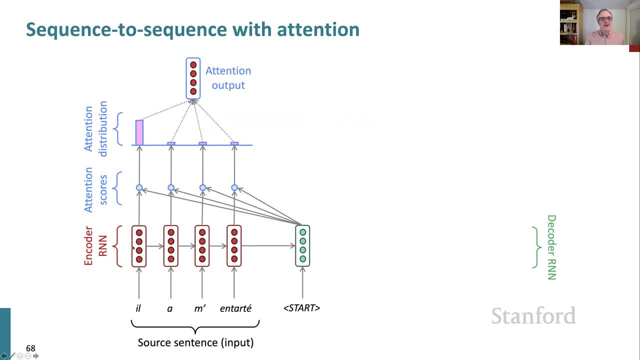 And so this attention output is going to be an average of the hidden states of the encoder model, but it's going to be a weighted average based on our attention distribution, And so we're then going to take that attention output, combine it with the hidden state.